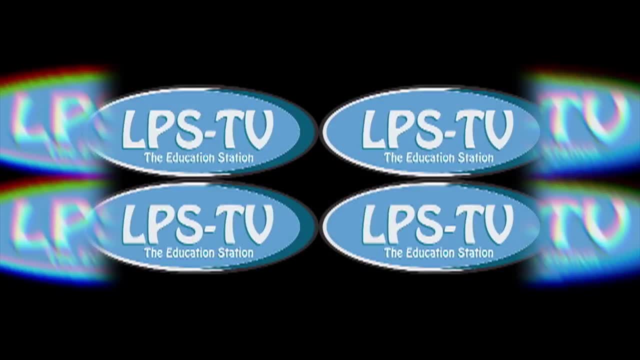 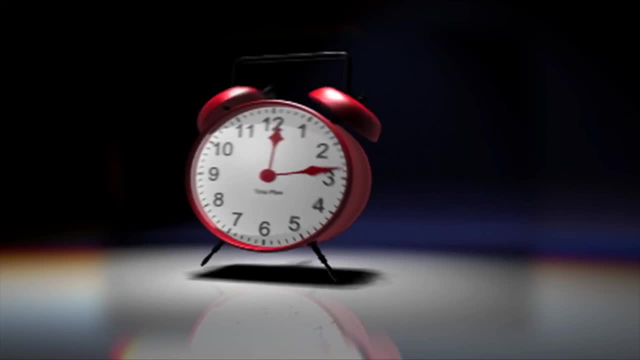 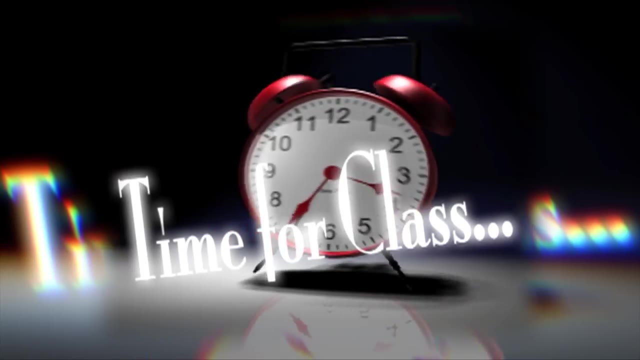 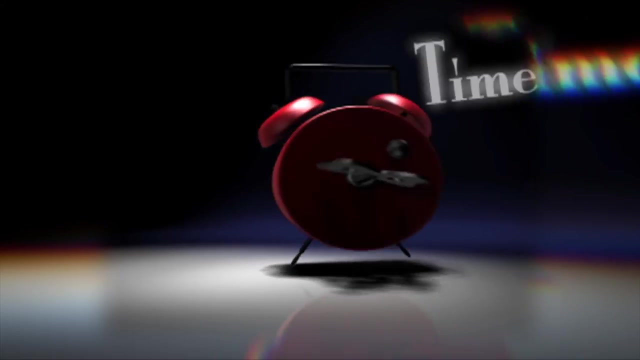 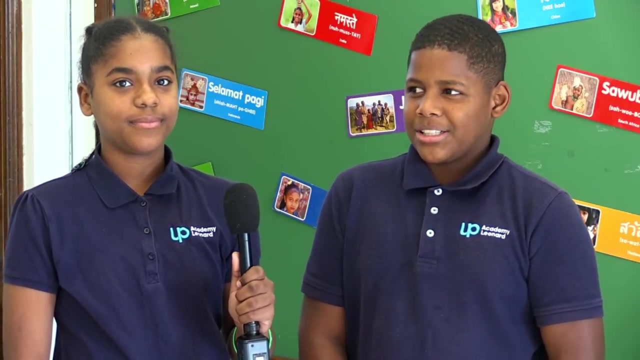 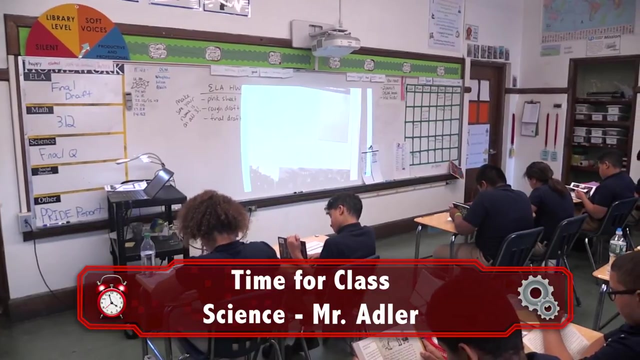 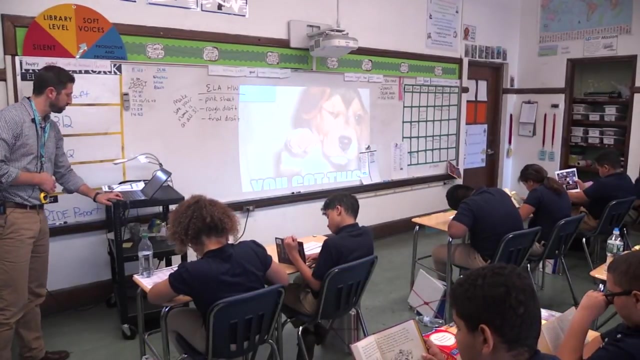 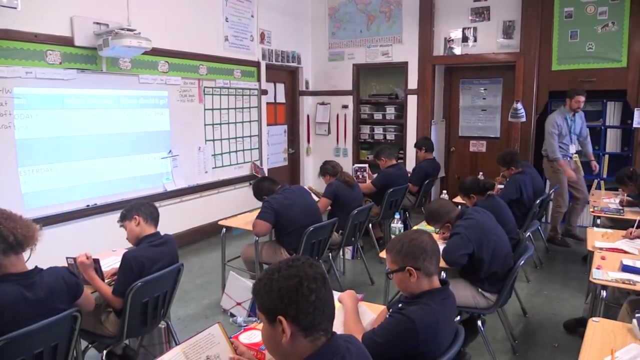 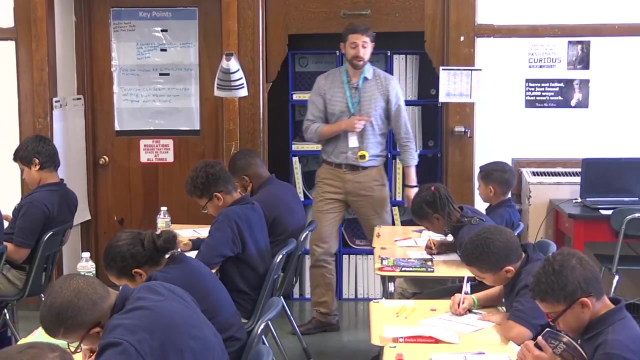 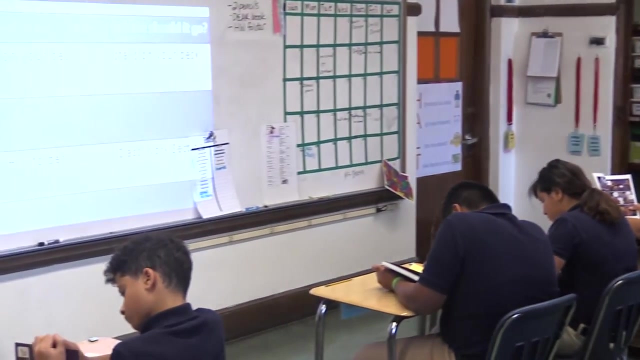 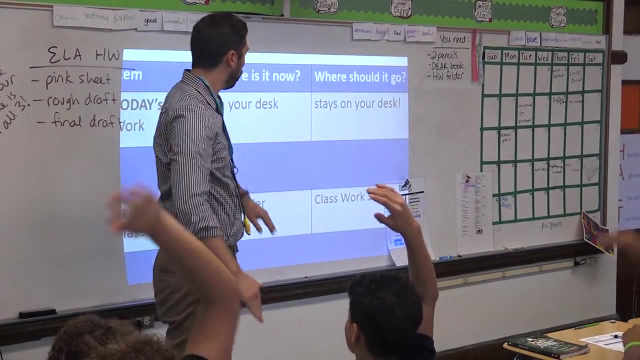 Welcome to the Op Academy Lennar. This is Mr Ellis, sixth grade science class. Final minute: Sienna, Make sure you have something written in the left column and in the middle column: Tres dos uno Hands down One minute. 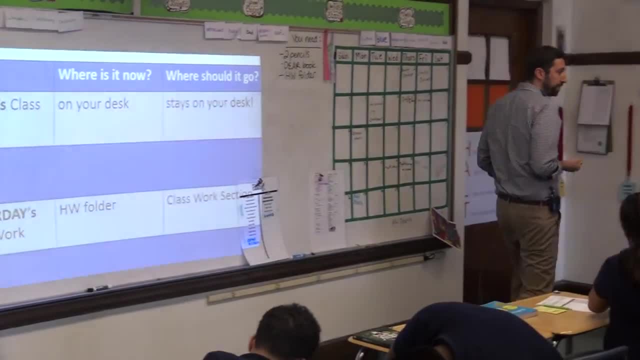 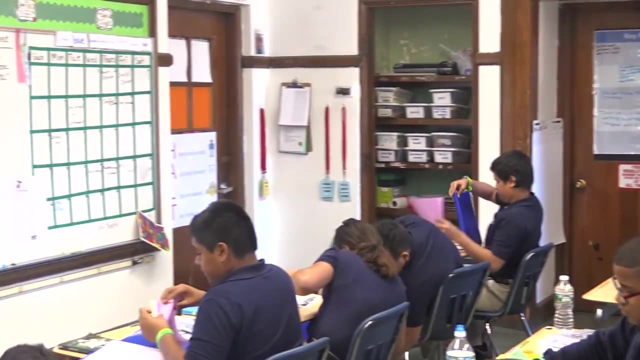 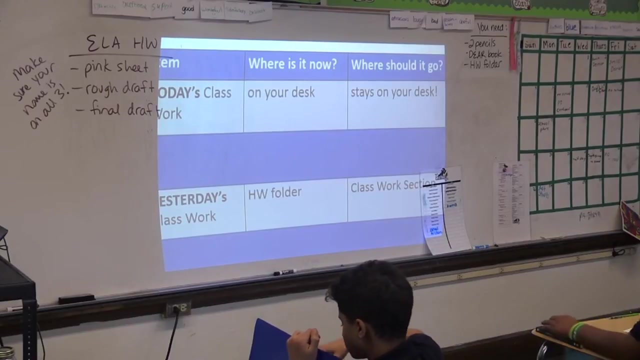 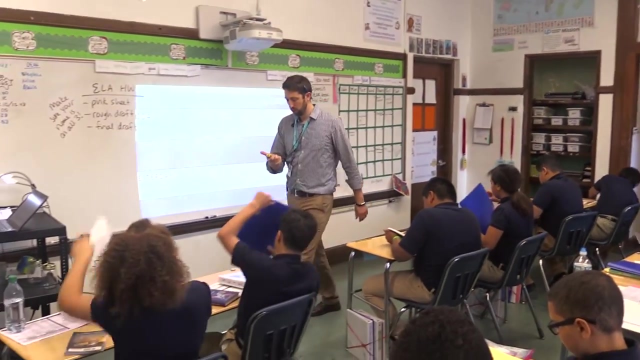 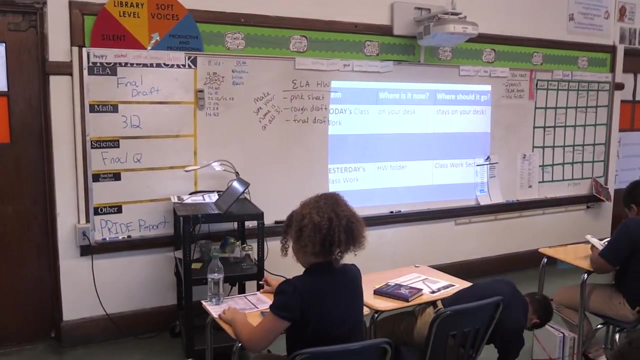 Sixty, fifty-nine, fifty-eight, fifty-seven Marital ladies, keep working on your. do now, or dear Fifty seconds, Nilsen's found, lesson twelve, Jose's getting organized, Merit Carlos, done and dearing Thirty seconds, Merit Nileshka. thank you for being responsible with that. 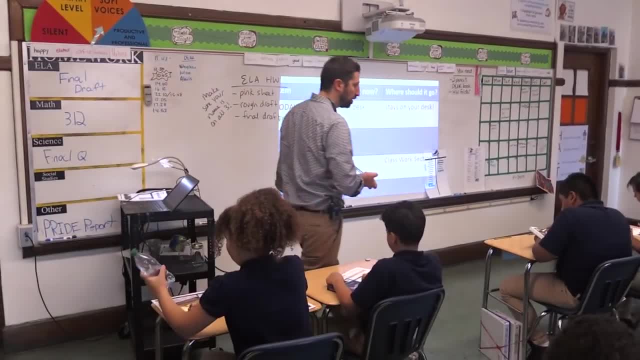 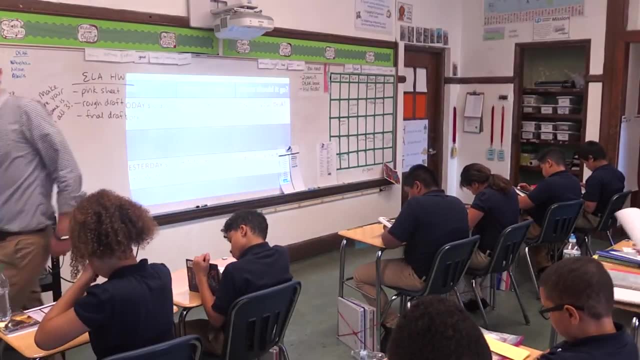 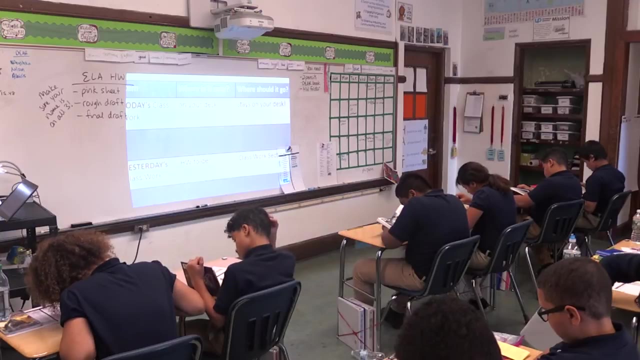 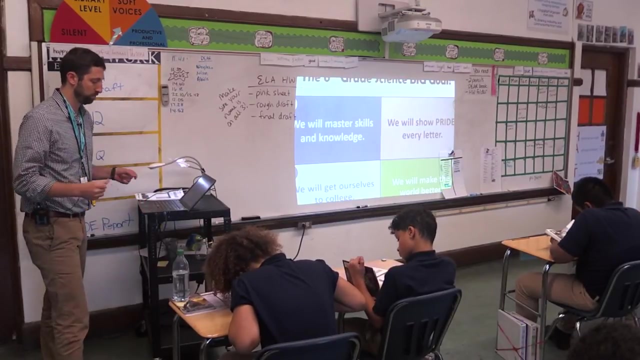 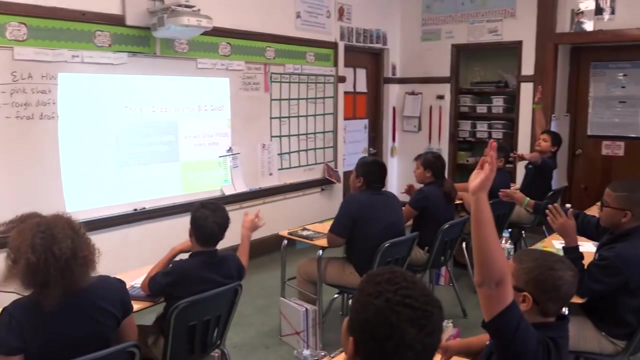 You've got twenty seconds. Anderson is done and dearing Omiel merit for remembering. You can go get it. I got it for you. Omiel, There you go. Who can read number one Anderson? We will match the skills in the army. 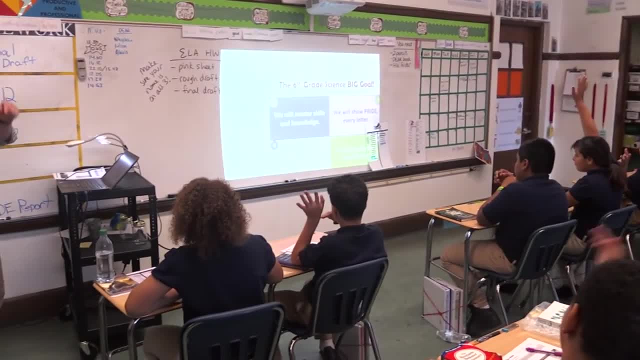 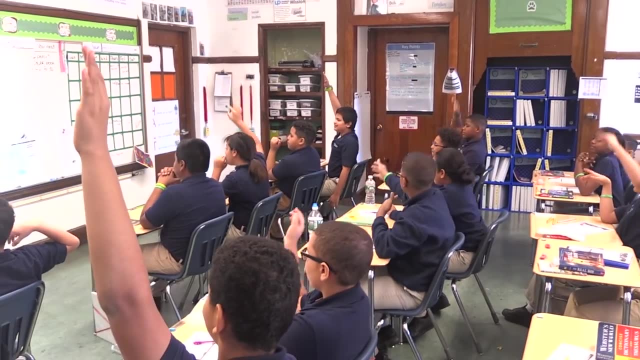 Power merit: Nileshka. We will get ourselves to college. Power merit: Darwin: We will show pride in the betterment. Wilbur for the class. We will make the world better. Sienna, snap it up for starting with our power merits. 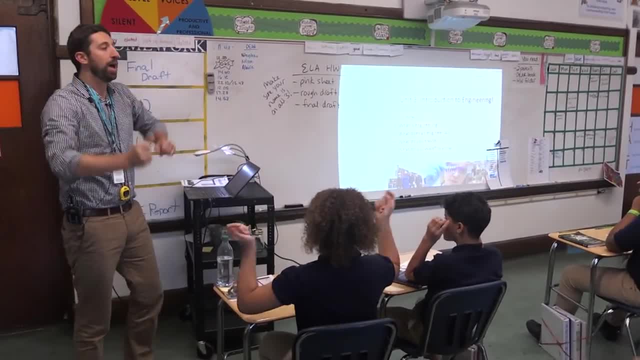 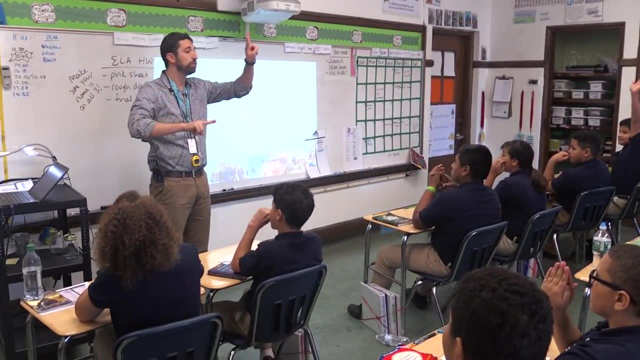 Welcome to unit three on engineering. I know we've been. this is actually day one and I don't know what you know from fifth grade, So I just want two answers from the first box and two from the second box. What do you know about engineering? 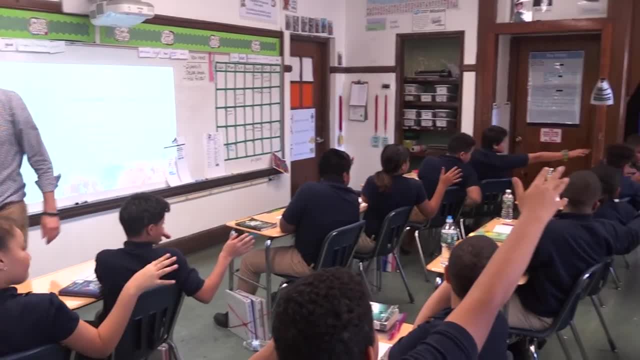 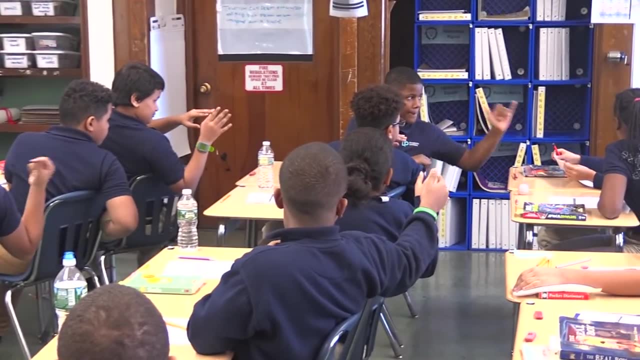 Hands down. track Jose, Mateo and Shine. I know that they know stuff, or sometimes they don't know what they want to do. Merit Jose for the agreement signal and merit Jose for the good start. track Edgar: what do you know? 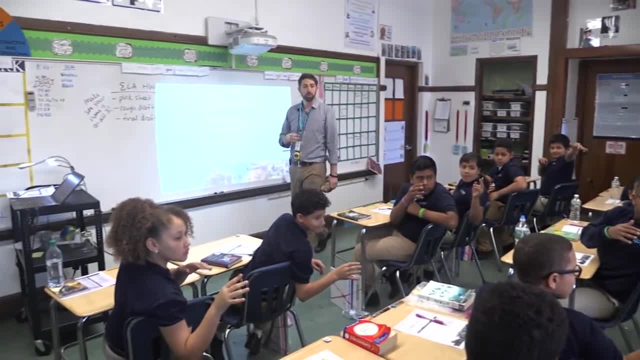 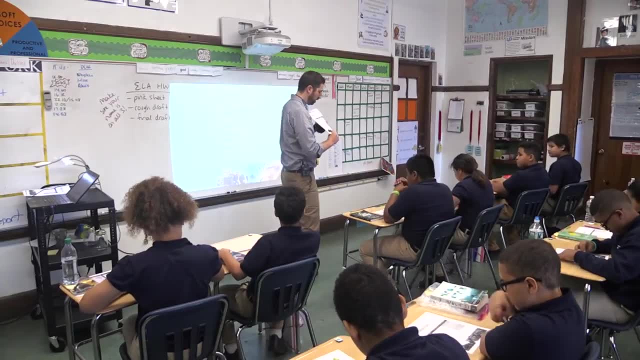 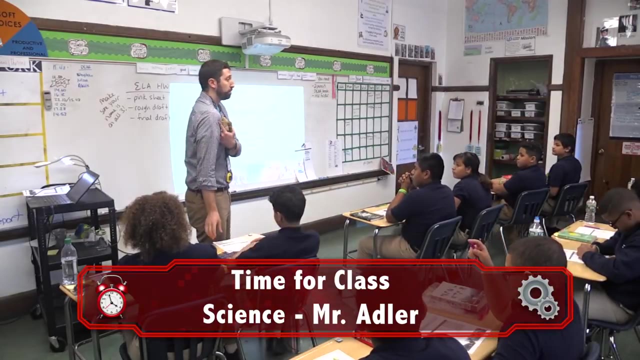 I know that engineering is like the kind of motor for Ooh, but you have to be careful, Hands down if you track the middle picture or me. sometimes people think it's just motors. Engineers might also design medicines. Engineers might also design replacement limbs for people who lose them during wars. 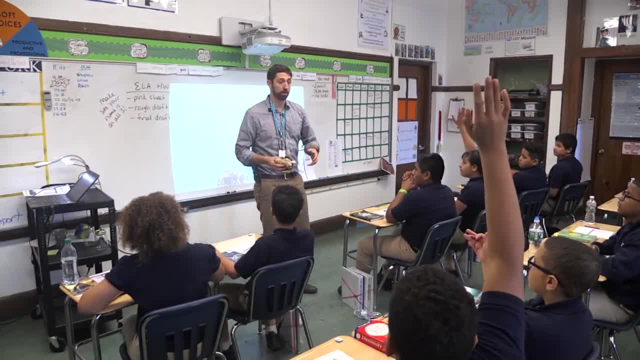 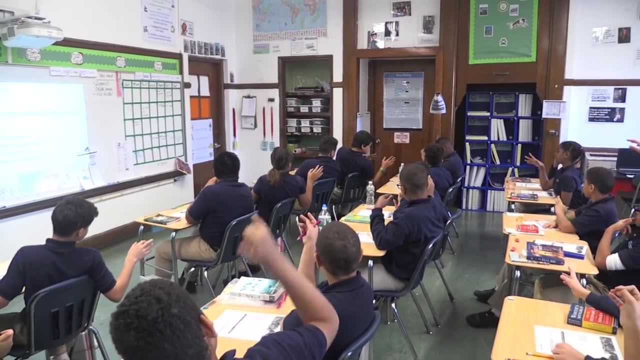 Engineers don't just make machines. What do you want to know about engineering? What do you want to know? Hands down track, Jose Francis Shining. I want to know how they Power. I want to know how they- And you won't get that- this unit. but we'll talk about that later this year. 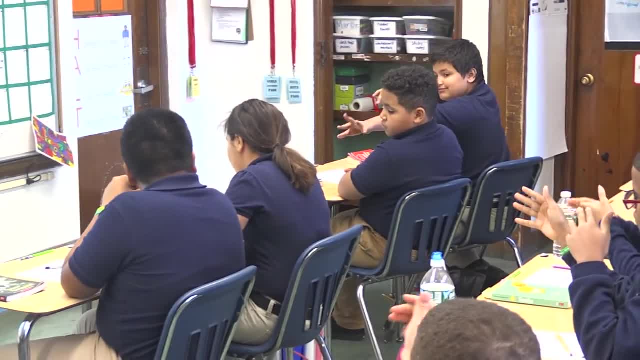 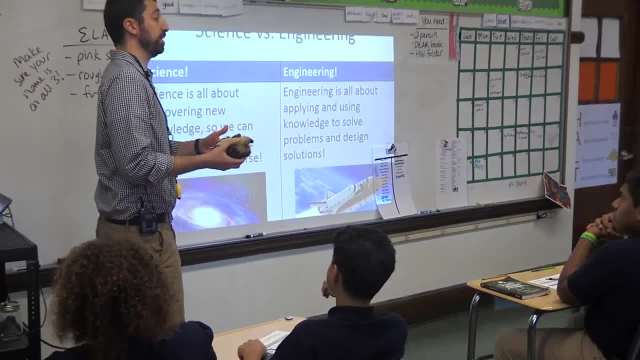 And hands down track. Jaylen, what do you want to know? I want to know if engineers build things. They almost always build things. Sometimes, though, they might design things. They might not be building things every day Tracking up here. 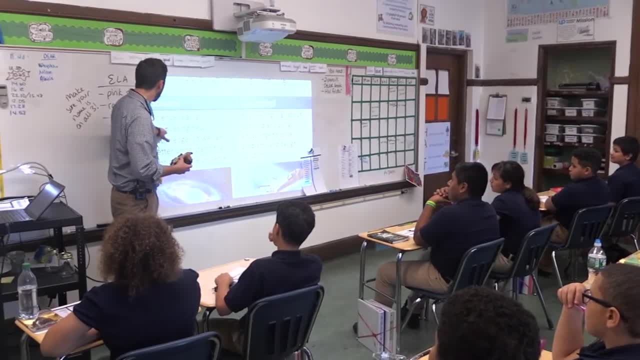 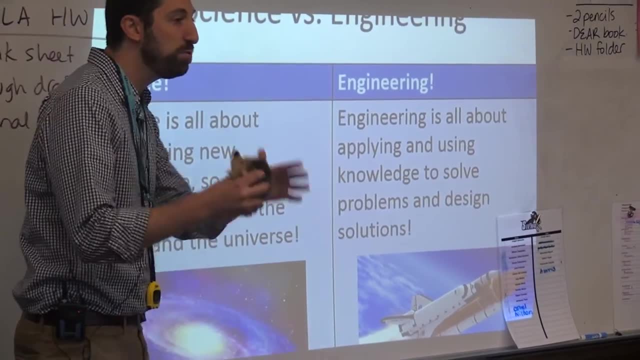 So far this year, we've just been talking about science. Science is all about discovering new knowledge, so we understand the universe. Scientists might go out and they might say: oh man, I just discovered this new galaxy super far away. Juan Luis de Mir, get your hand down. 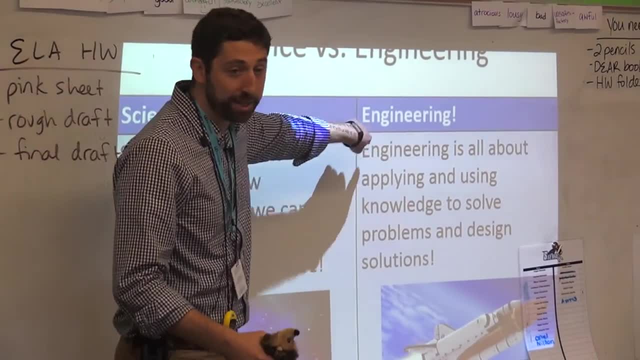 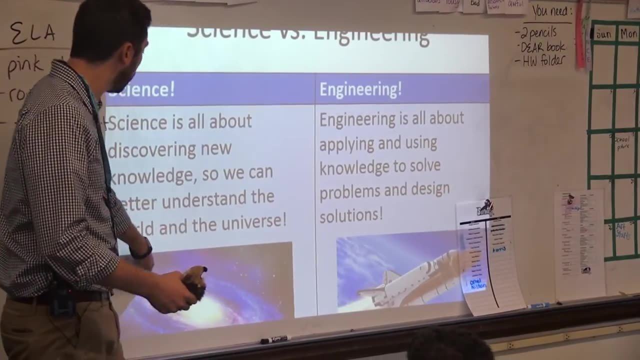 They might say, oh man, I just discovered how particles work. But engineering is all about using the knowledge to design solutions and solve problems. So if scientists say, oh man, here's the galaxy, engineers would say, sweet, how do we solve the problem of? 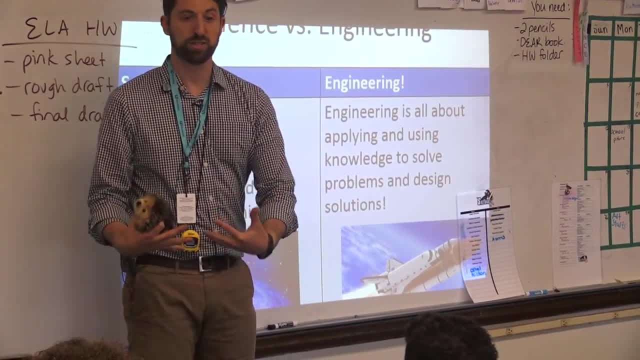 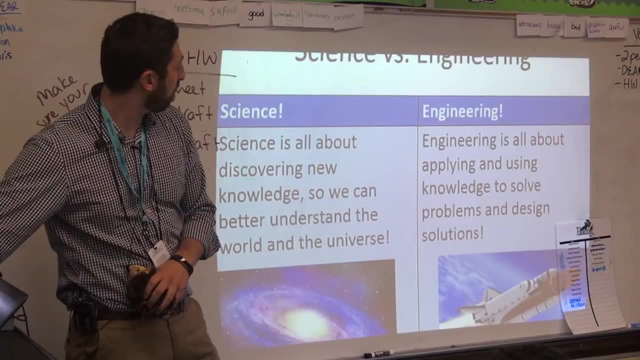 I need to discover it and it's really far away. I have to invent a space shuttle. Engineers are using the knowledge scientists find to design solutions to problems. So here is your first problem you need to solve during this unit With power: Frandi. 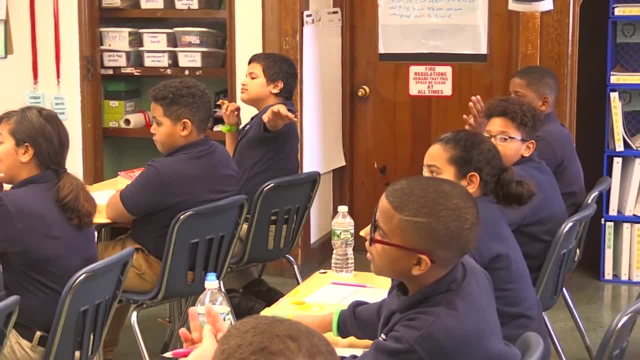 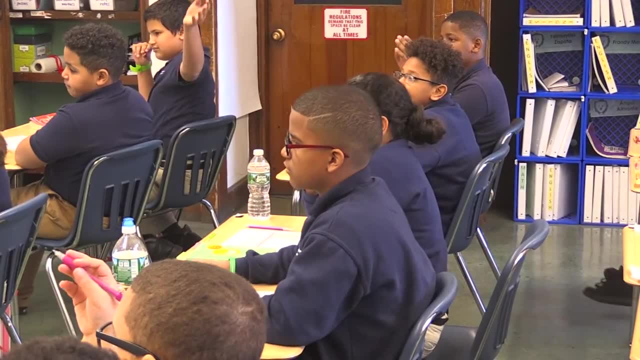 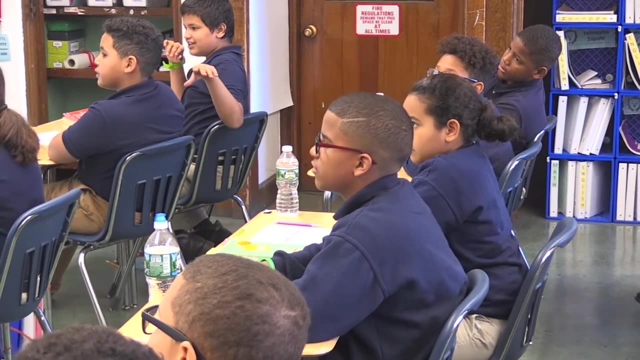 Engineers will be able to build an index card for Yep. Repeat after me: Frandi Tower, Gland. Wave the ball. Repeat after me: hedgehog, Hedgehog, Hedgehog, Hedgehog. Track me. This is Glenn the hedgehog. 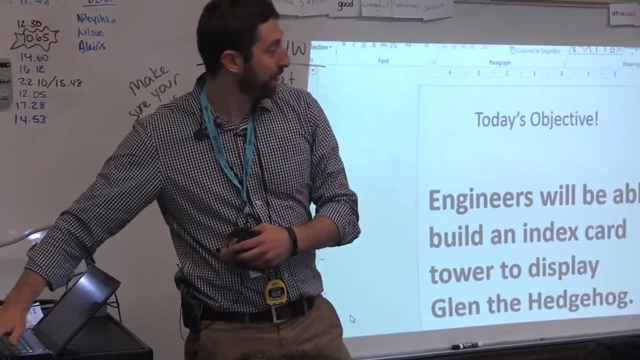 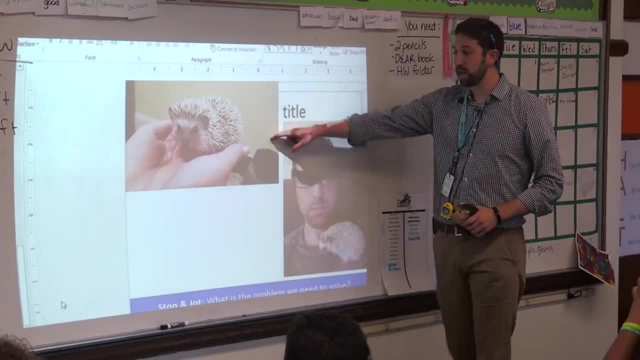 Everyone say hi Glenn, Hi Glenn. So you guys might not know this, but I actually I don't have a dog and I don't have a cat. I have a hedgehog. This is my hedgehog. Her name is Eleanor and she is the best hedgehog ever. 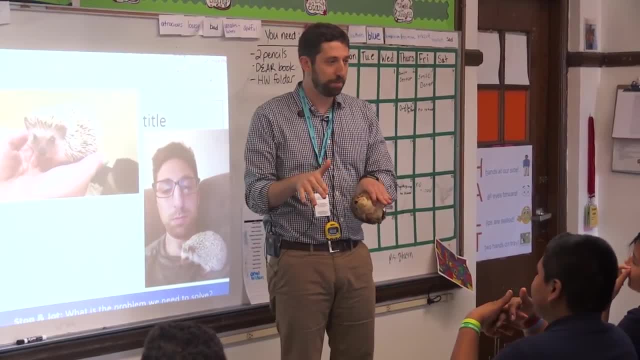 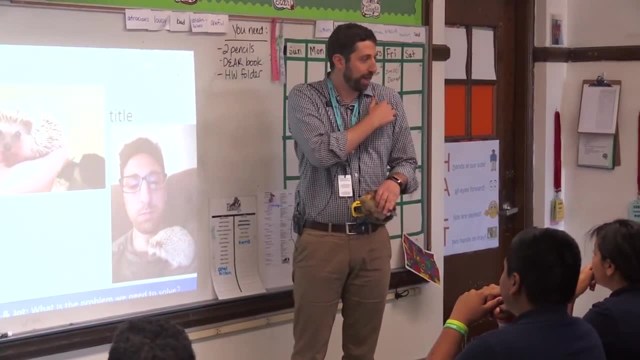 Snap it up for Eleanor the hedgehog. This is not a joke. This is legitimately my hedgehog And because someone didn't believe me, I took a picture last night with Eleanor on my shoulder. she really likes to crawl and like hide, but she 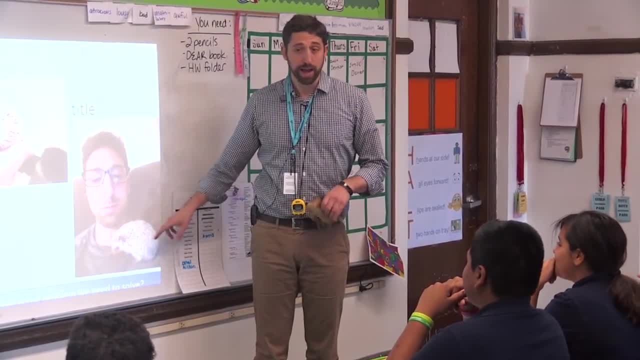 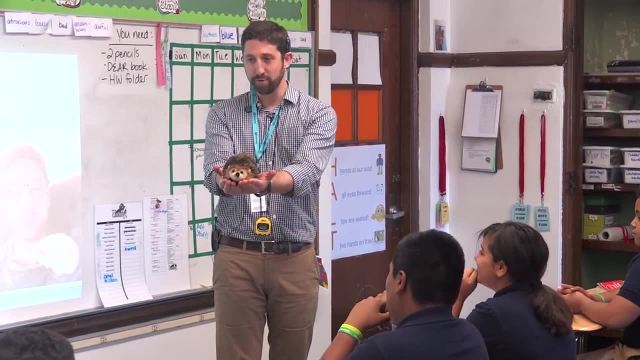 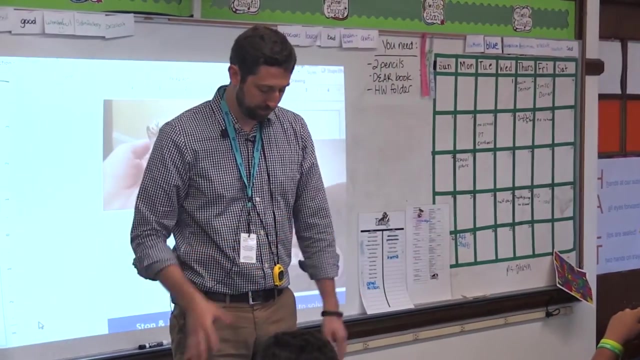 couldn't find a place to hide, so I took a good picture. this is Eleanor, and Eleanor is very important. this is Glen, who is her slightly less alive cousin. this is a hedgehog. everyone say hi, hedgehogs. hedgehogs are great. they're normally really spiky, but this one is not. now, here's the problem: hedgehogs are. 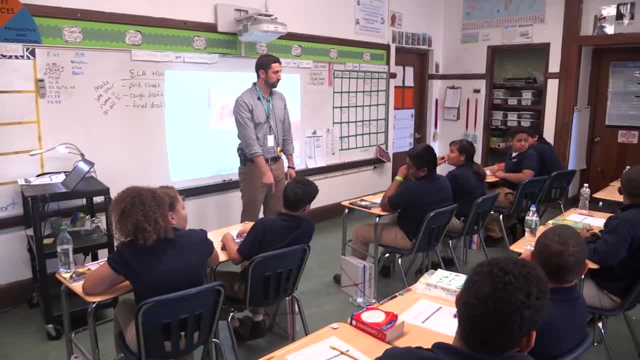 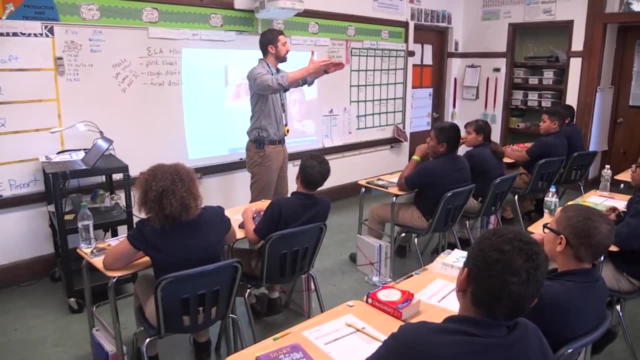 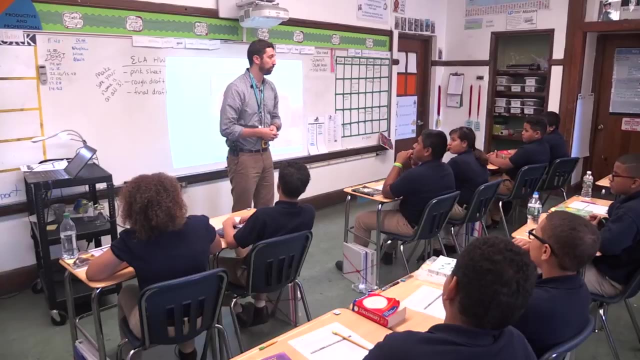 important ladies. can you see Glen the Hedgehog? no, not really. I want to make hands down a tower tall enough that I can see Glen the Hedgehog. because the problem is, I want to see Glen. Glen is really important to me, but I can't see Glen. Glen is on the floor. who can tell me what's the problem? I need to solve? 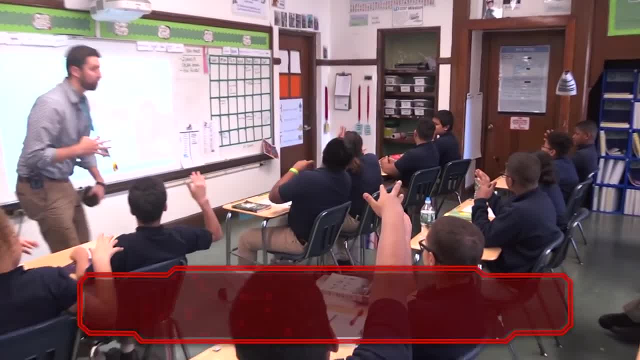 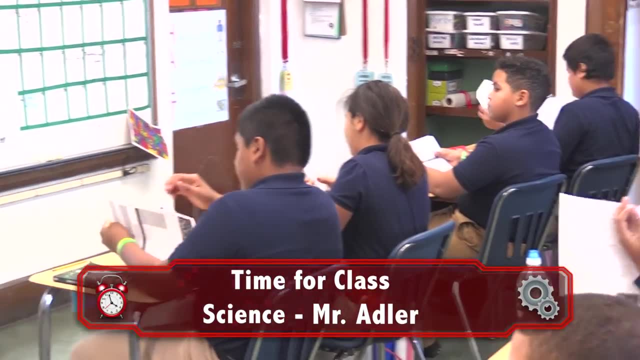 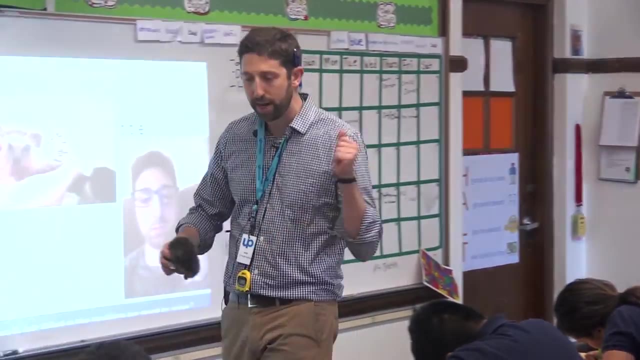 today. hands down, track Wilbur and shine. turn the page at the top of page two, stop and jot. you have one minute. what is the problem we need to solve today? what is the problem I need to solve today? Merritt Edgar started right away. Juan Lewis is writing a. ladies is writing. what is the problem I? 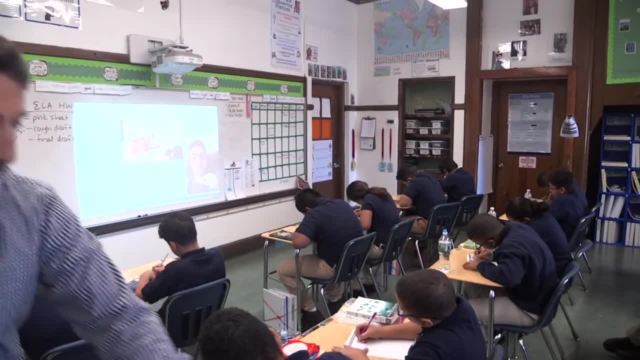 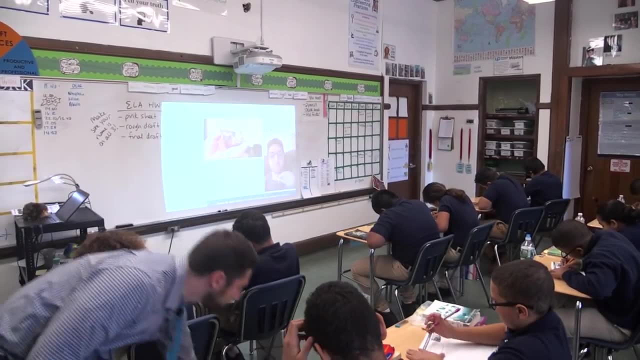 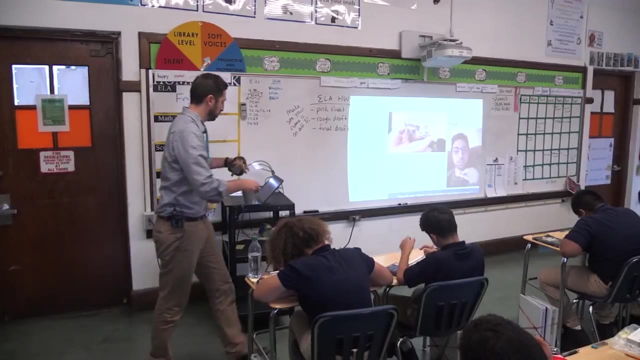 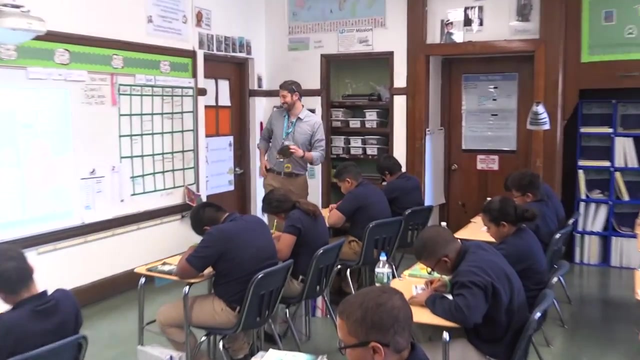 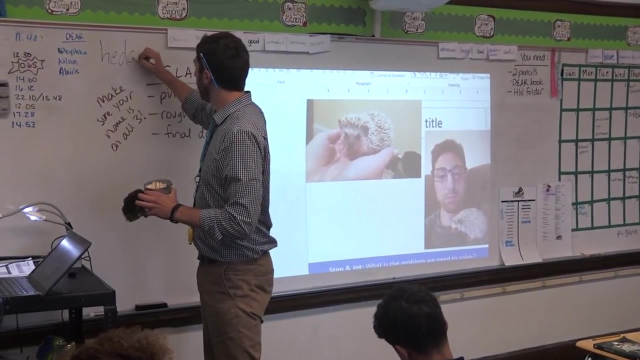 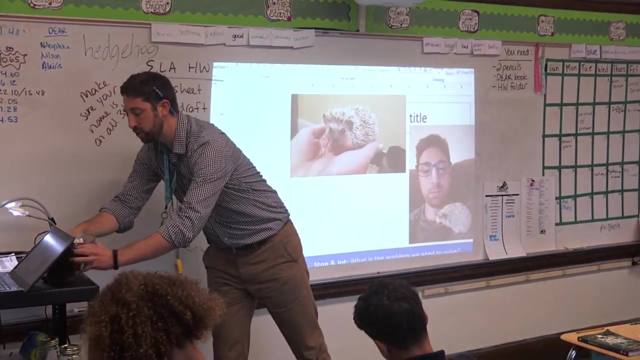 need to solve today. top of page two. what is the problem we need to solve? Angel's writing. Nileshka's writing smart hand. Merritt to Carlos. you write hedgehog. in case you're looking for some spelling help: HED GE HOG. when you were done, show me a thumb. you have 30 seconds. 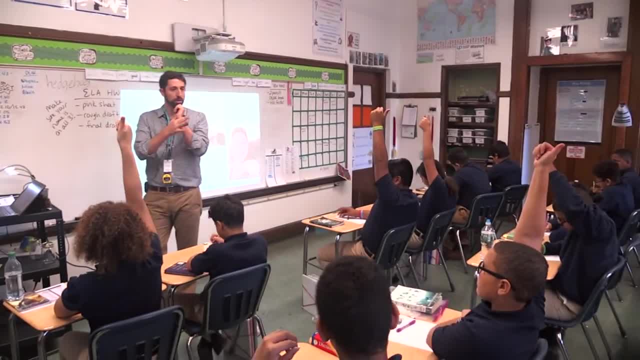 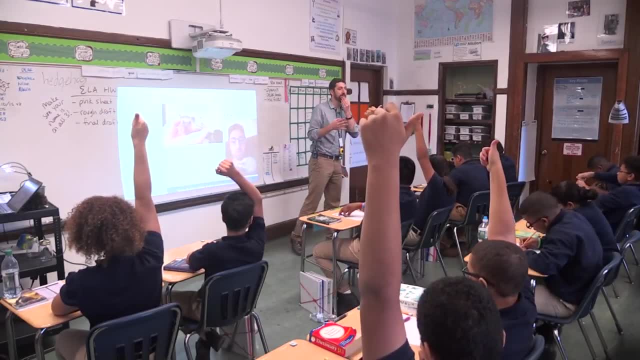 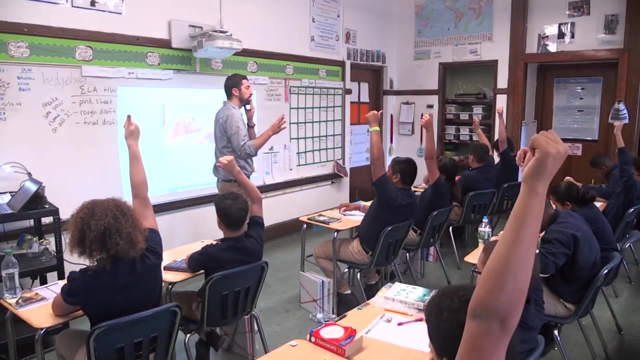 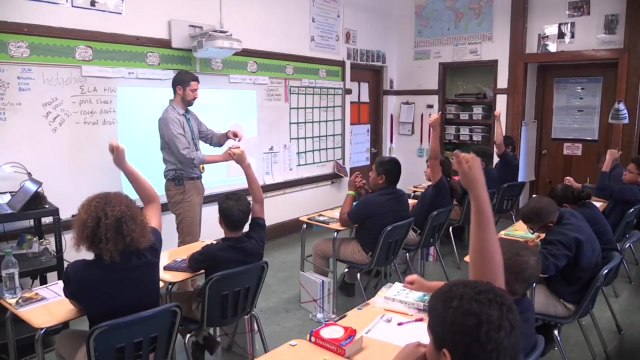 a lady's posture: Merritt. Edgar looks ready, Oscar looks ready. not that one yet. 15, 14, 13. angel looks ready. angel to Merrick, get your arm off your chair. seven, six, five, four, three, two thumbs down right or track Anderson. Anderson, what's the problem? I need to. 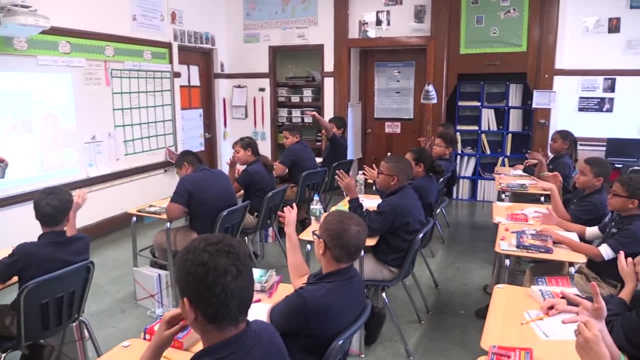 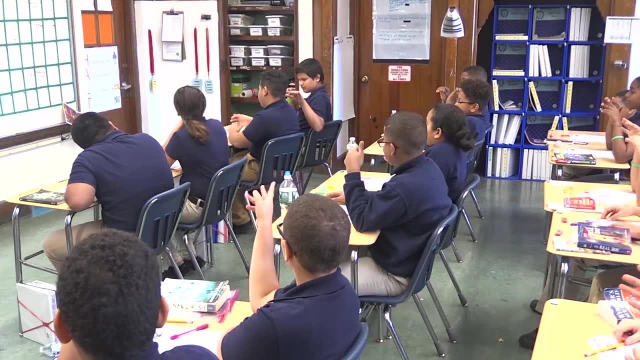 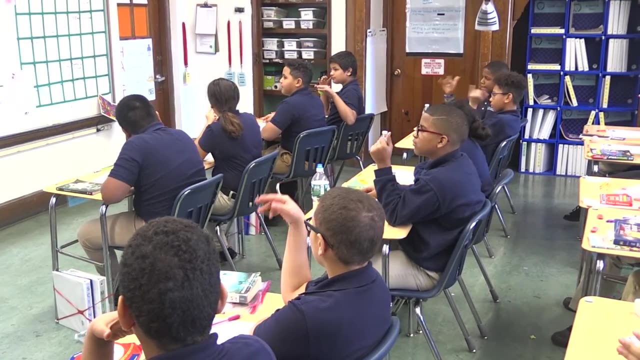 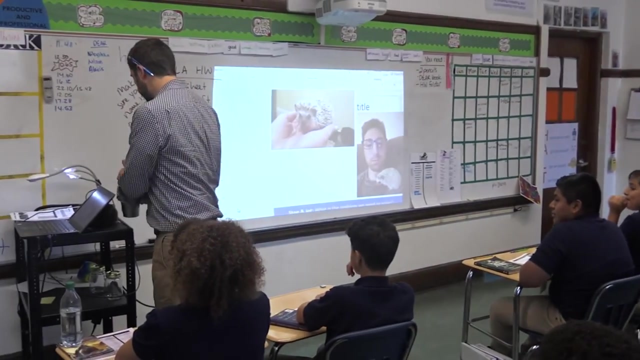 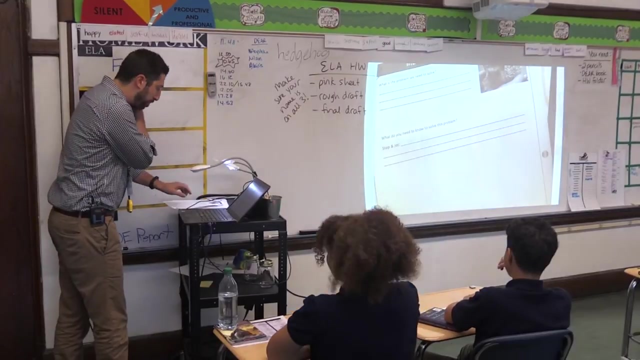 solve today. make a tower to see Glen the Hedgehog. who can tell me what Anderson said, Carlos or what you thought? and again, Hedgehog's name today is Glenn. this is Glenn. everyone say again: hi Glenn. but the problem is you don't really know how you're doing this. and on page two, right. 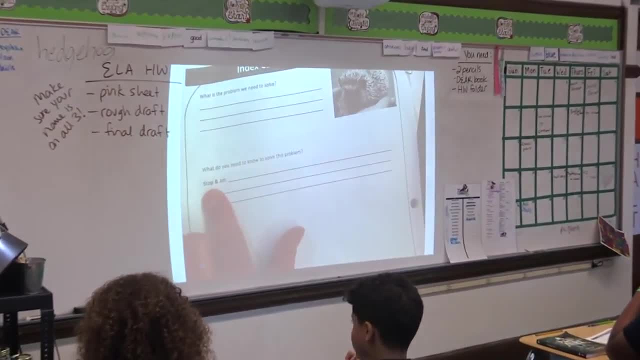 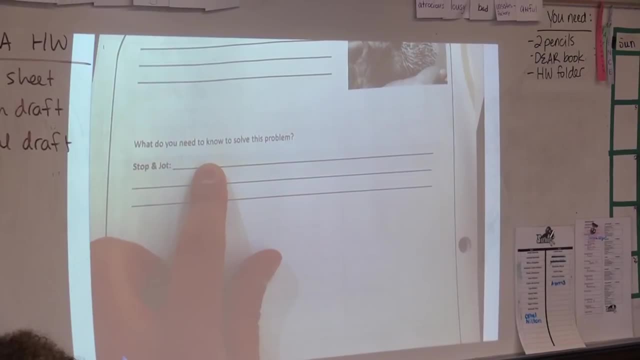 below, where you just wrote the problem. I want you to brainstorm storm. what do you think you need to know to solve this problem? Second, stop and jot. what do you think you need to know? What questions do you have for me? What do you need to know to solve this problem? Think about it and try to write. 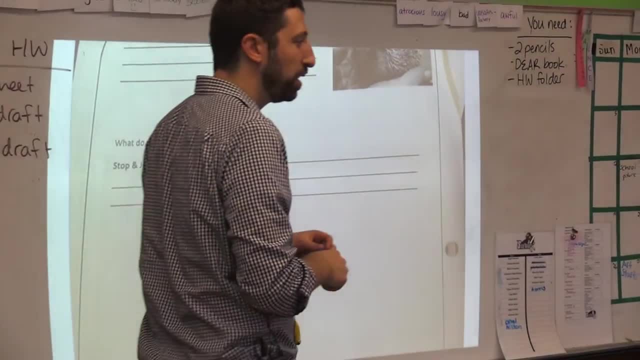 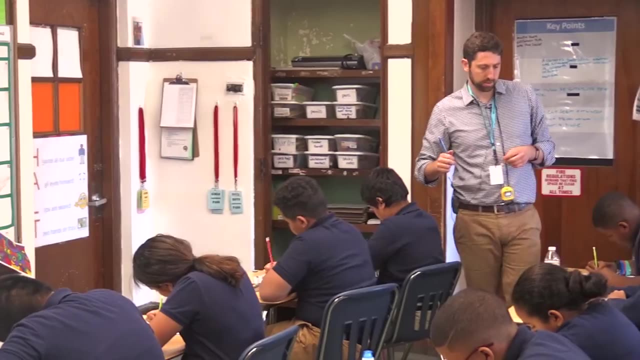 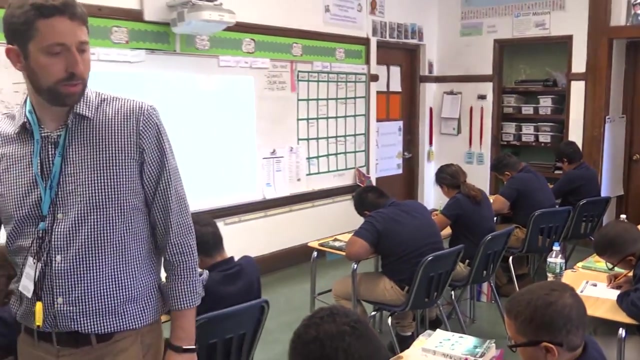 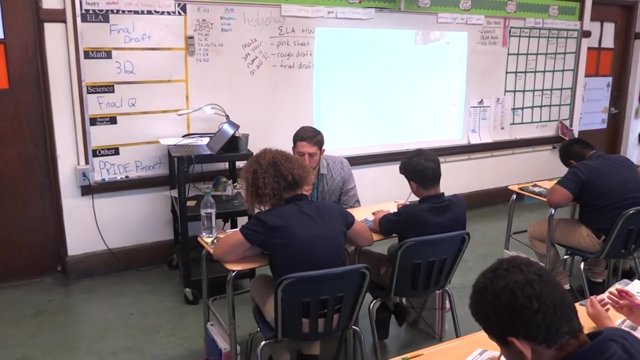 at least one question you have for me in the next minute. What do you need to know? Jose has an idea. Darwin is writing. Angel is writing. What do you need to know from me? Elysa has a great question for me. 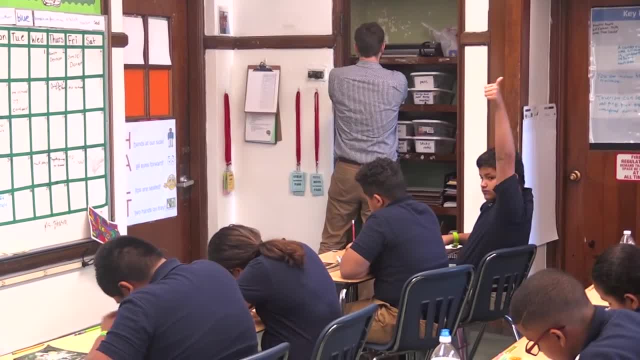 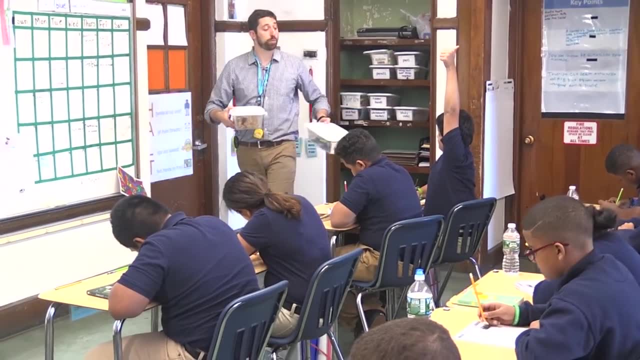 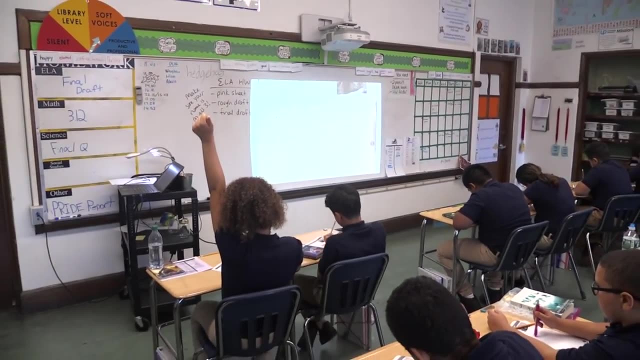 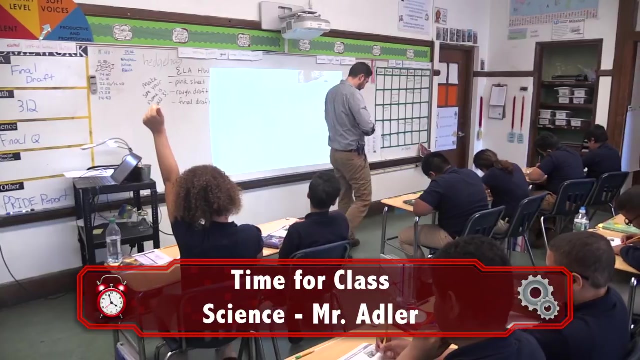 You've got 30 seconds, If you think your, If you're done early, see if you can come up with another question. Ten seconds: Milos has got a question. Antoine's got his question. see if you can think of one more. 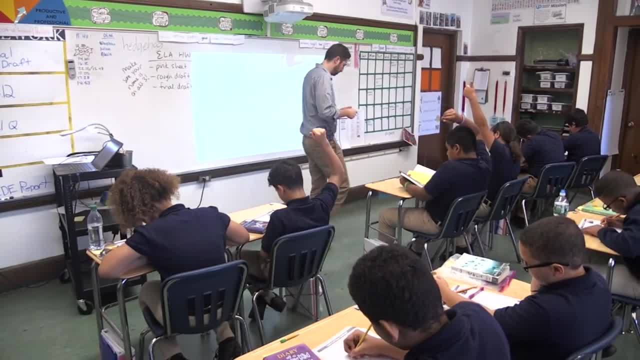 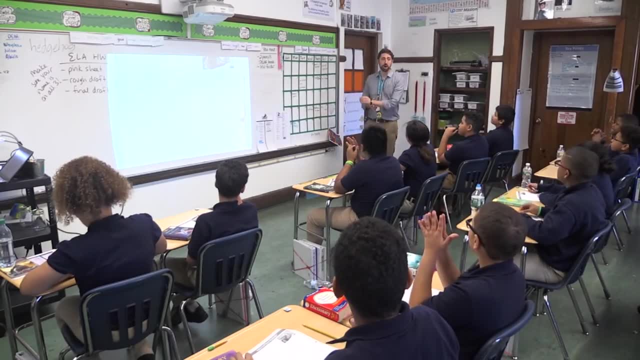 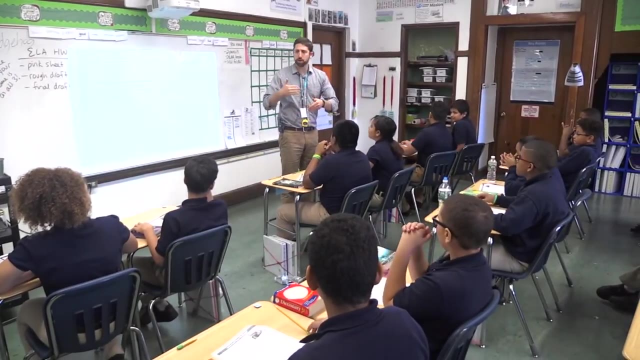 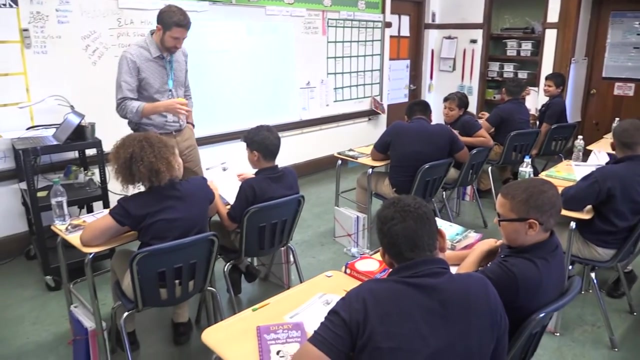 since you're done, early Rally Robin Back and forth. A then B. A share your question, B share your question, And if your partner gives you something you didn't think of, write that down too. You have one minute. I said: how's the toilet? 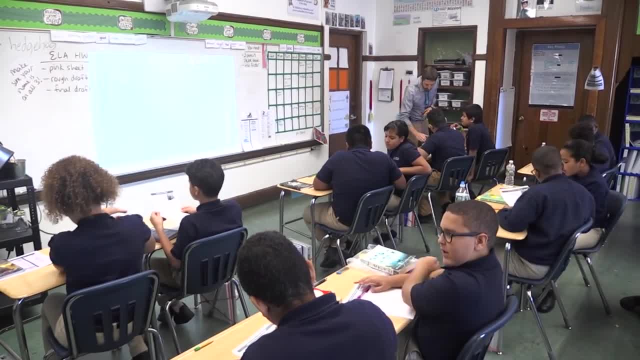 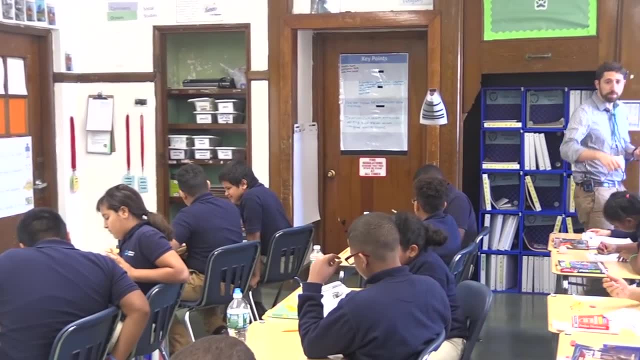 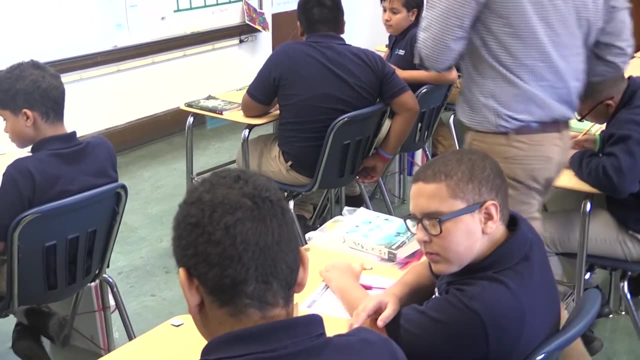 I said: how's the toilet? When I see the paper between you you're leaning in. that's what respect looks like. Merit Merit Alades adding to her answer. Merit Nileshka adding to her answer. 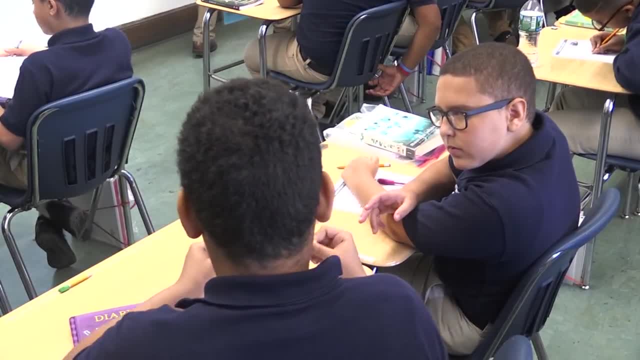 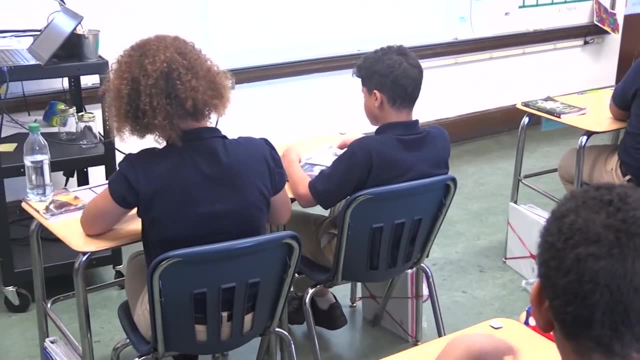 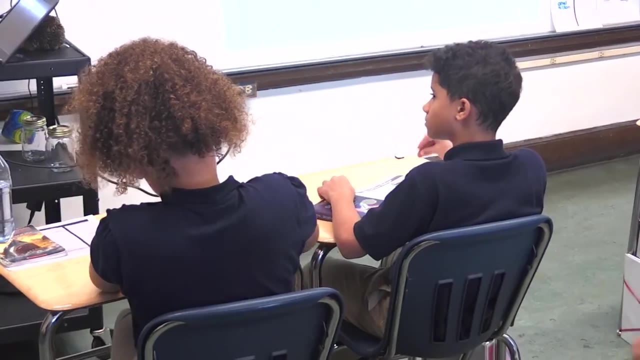 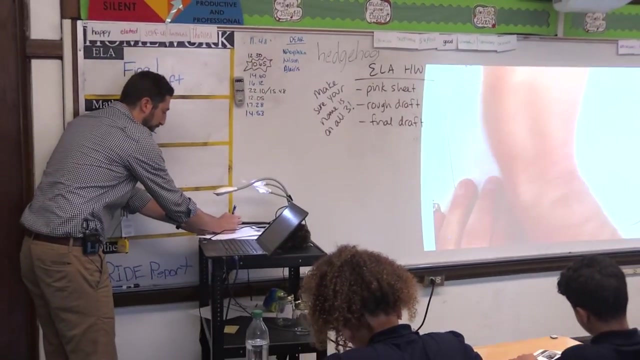 Merit Giamaitis, Merit Frandi Jose. did she give you anything you didn't have? You wrote it down. Okay, Write or track me Below the stop and jot. I want you to write a T chart. 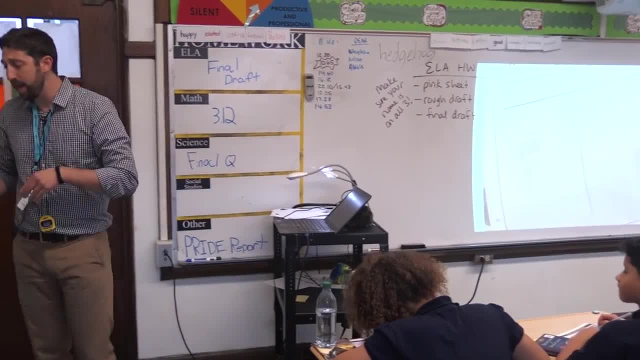 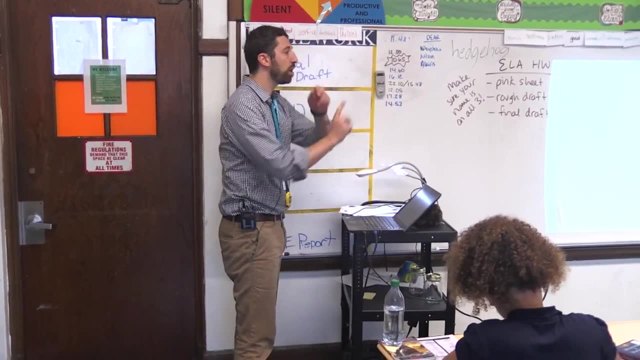 And we're going to write down not the questions you ask me, but the answers. If it's important, I need to tell you Who has a question for me about what you need to know today. Track Carlos or write The weather. 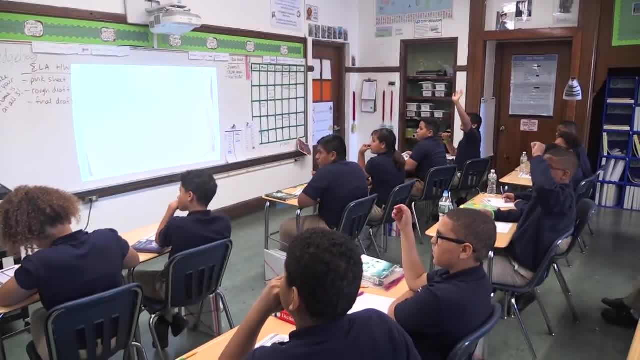 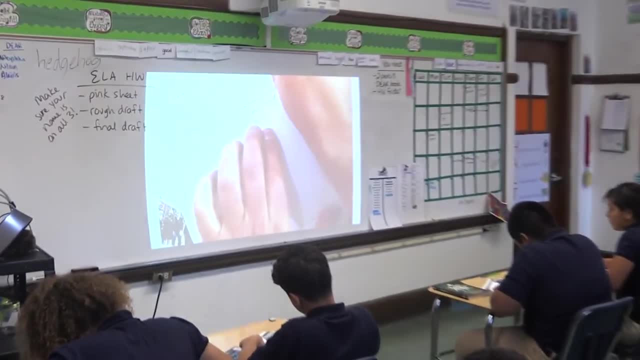 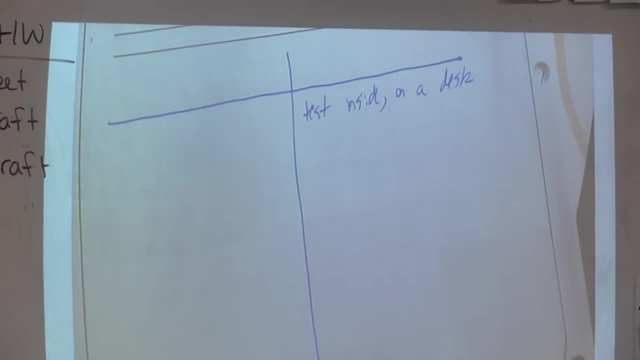 The weather. Good question, We are building it inside. You must test inside. So I'm going to answer Carlos' question: test inside on a desk. Good question. Make sure you write down the answer to Carlos' question. Darwin. what do you need to know today? 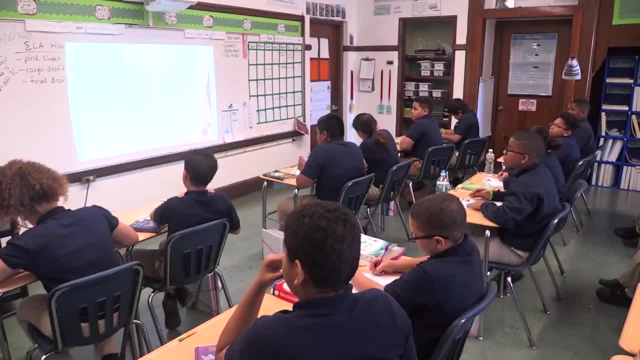 I need to know how to stack cards. Ah, do you know you've got cards? What? How do you know you've got cards? Is it on the top? Is it in there? Is it on the top? Is it in there? 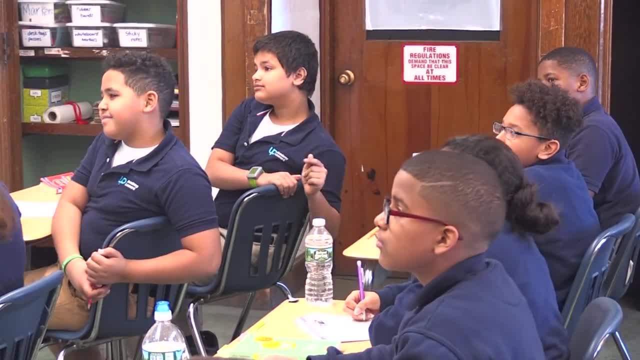 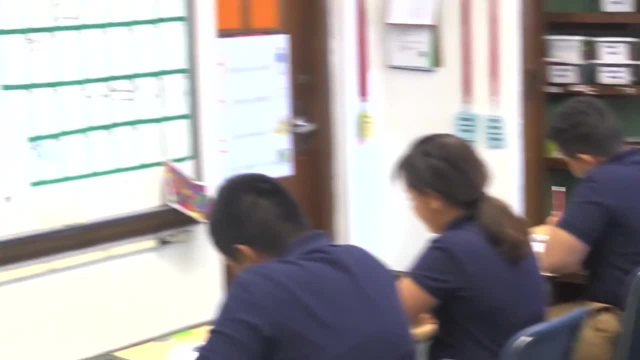 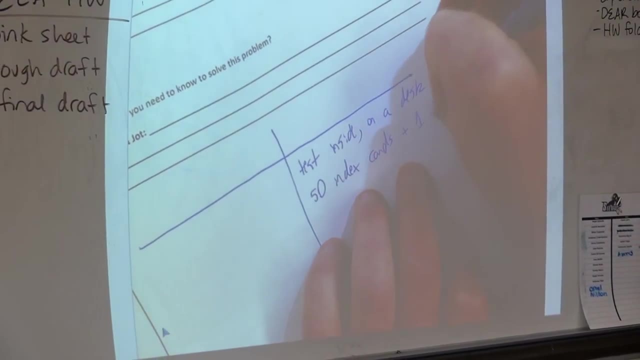 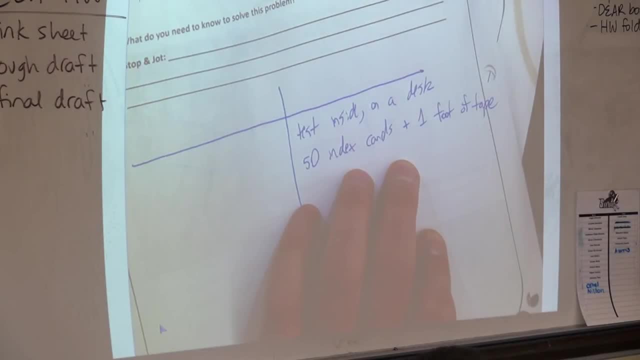 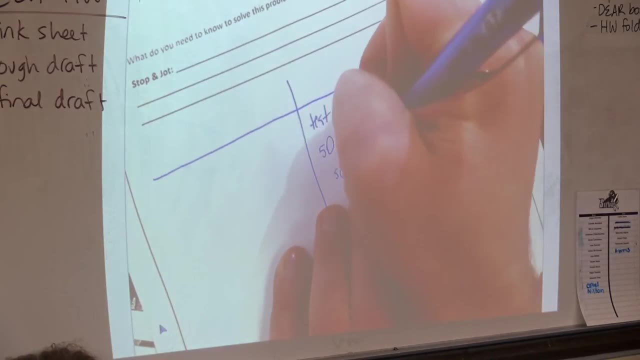 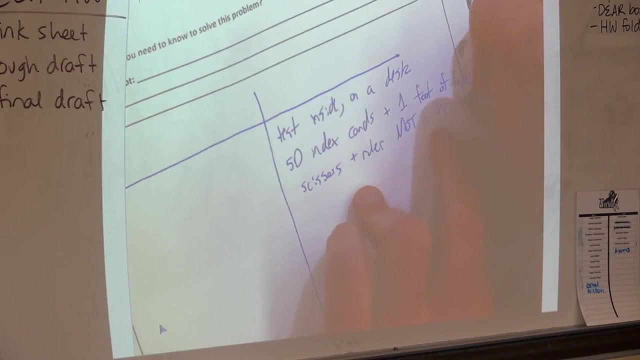 50 index cards and one foot of tape. You may also use hands down for just a minute. You may also use scissors, Scissors, Scissors, Scissors, Scissors, Scissors, Plays, Plays, Plays, Plays. 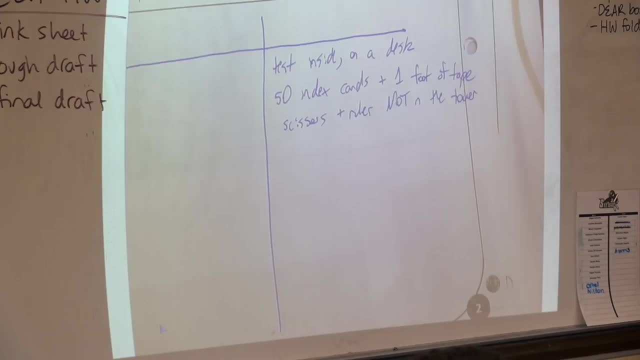 Plays, Plays Plus- crueler, but not in the tower. So you can use them to build. but, Anderson, can I actually put the scissors and ruler in my tower? I cannot Give me a thumb when you have those written, and then I'll take the next question. 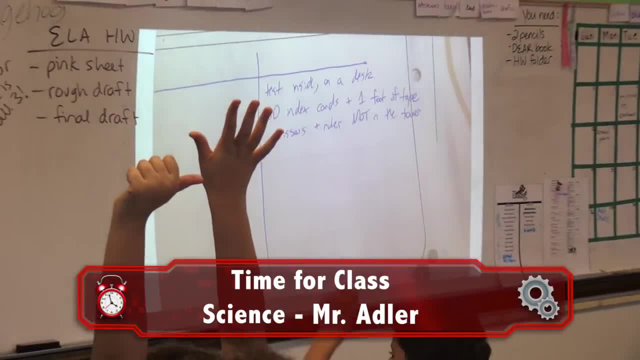 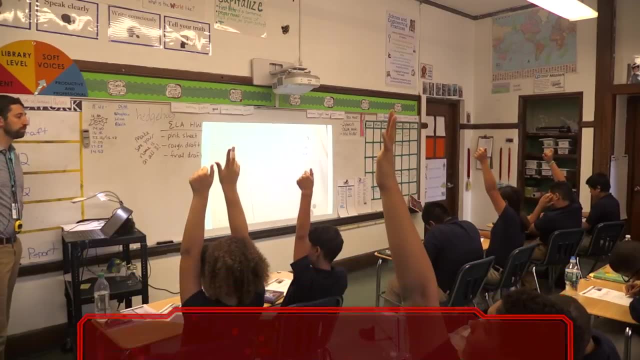 Ready, Ready, Ready, Ready. I'll give you 10 more seconds before I take the next question. What else do you need to know? All right, Let's go. All right, next question, Frandy. what do you need to know? 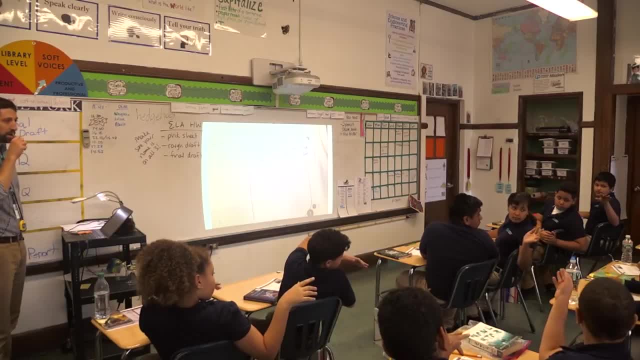 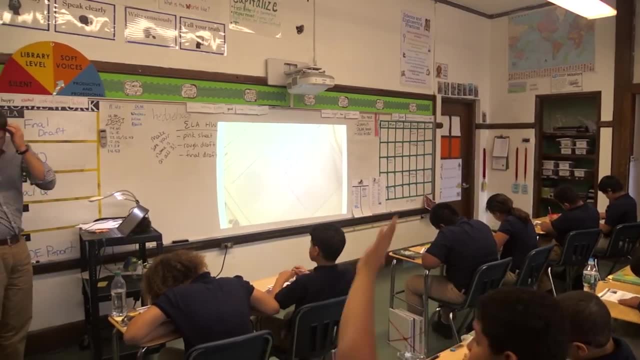 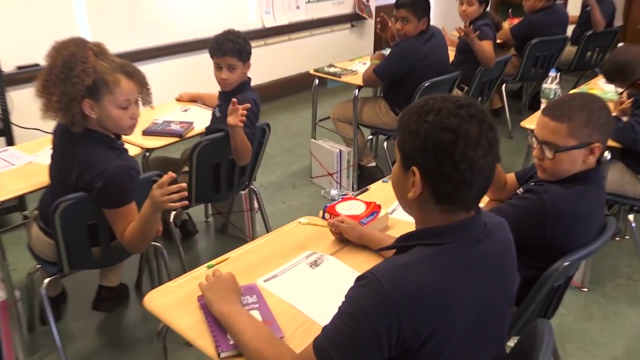 Hands down track. Frandy, I need to know how long it will take to build. Ah, great question. You have 20 minutes to build. 20 minutes to build, Angel. what's your question? How long are we going to build the tower? 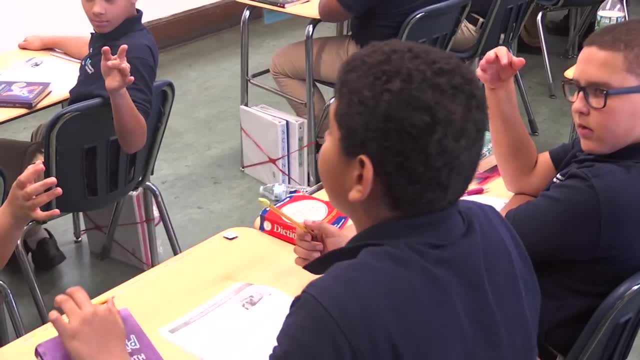 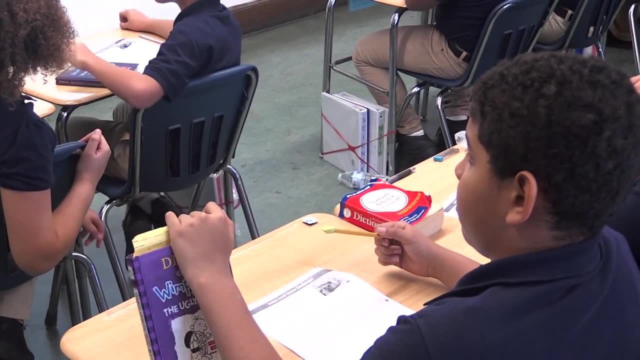 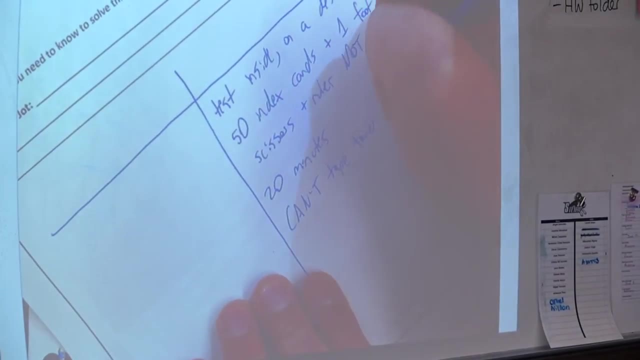 Hands down, shining on him: Well, you're going to have these materials on your desk. The one other rule that could answer his question, hands down, is you can't tape tower to desk, So you can use tape, but, Jalen, can I actually tape the tower to my desk? 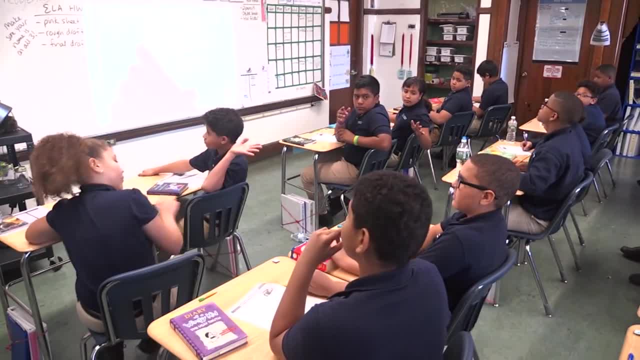 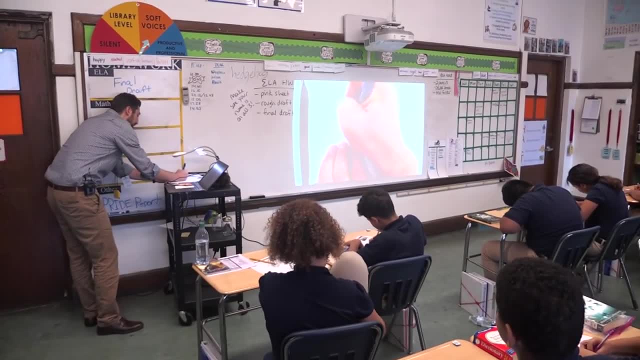 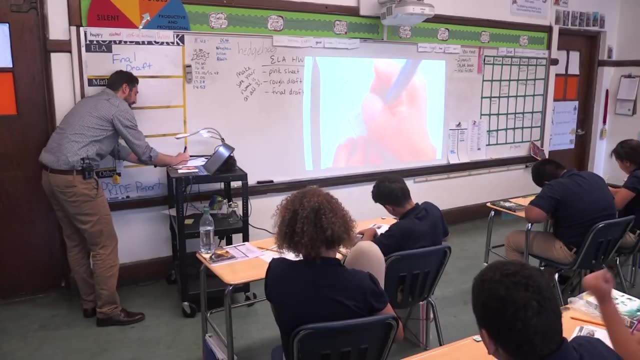 Hands down track Oscar, if you're done writing. Oh, you're placing Glenn on top of the tower And that I can actually put. Glenn must be on the tower for 10 seconds. Glenn must be on the tower for 10 seconds. 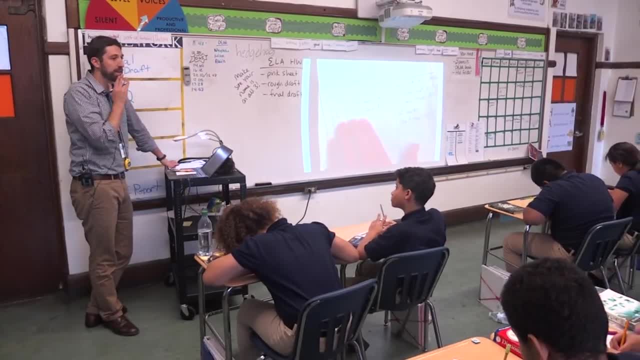 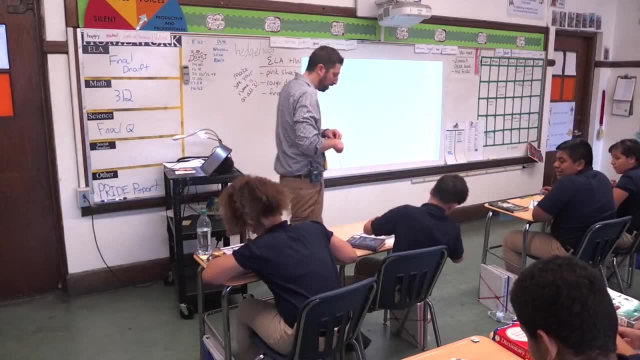 And Carlos asked a really important question about the weather. Guys, I have bad news. It's really really windy today. Antoine, can you lend me your binder please? So once we put Glenn on top of the tower, Glenn must stay there for 10 seconds. 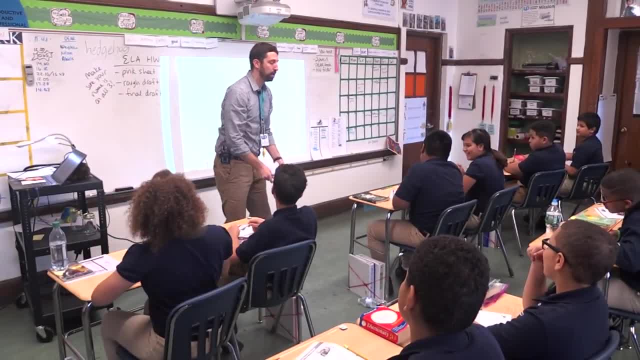 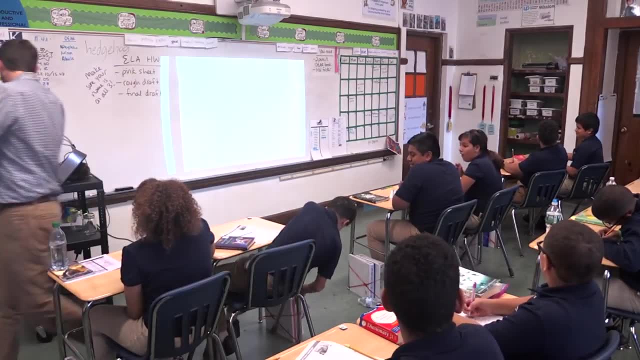 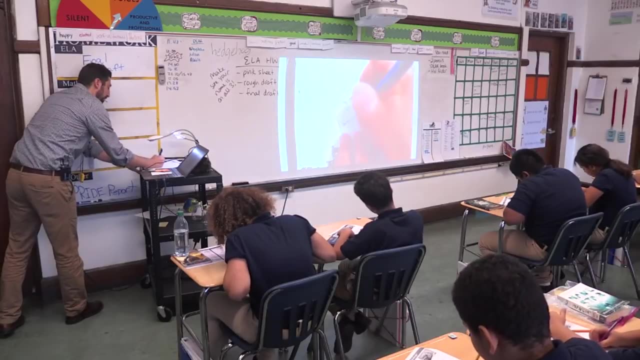 But then there's going to be a little bit of a wind today And the tower has to stand up to wind for three seconds. So I'm going to add that below Glenn must be on the tower for 10 seconds. Tower must stand up to wind. 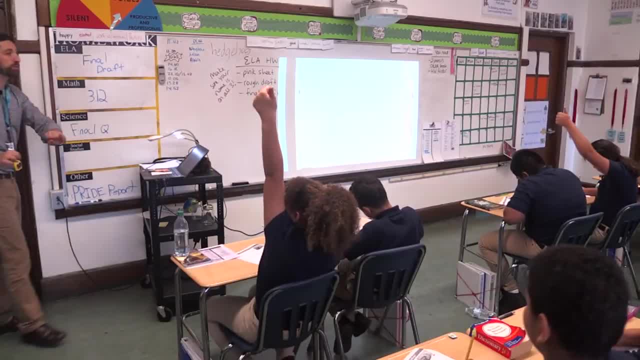 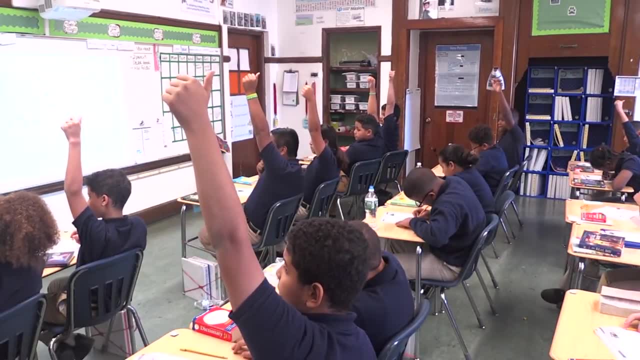 Tower must stand up to wind. Give me a thumb when you have those written. Jose looks ready, Nileshka looks ready. You guys are crushing it. Thumbs down. There's only one question you did not ask me yet. Well, actually two. 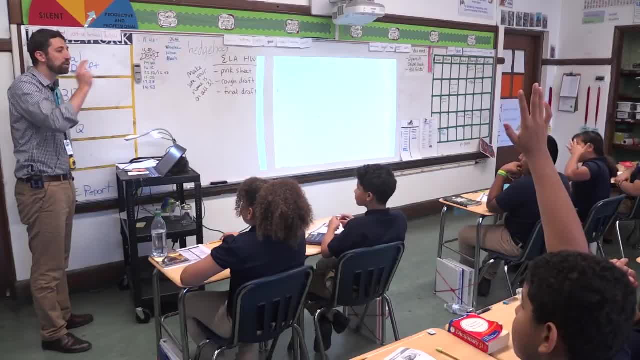 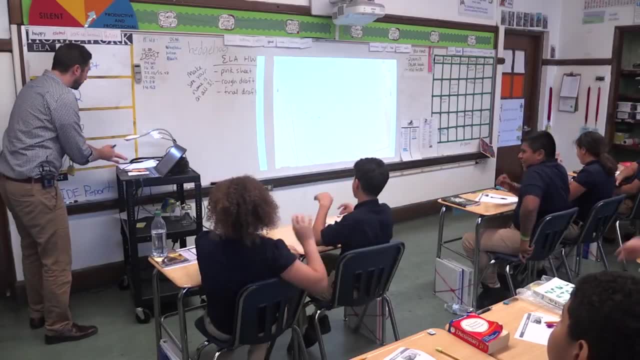 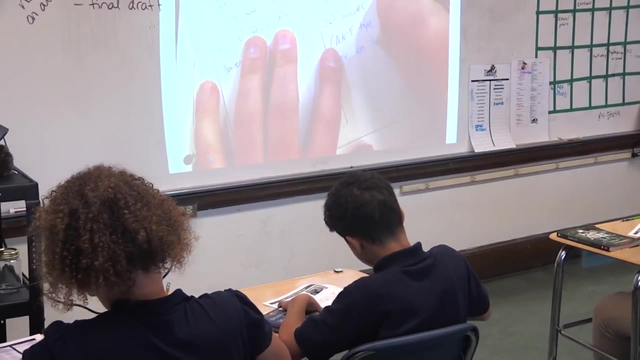 Two Hands down track. one, Luis, What is Glenn's height and weight? So if you know the tower's weight, That was one of my questions, which is, I won't tell you his weight, But I will tell you you can hold Glenn. 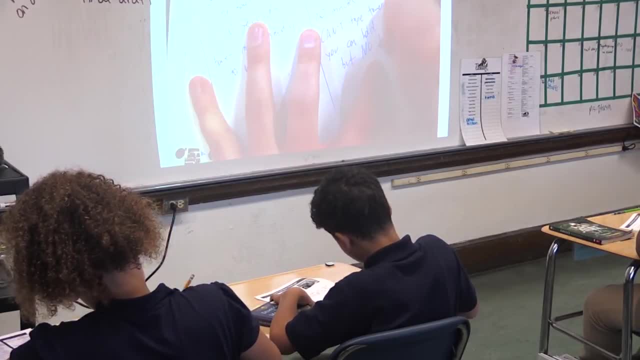 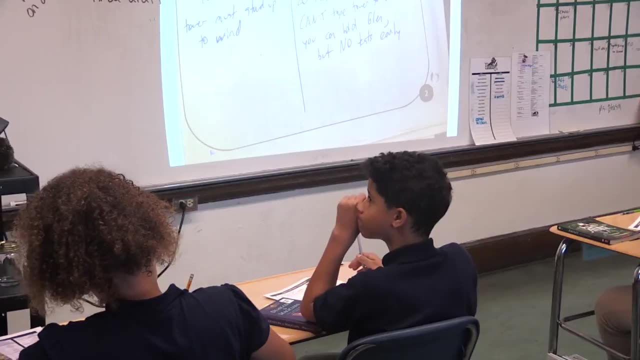 But no tests early. You can hold Glenn, but if you put him on your tower early you will fail the challenge. So if you ask me, Mr, Can I see Glenn? I will say: sure thing, You can hold him. 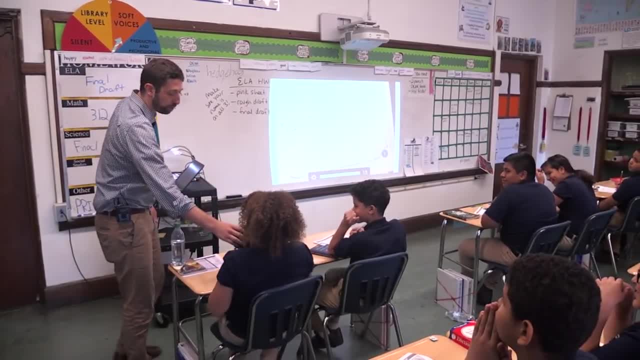 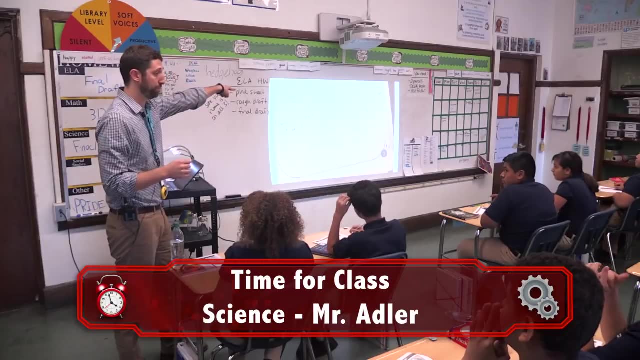 You can hold him, It's okay, He won't bite. You can hold him and feel how heavy or light he is, But you cannot put him on the tower early. There's only one question: Belongs on the left. He must be on the tower for 10 seconds. 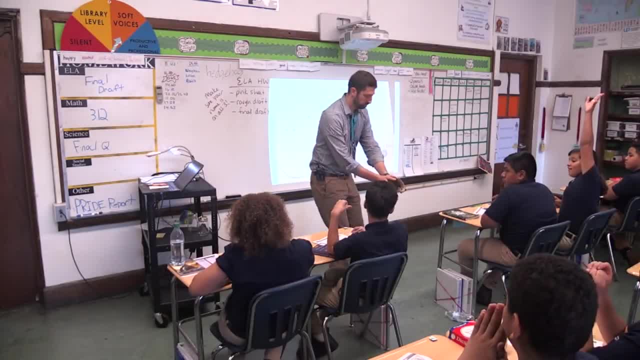 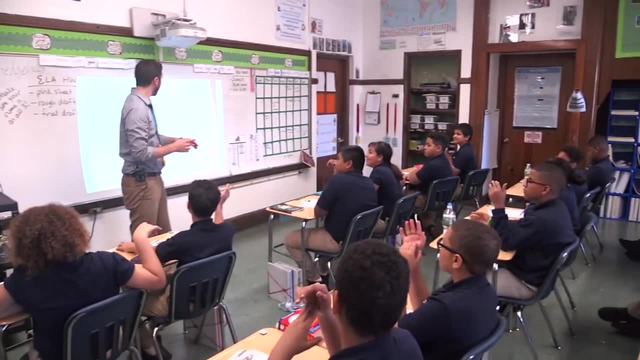 The tower must stand up to wind. What do you think? the last question you should ask me is: Hands down track Jalen, if you're done writing, He can't fall. Well, that, I think, is over here, because he needs to be on the tower. 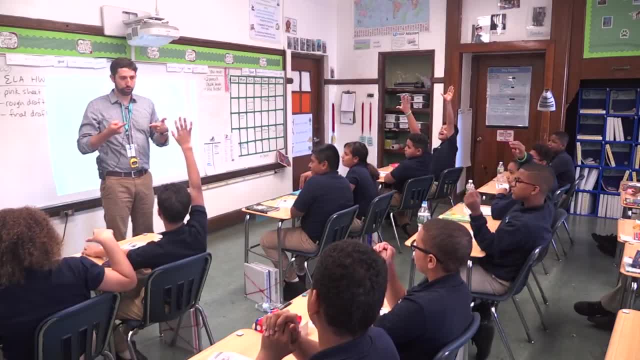 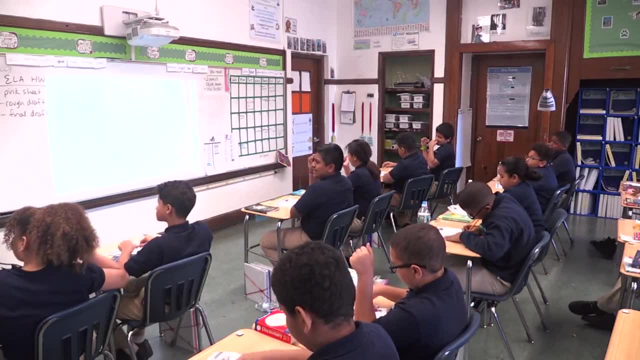 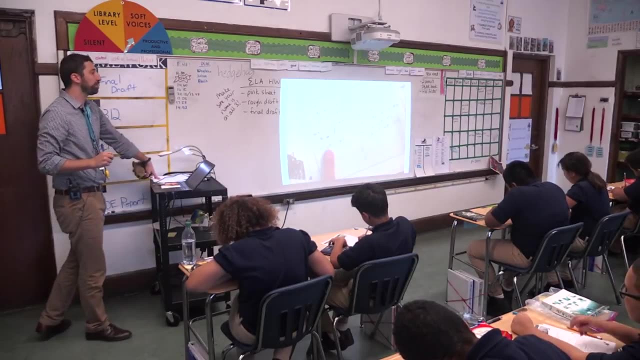 I can't see Glenn. He's too far down, So what question should you be asking me? Hands down, track, Antoine. That is the final question, which the answer is. your tower must be 15 centimeters tall. What does CM mean? again, Wilbur. 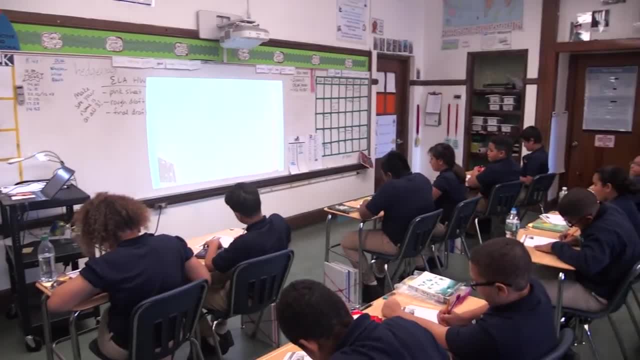 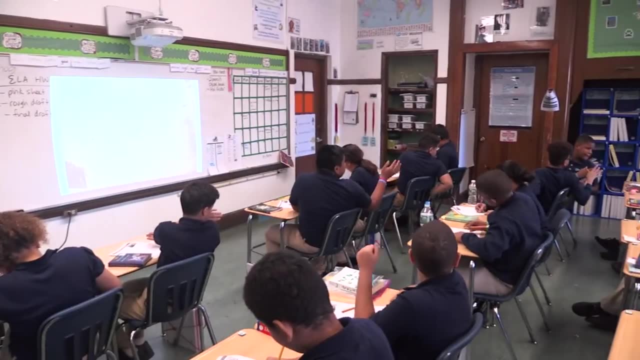 Centimeters Your tower has to be. how tall Darwin? 15 centimeters tall Is correct. Final question: when you're done writing track, Jose Mateo, What's up? Do you want to do it on a group or one? 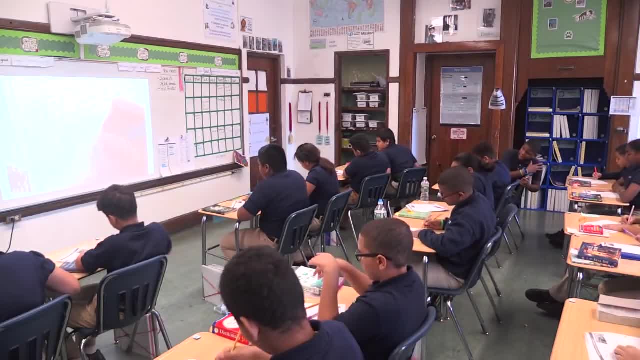 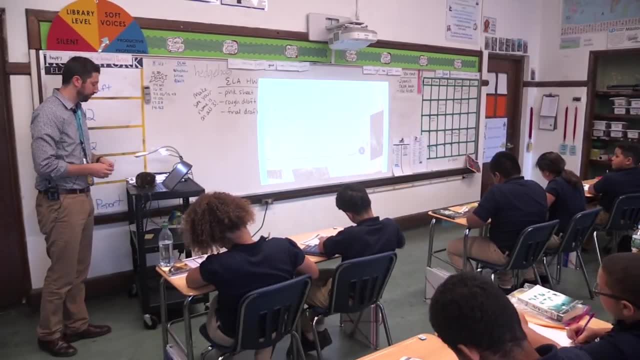 Ah, I'm going to put that over here. Your groups are two or three and I have made groups for you. I will tell you what they are in just a minute. Now, how much time do you have for this challenge? How much time? 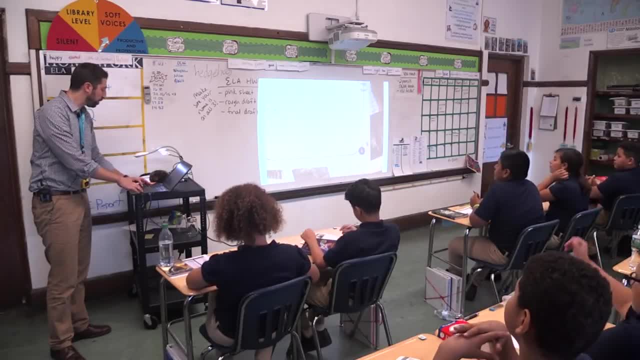 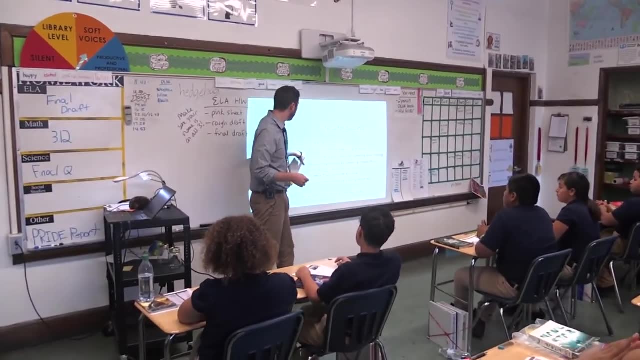 How much time do you have, Carlos? 40 minutes Exactly. Let me show you how you will meet success today: tracking me. once you're done writing, I see you, Darwin. Carlos, To earn a four out of four today, you must brainstorm before beginning to build. 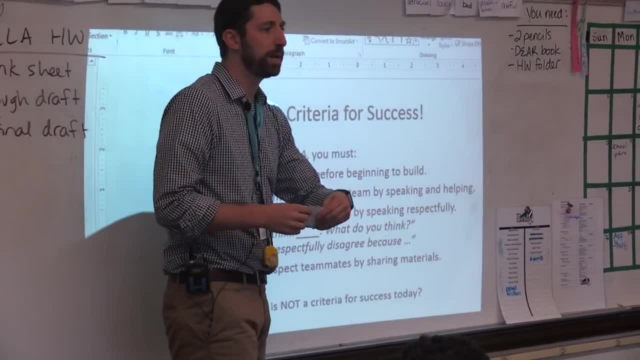 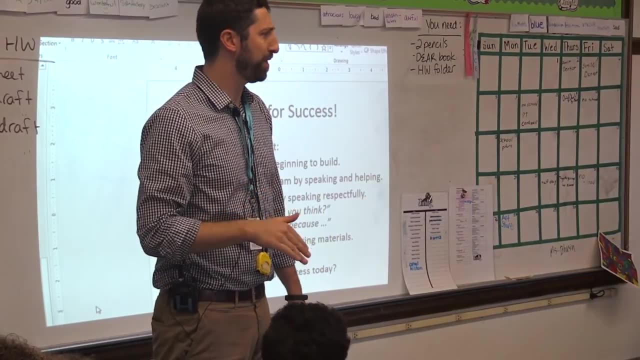 The next page has brainstorming space. What does brainstorming mean? Hands down. tracking Frandy in the middle Merit for that Good answer. So if Jose is in a group with Darwin, for example, track me. They would need to think together. 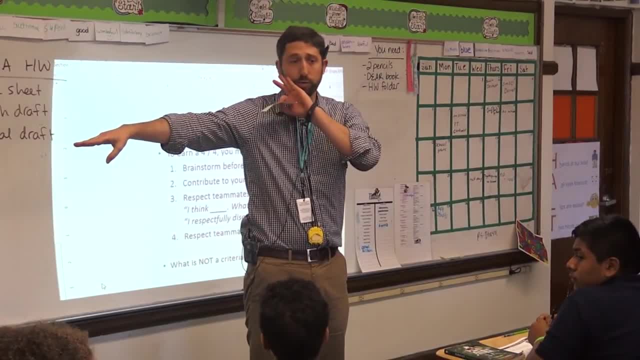 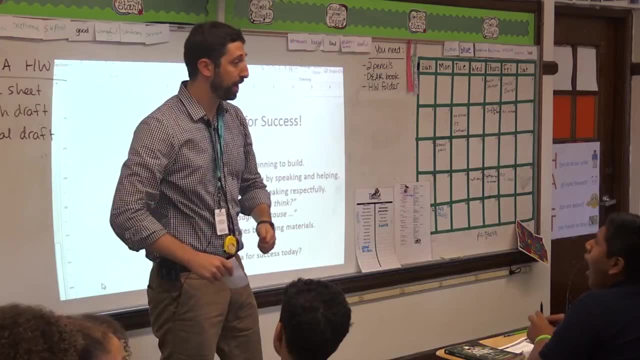 And have some ideas down before they get their materials, which are over here. Your second point is you need to speak to your team and help your team respectfully. One Lewis, second to Merit Hands got to be down. So, for example, if I see Jaylen not talk the whole time, she will not get that point. 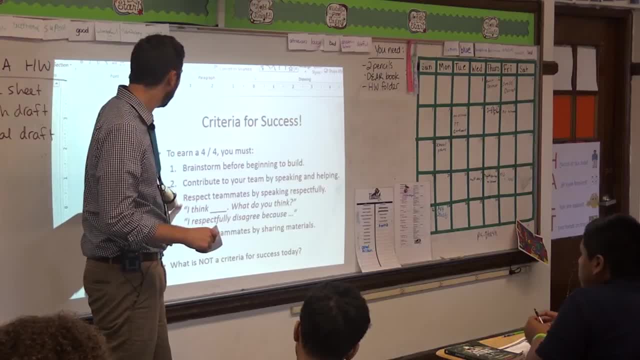 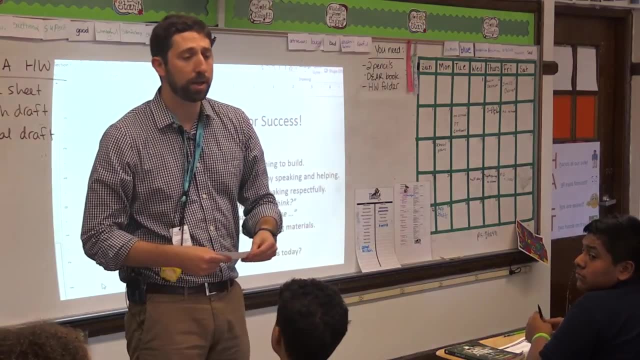 Third is respect teammates by speaking respectfully. I think blank. what do you think So? for example, if Oscar has a great idea, he can't just talk, He needs to say something like: well, I think we should use the cards this way. 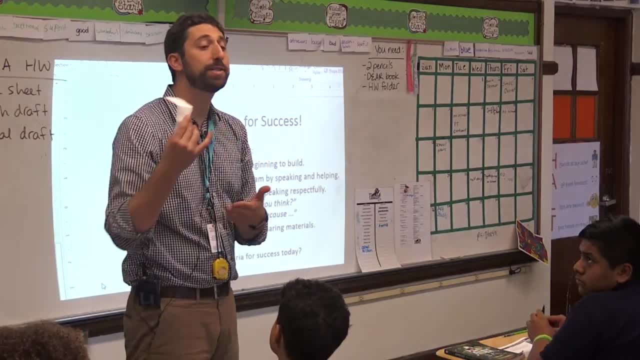 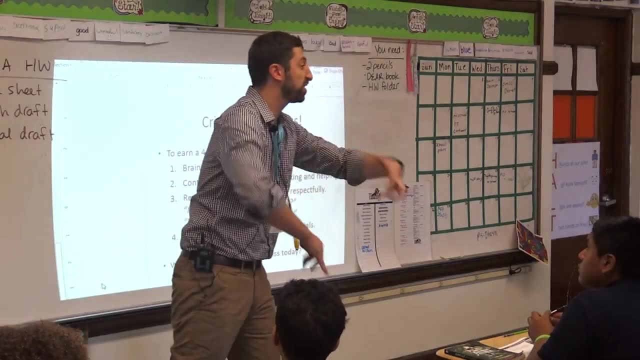 Angel, what do you think? And make sure that his teammate gets to speak too. And the last point: you have to share materials. If I see someone go- no, the index cards are mine- and not actually share any of the materials. 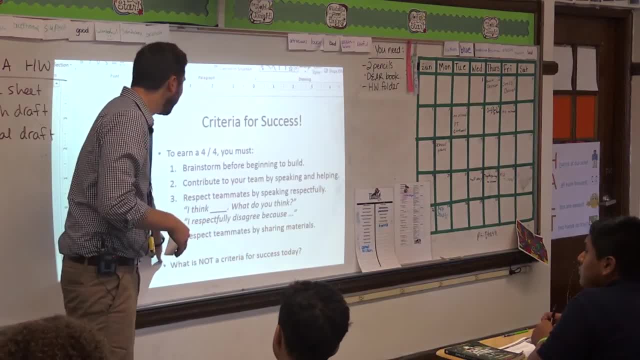 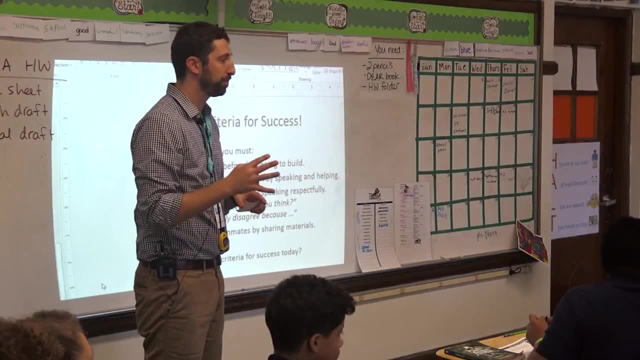 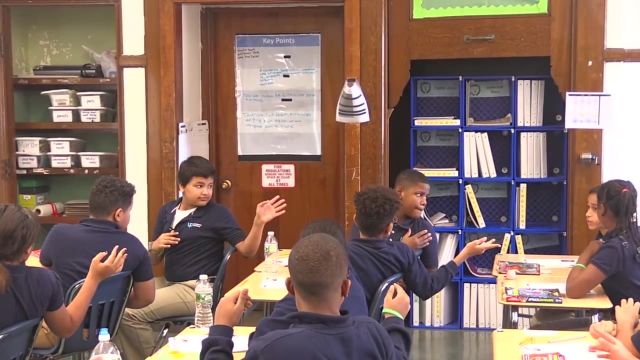 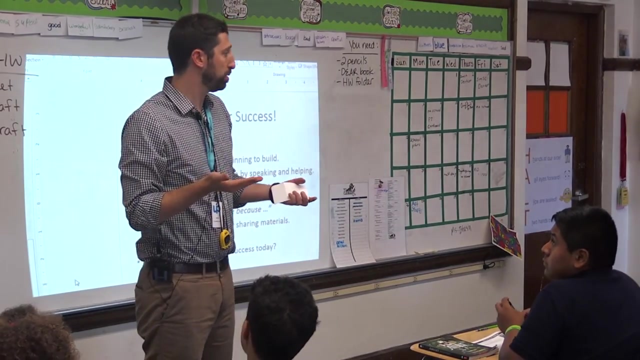 you will lose that. fourth point For Merit. what is not a criteria for success today? What's not on this list because you're not graded on it? Hands down track. Jose Mateo, If you don't finish posture, check a lady's Merit. you're not going to lose and you could still get a four out of four. 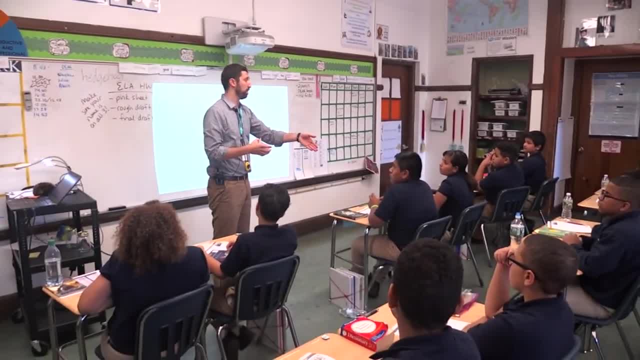 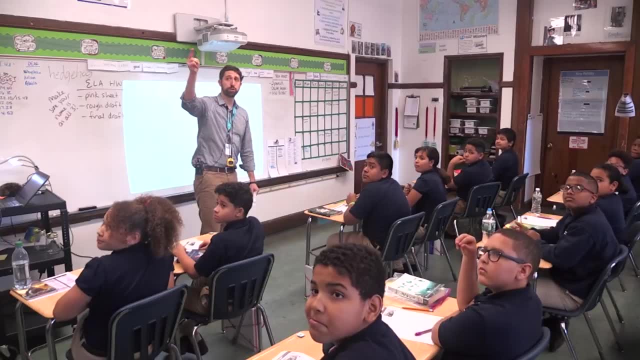 Also, if you fail, if Jose's tower doesn't work, can he still get a four out of four? And it is more important to me- track the pride values that I see you respect, your team track me by talking respectfully and sharing materials than that I see you succeed. 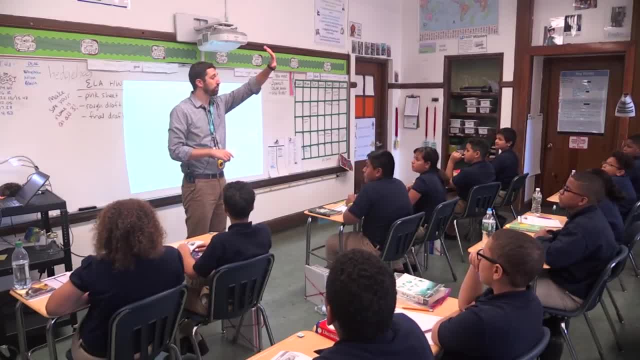 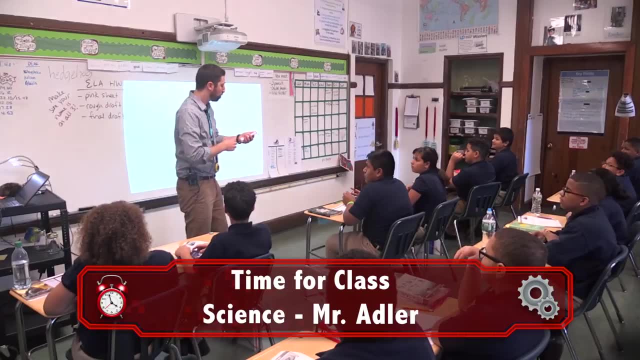 Capisce, Capisce. You're going to have 20 minutes. I recommend you do five for brainstorm, 15 minutes, 15 to build. I am going to tell you your groups. You can pick whose desk you build on. Group number one is Carlos and Wilbur. 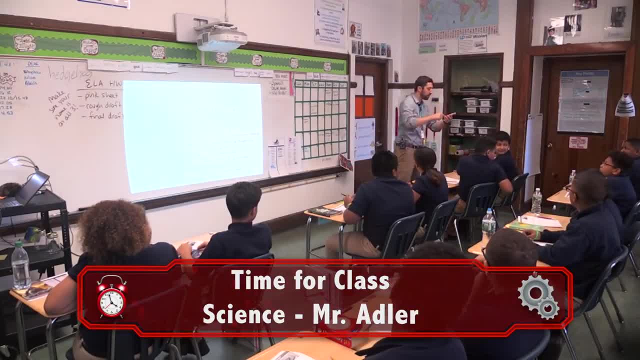 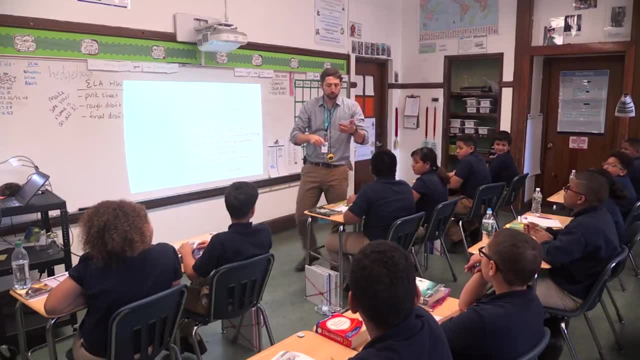 Group number two is Jose, Jose and the ladies. Group number three is Nilsson, Juan Luis and Jelmaides. Group number four is Franny, Jaylin and Anderson. Group number five is Omiel, Camille and Edgar. 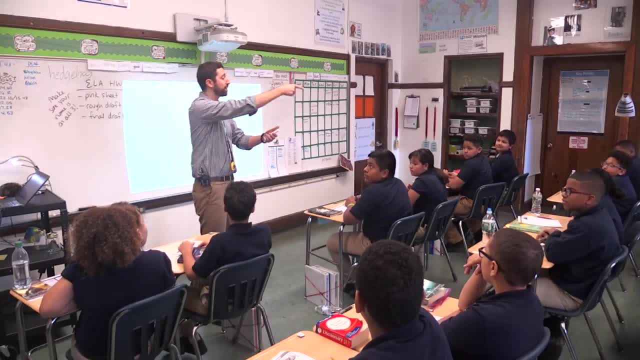 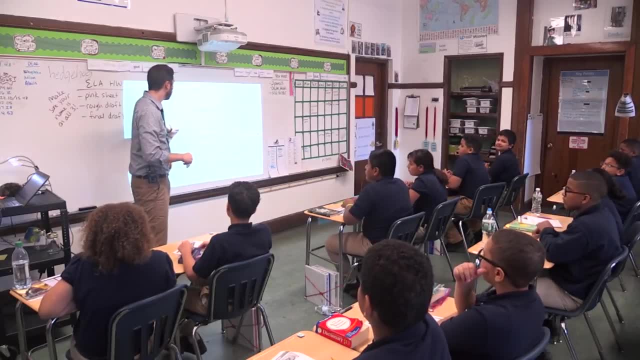 Group number six is Angel, Oscar and Darwin. You're actually going to come over and take one of these chairs to work with them. And group number seven is Nileshka. Antoine, Track me Thumb up or down. Can you get materials right away? 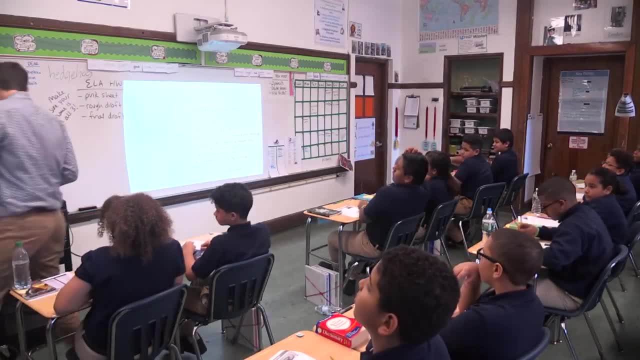 Excellent Thumbs down. Track the board. You have 20 minutes for this challenge. Oops, did that wrong. I did 20 seconds. That is not enough time, even for master engineers. Your 20 minutes begins now, Thank you. 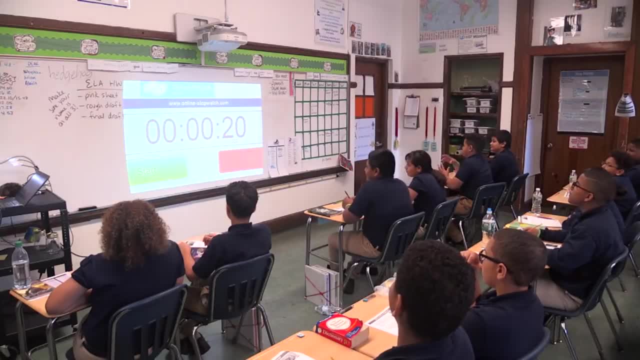 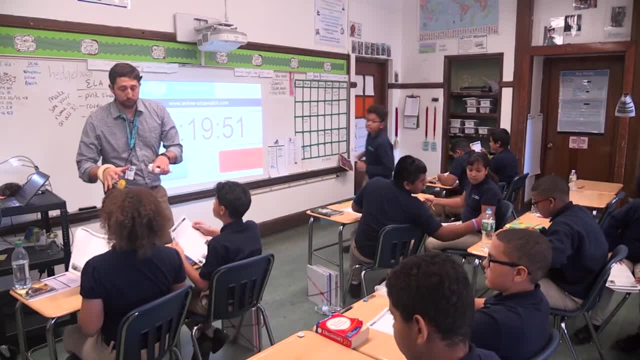 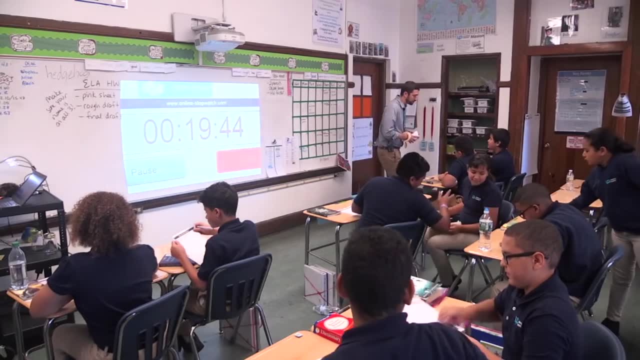 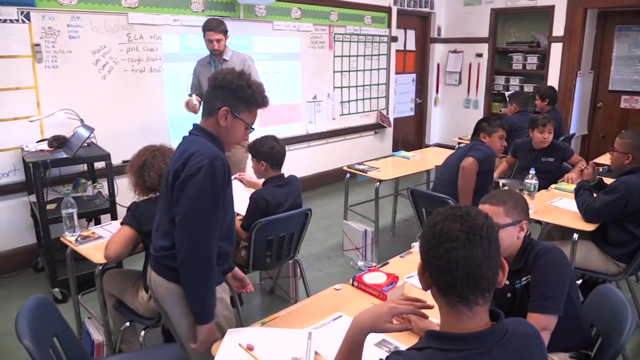 Thank you. So you guys only have two, which makes it even more important. you're sharing conversations and talking with each other, So I'm going to tell you what I told them: You only have two. It makes it more important you both step up to have good conversations. 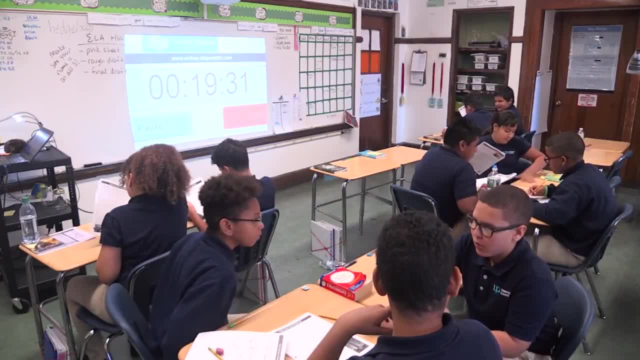 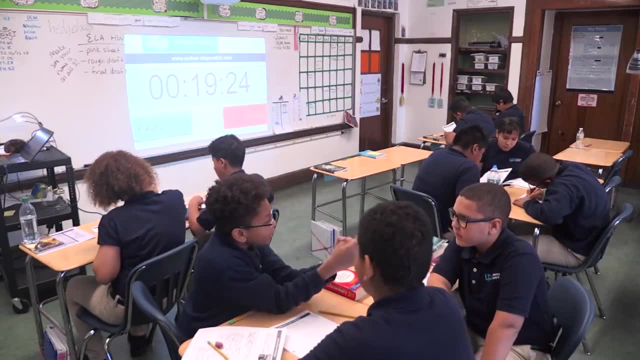 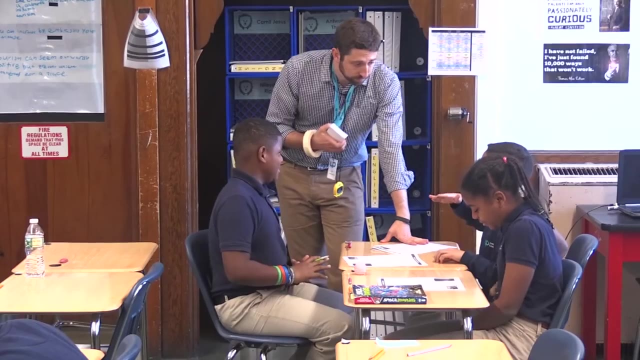 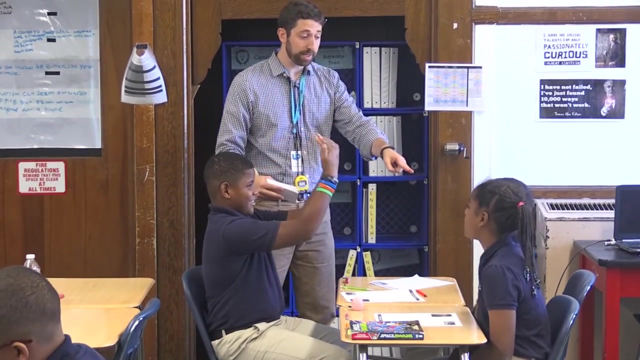 Okay, Okay, Can I pause you? One, I'm not a mess. Two, be careful. careful that everyone speaks. You can draw or you can write for your brainstorming. So you're telling me. who should you be telling this to? 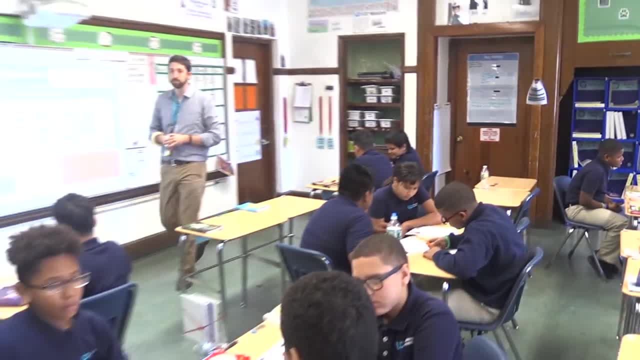 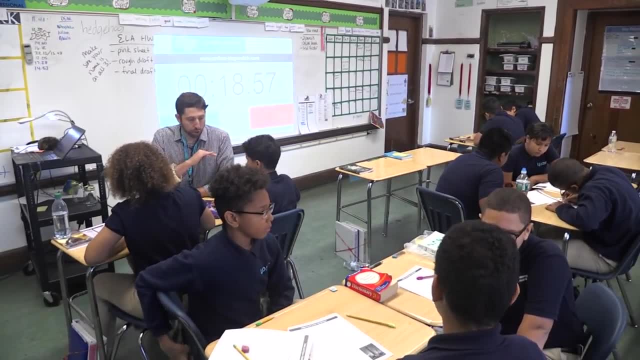 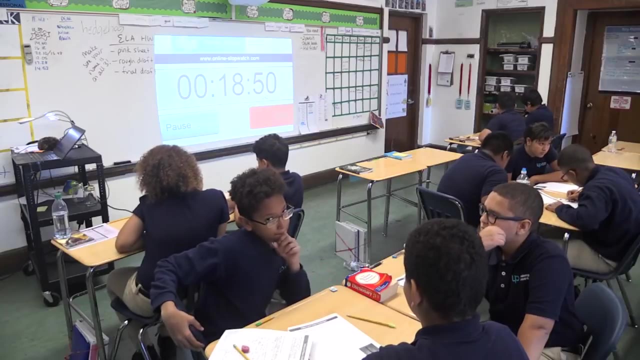 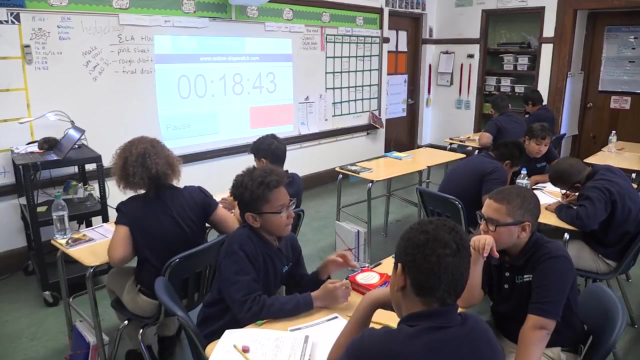 There are no requirements for width, Good question, Good question, Because that's not in the materials list. you can't use your binder, You can only use the cards, the tape, and I can use the scissors and the ruler to help. 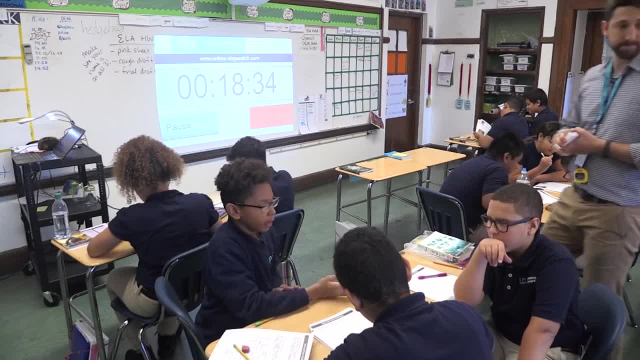 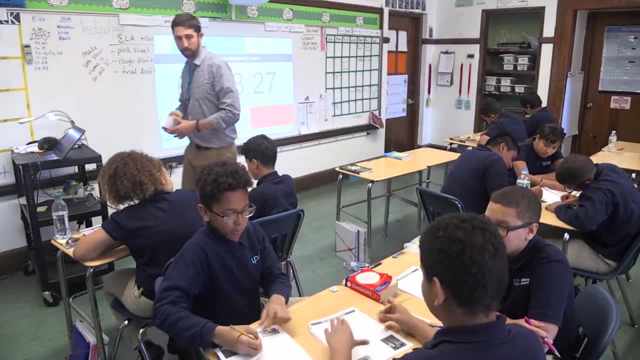 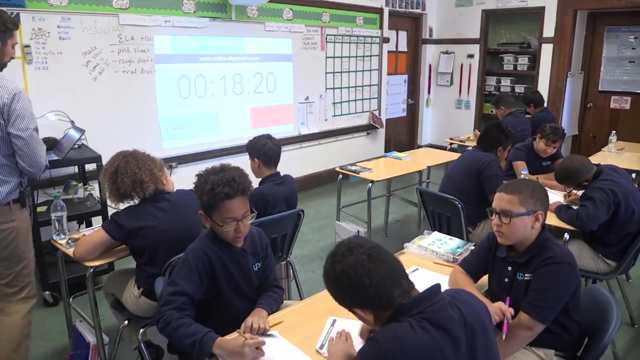 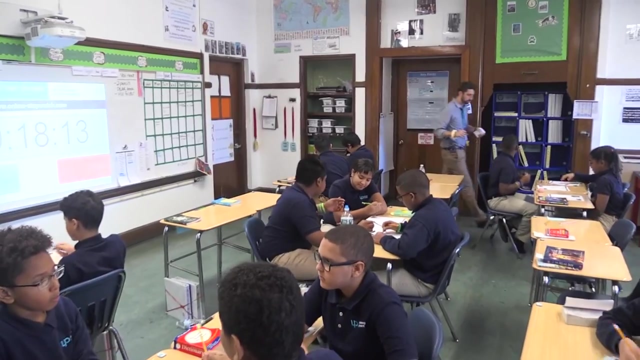 But they can't be in my tower. Not in the tower, just to help you make it. So are you guys drawing or writing your brainstorming? Are you guys drawing or writing your brainstorming? I don't care what it looks like. 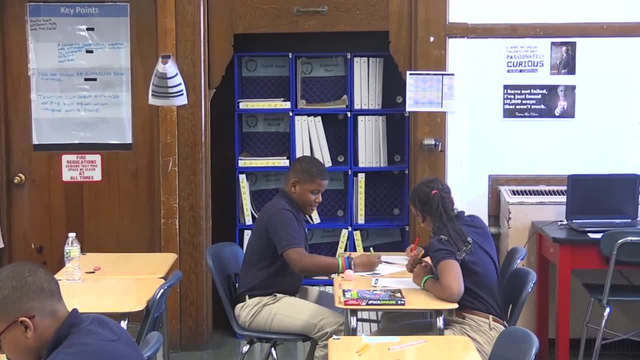 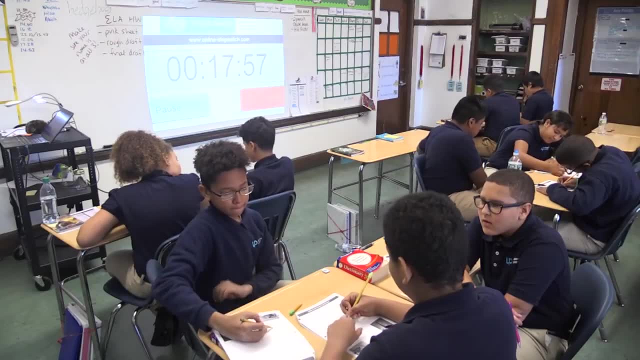 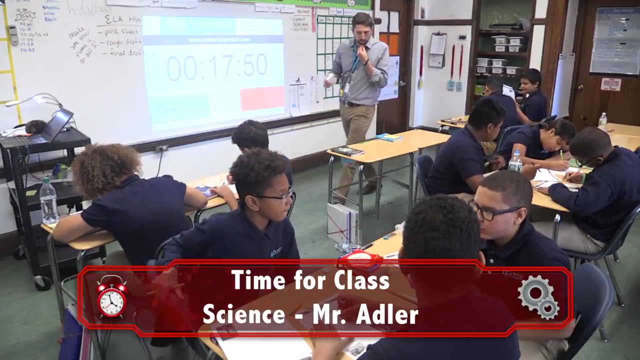 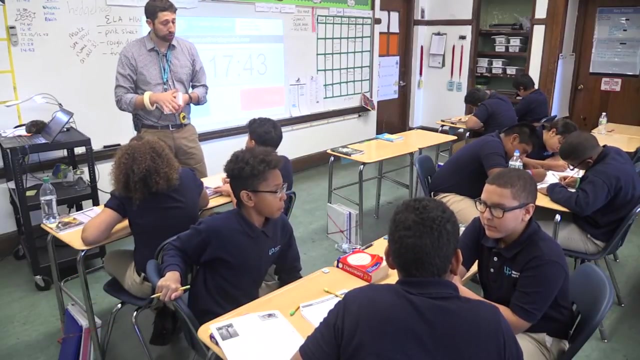 As long as you have some idea of what you're doing. okay, Merit. So you guys are writing down your ideas, Good, And you can draw to help you, or, if you'd rather, you can just write a couple of sentences, okay. 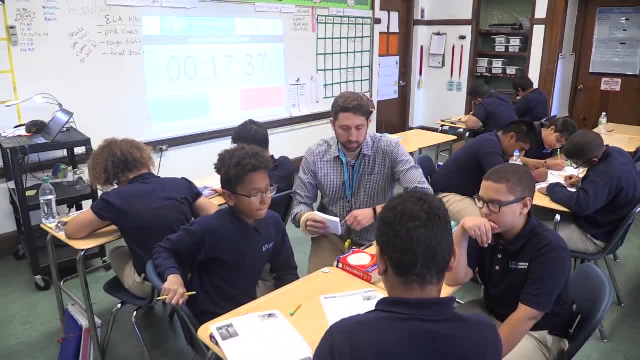 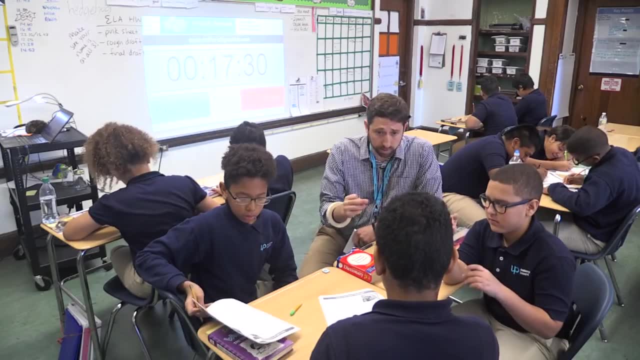 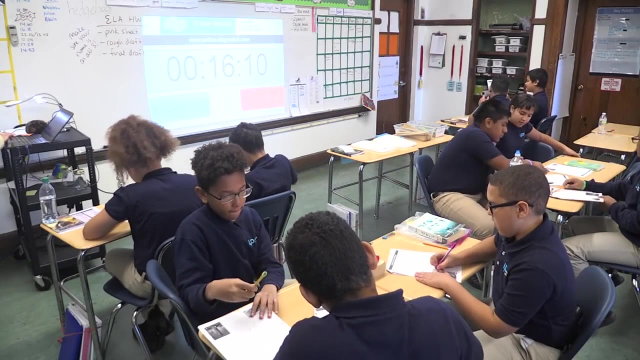 And Angel merit for going back to check the rules of the challenge. That's a smart idea. okay, Let's keep going. That's okay. Track me. Don't worry, I've stopped the clock. Your time is not continuing. 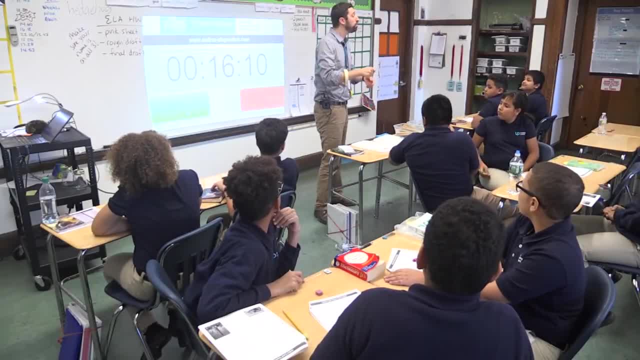 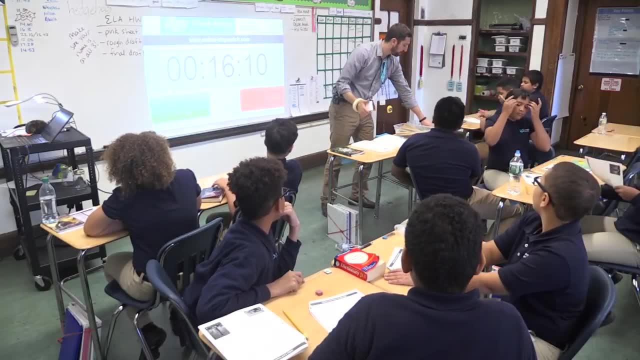 My first group is done. When you think your brainstorm is done and everyone has brainstorm written, hold up your papers. You will then get the following from me: Oh, I see a group has their papers up. Put your papers down. I give them one ruler. 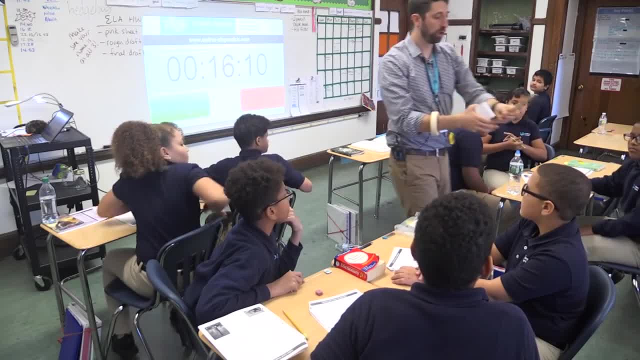 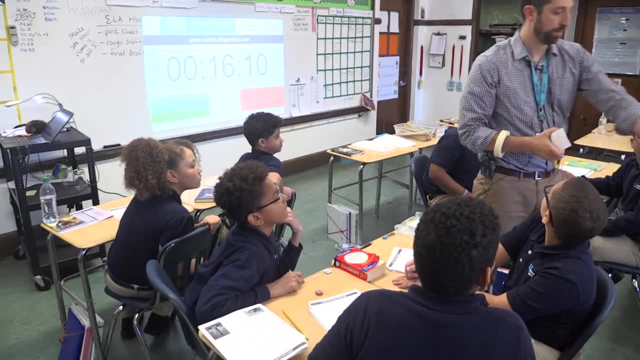 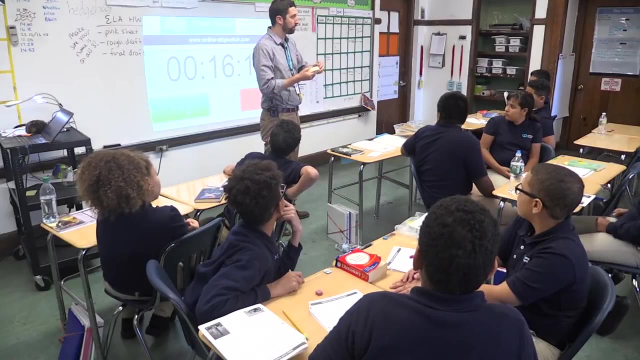 Jose de Merit, you should be tracking me right now. One ruler, One scissors, They get 50 index cards. And remember, you only get one foot of tape. Some people were asking me, Mister, how much is one foot of tape? 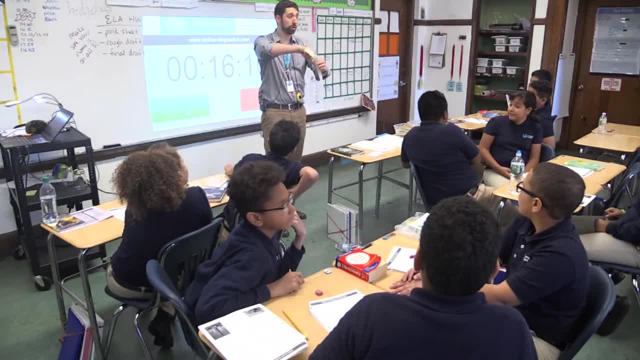 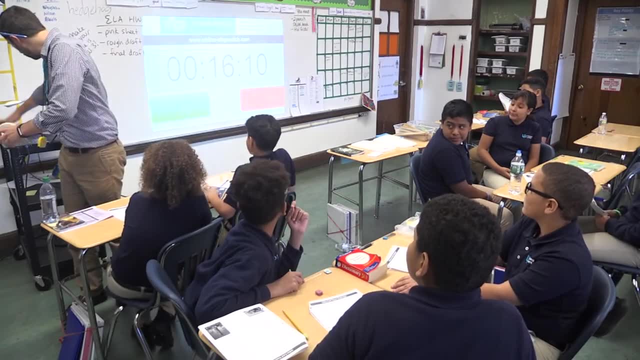 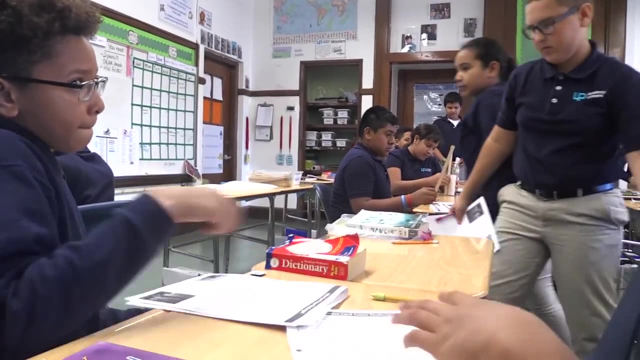 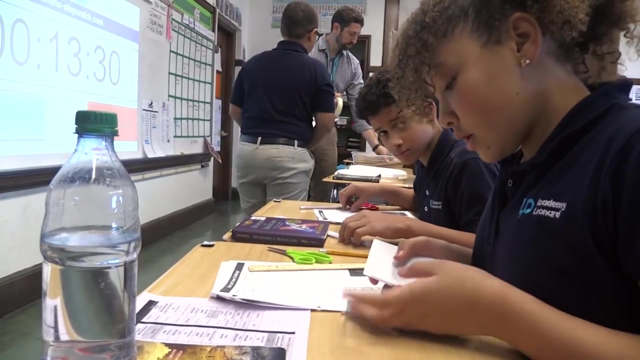 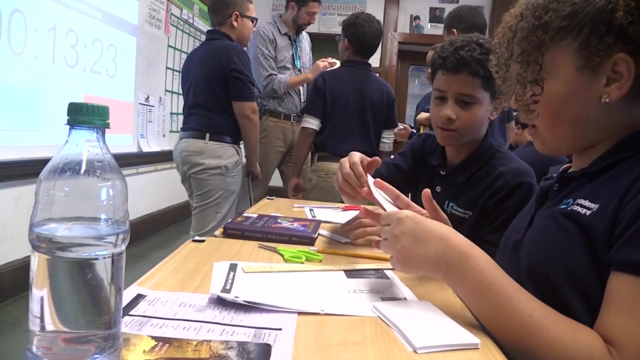 It's not a lot, It's only about that much. So be careful with your design. When I say go, I am restarting the timer. Go, And here, Okay, There are your cards. And then and, and wait, Y'all might, Y'all mighties, you need your tape too. 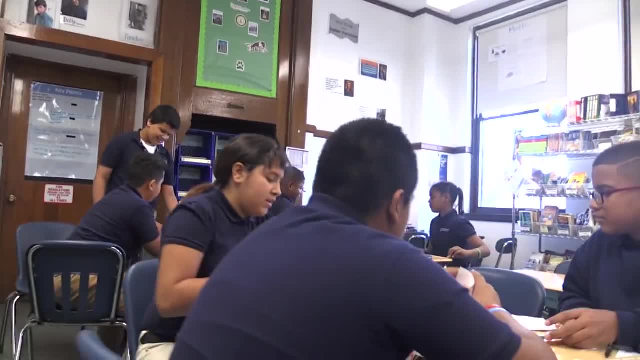 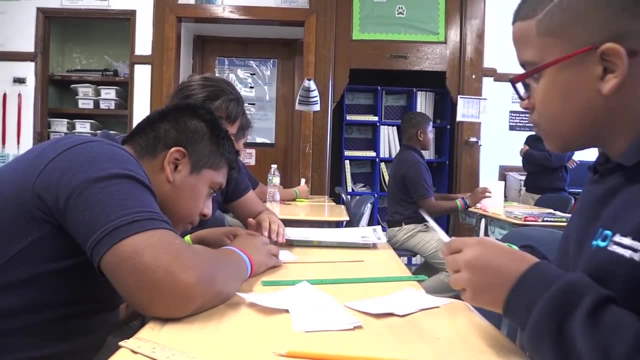 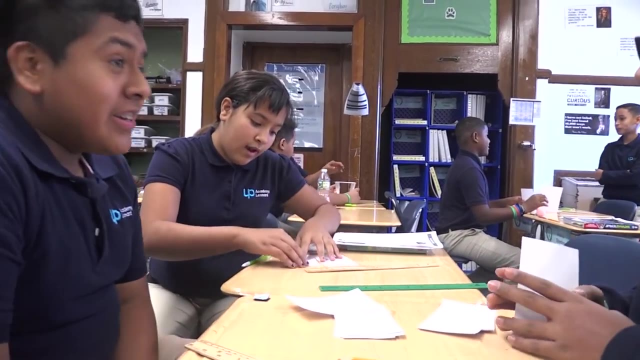 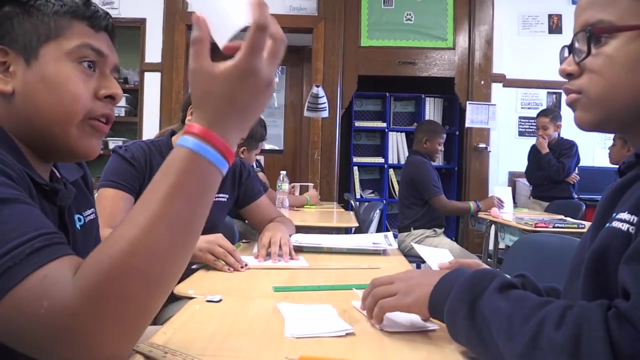 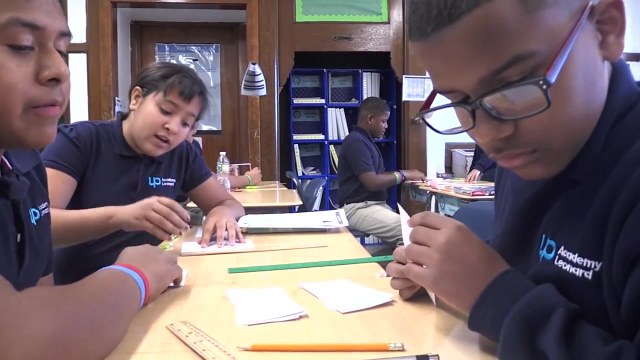 There you go. Alright, last group. Where's the rest of your group? Ah, they're still working. There is your index cards. Ready Ladies, Jose, do you guys need extra scissors or rulers? Now here's my question. I see you holding materials, him holding materials. what does? 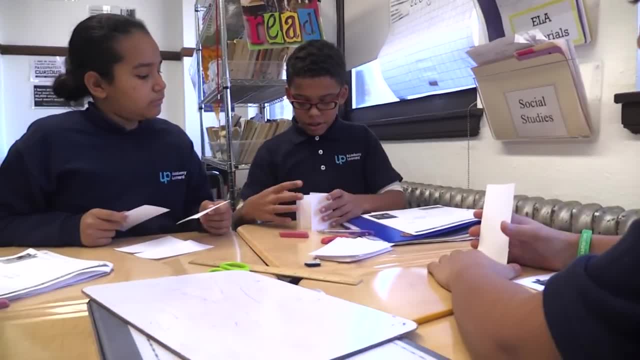 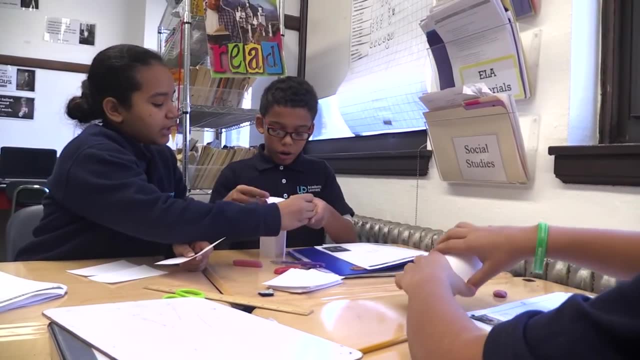 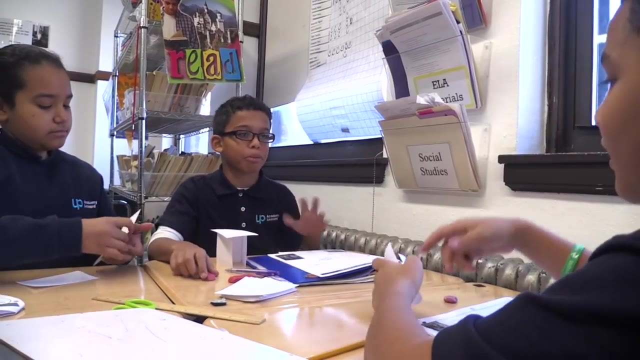 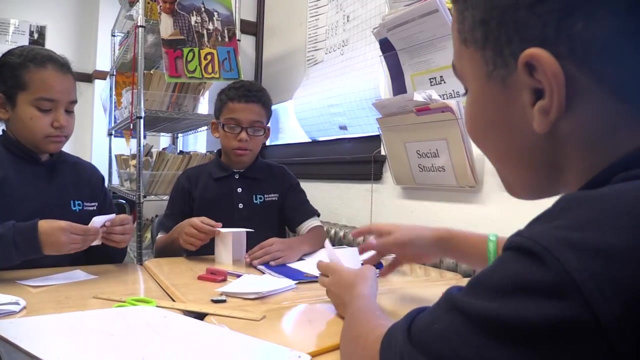 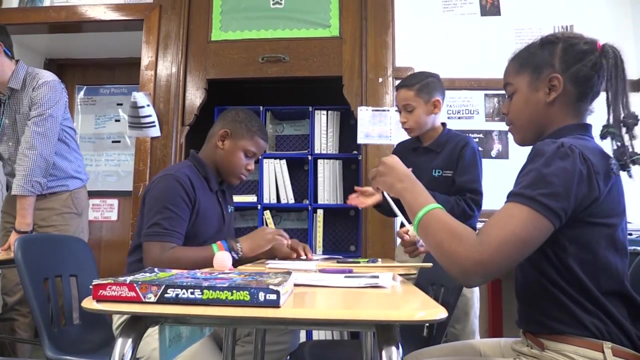 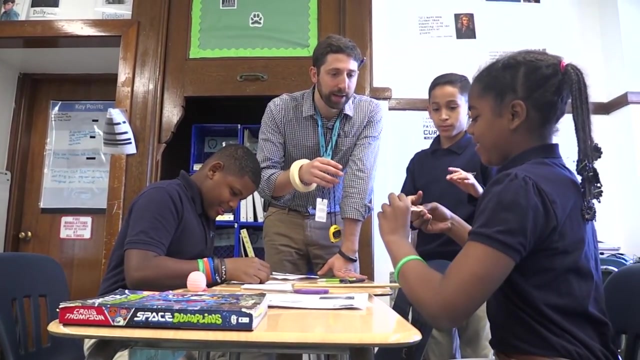 she get to do. Is that okay with you? All of the scissors Merit for the good thinking, But do you need that much tape to connect those two cards? It's okay. Now the tricky thing is: if this was a real, if you were a real engineer, you'd have to. 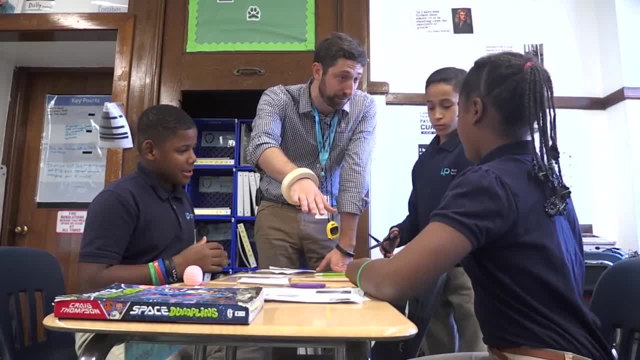 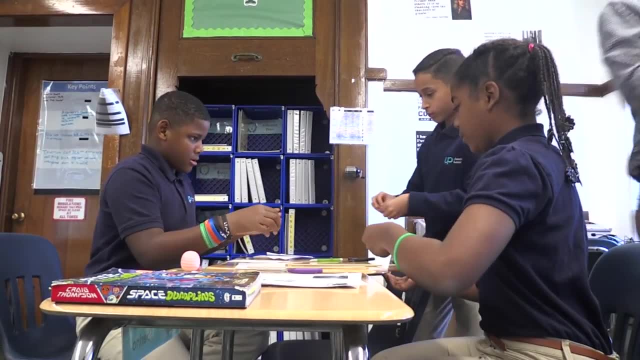 be careful with your materials, because could you go say: I'm going to go buy a lot more steel for my bridge? Nope, that costs a lot, It costs a lot. so be very careful with how you use your materials. Mister, is that? can we hold it? 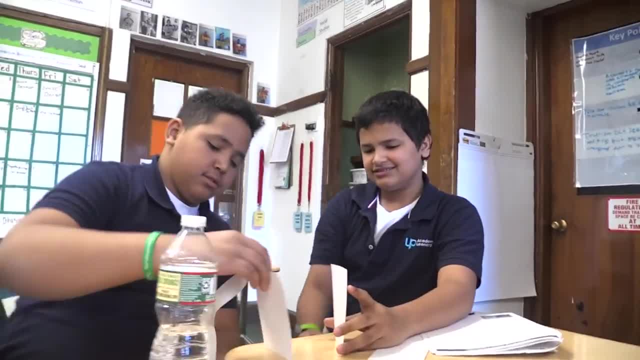 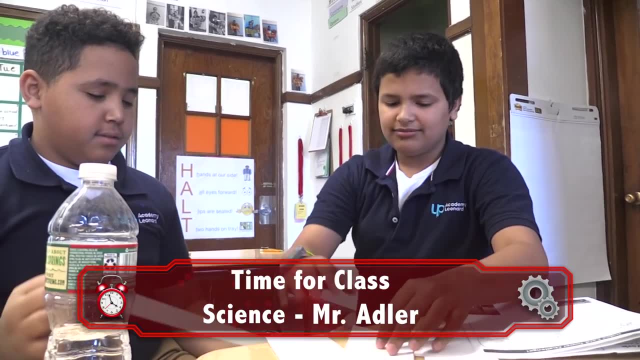 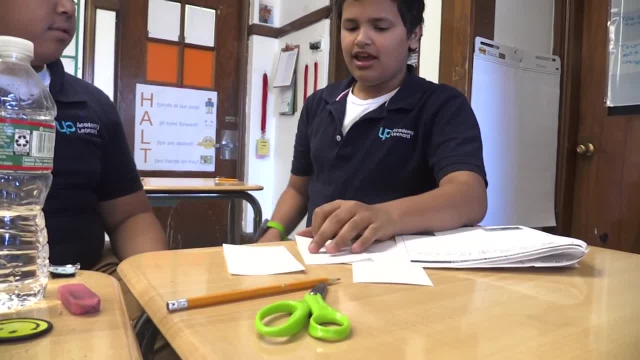 So what is your idea for your design? So our idea is to make a strong base and build it up. I like it. You know how Anderson put that in there. It go like that, Mm, Why are you using triangles? 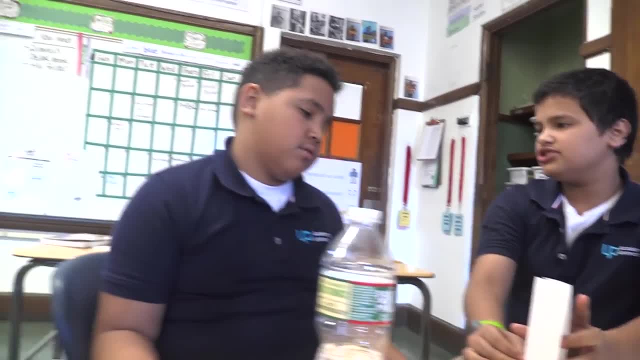 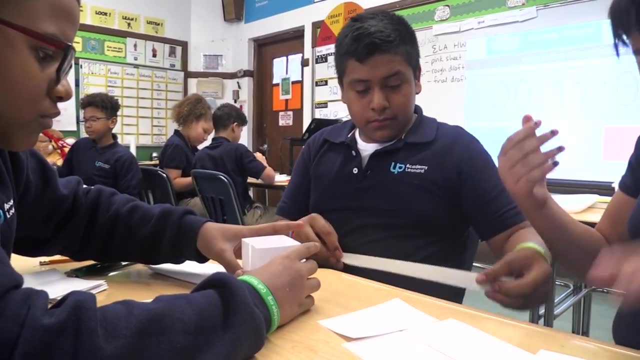 Oh, because when we saw the one like this and then we thought that we had to go with triangles like that, That's what it is- Because we thought that, you know, it's going to be like a triangle. It's going to be like a triangle. 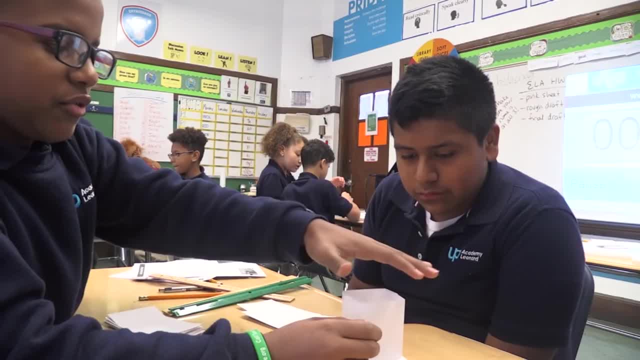 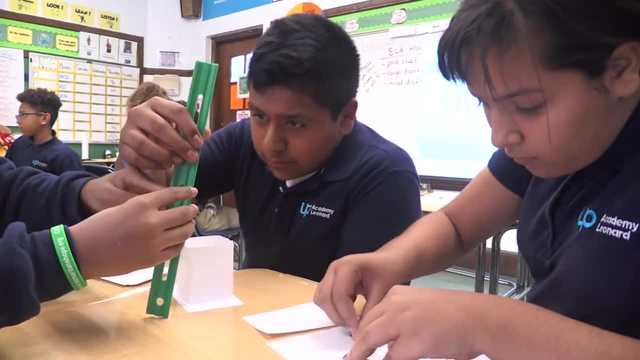 But it's not going to be like a triangle, Because we thought that you had to build it up. You had to add it up. How do you think you could make it more stable? Well, no, I think the triangles are stable, but is this your only base? 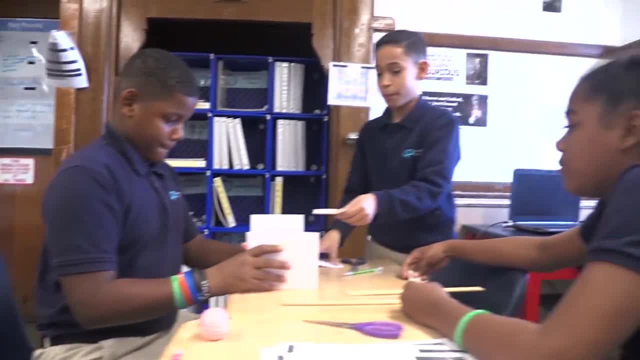 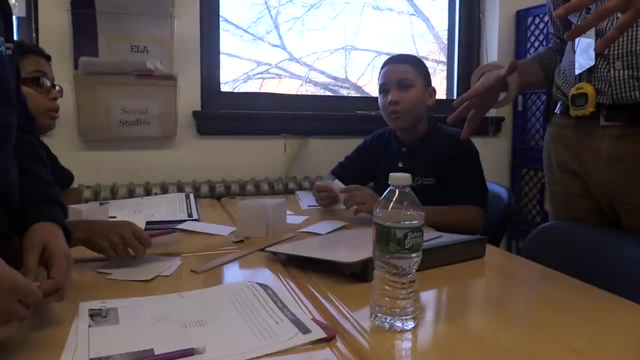 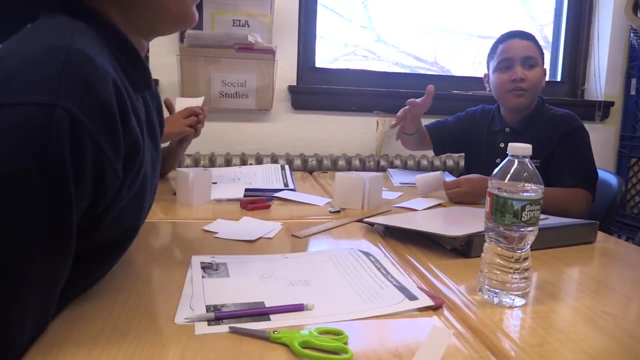 See, that seems interesting to me, because if we did that, what do you think the bigger base would do, Nilsen? Well, what would that do to the top if the base is stronger? I mean, what do you observe in the tower on your paper? 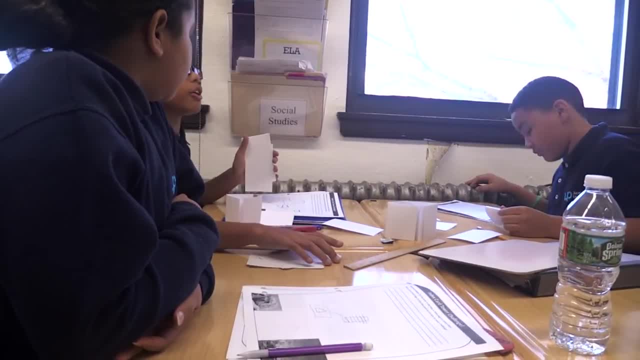 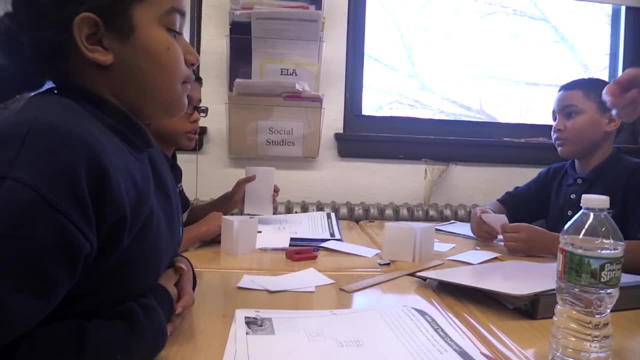 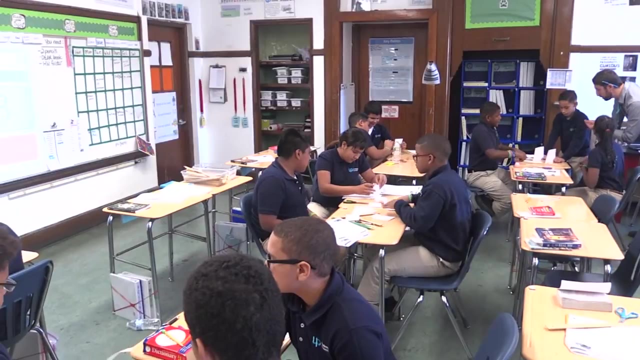 What does it look like in the base compared to the top? But where is it bigger? Use that in your design. Also, remember to keep checking the height to make sure it's on track. Track me. I'm going to warn you. your group is not on track for a 4 out of 4.. Why? 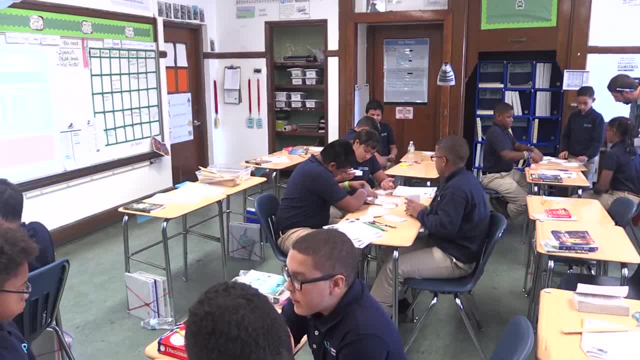 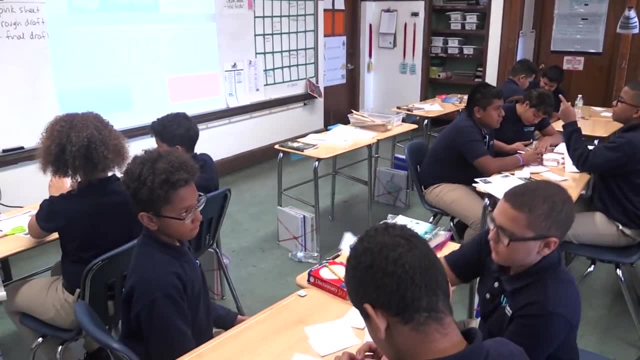 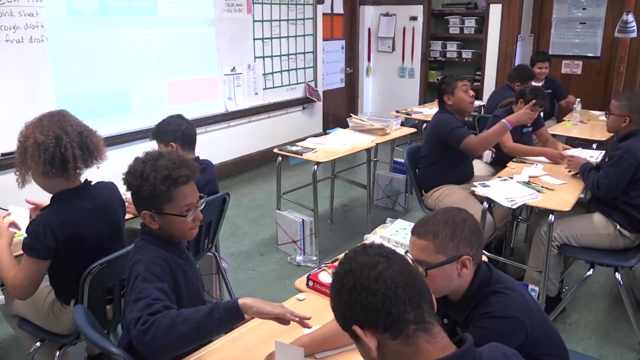 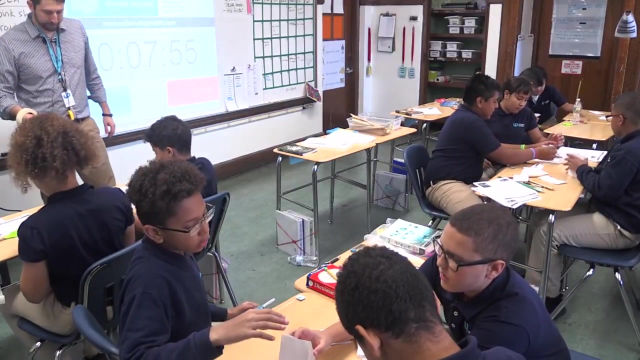 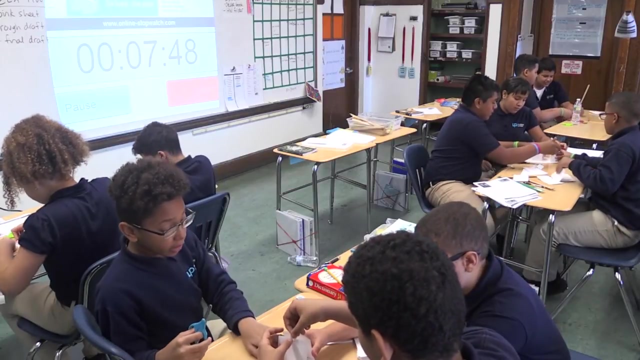 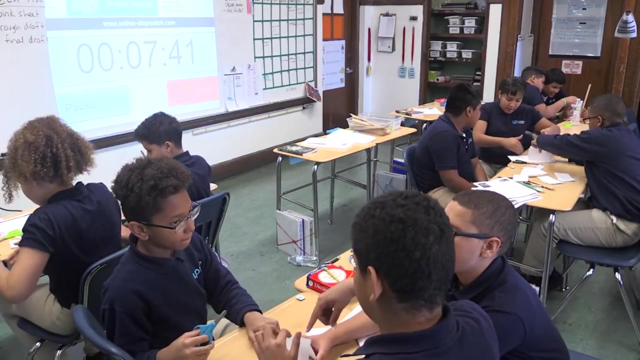 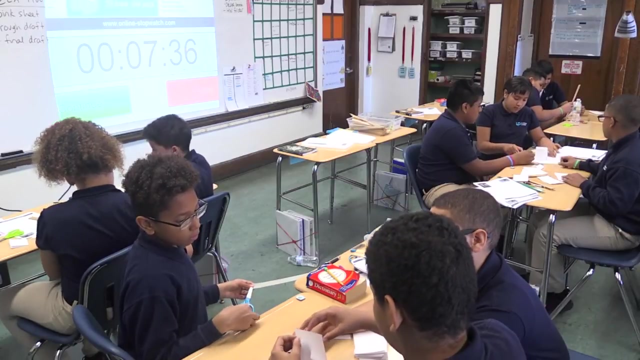 I'm still seeing you guys hold cards and her looking at you. Make sure you're on track. Make sure every teammate is getting a chance to hold the cards. Oh see, that looks very stable. That looks interesting. You have a choice? Track me. 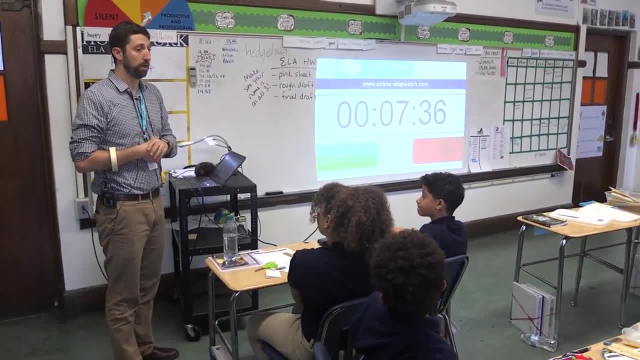 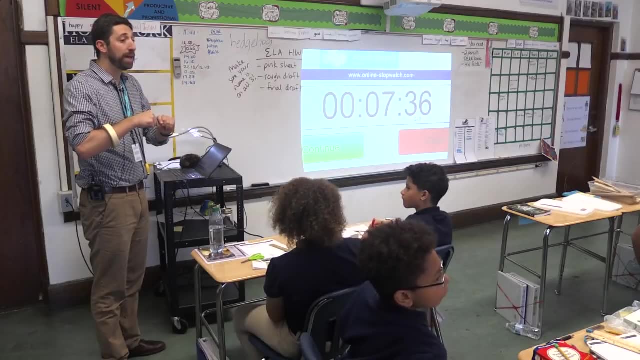 I am pausing the clock for exactly 2 minutes. You may either use it to continue building or you may walk around to see what other groups are doing. If you choose to walk around, you cannot disrupt them or ask them questions because they're busy building. 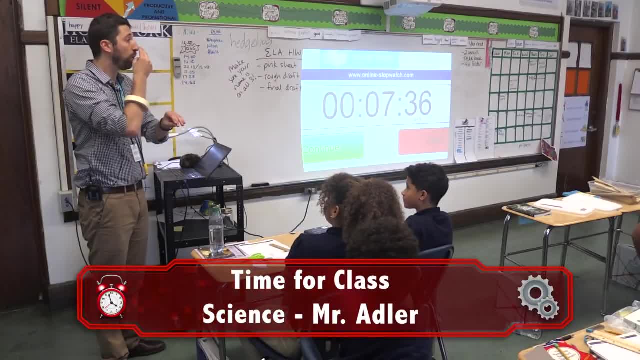 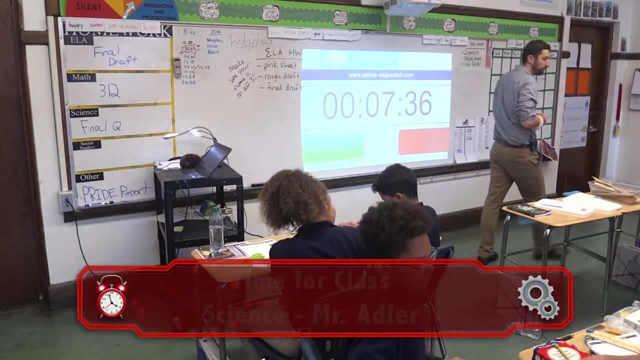 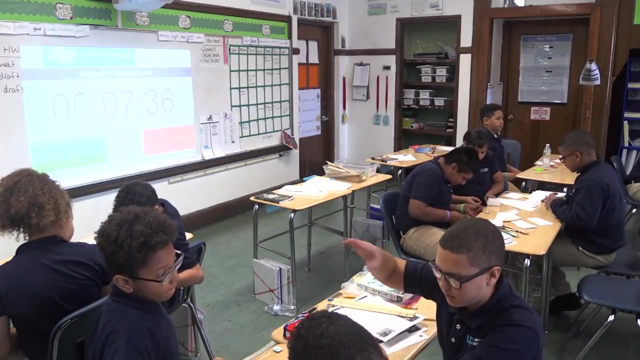 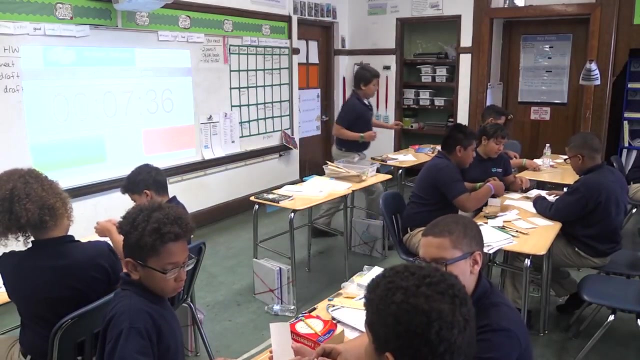 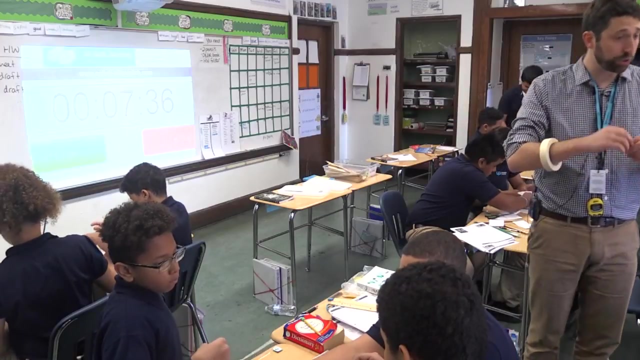 But you may either continue building or look at the other designs for the next 2 minutes. So we've got our base there. Is he making more triangles? I like it. Keep going. I think that could make it really stable. Omiel, when you get to 5 minutes remaining, use your timers, okay. 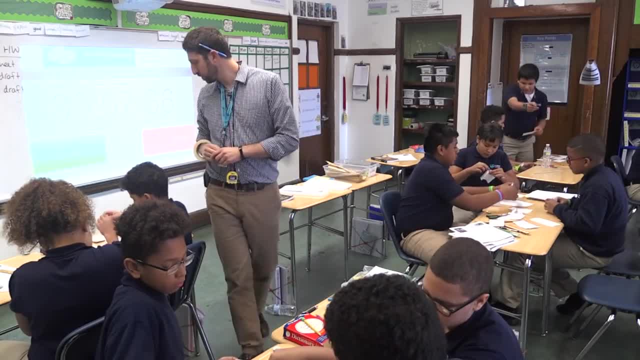 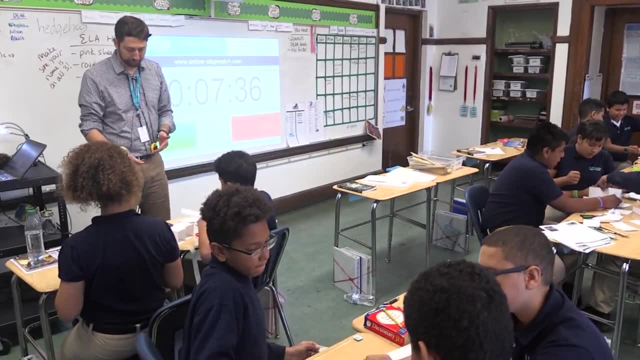 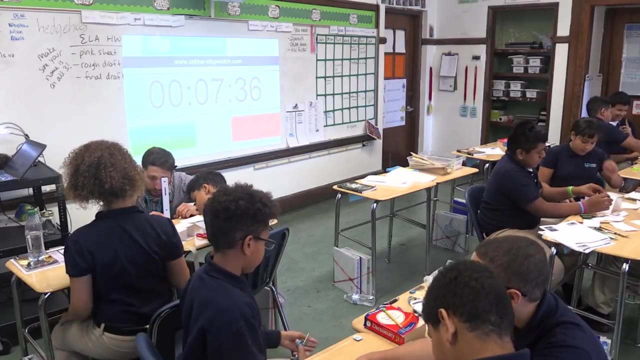 Good, Oh, so I see You're going to add up squares. How tall is each square? About 2 and a half centimeters, I think. it's taller than that. It looks like it's more like 7.. So you don't actually need that many more to get to 15.. 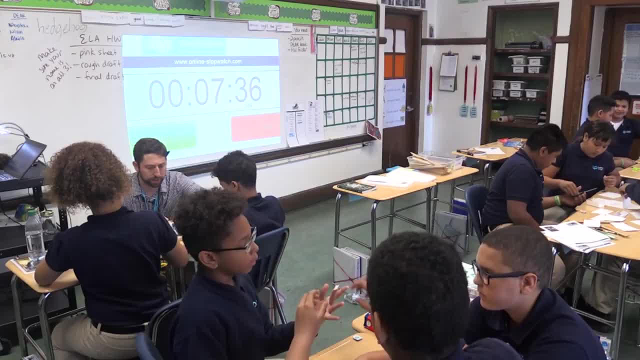 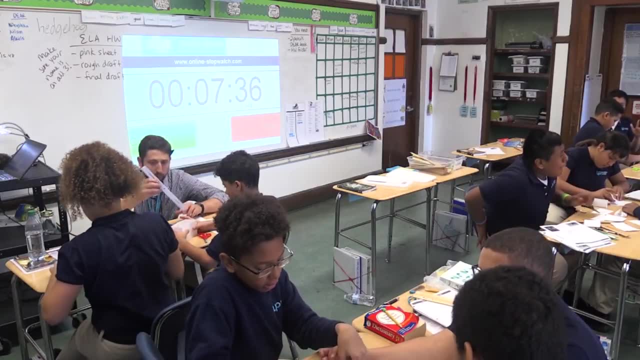 My only question is: why did you choose to add more squares? Why did you choose to put them the short way instead of the tall way? Well, could you do it the tall way now? Yeah, Because then each one is even taller. 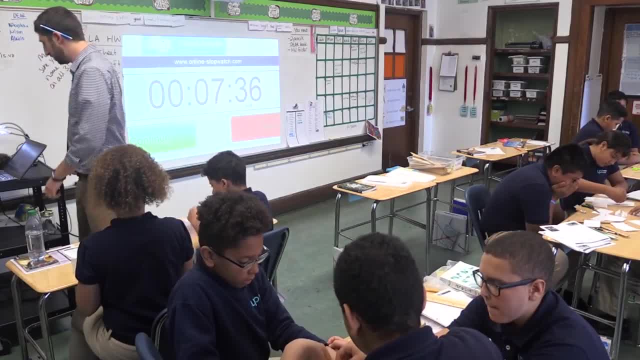 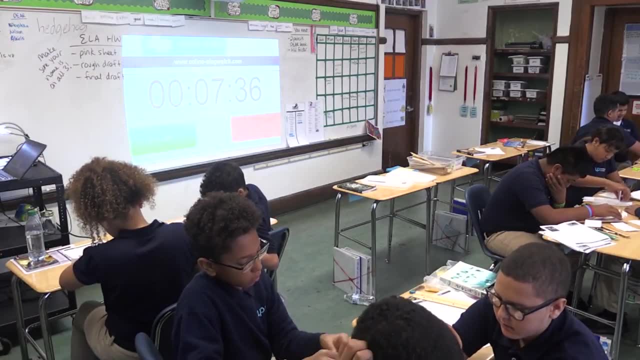 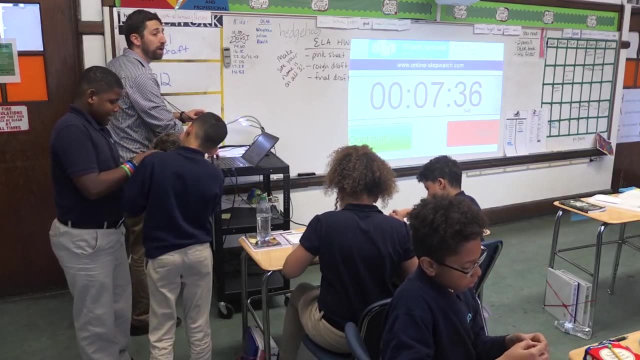 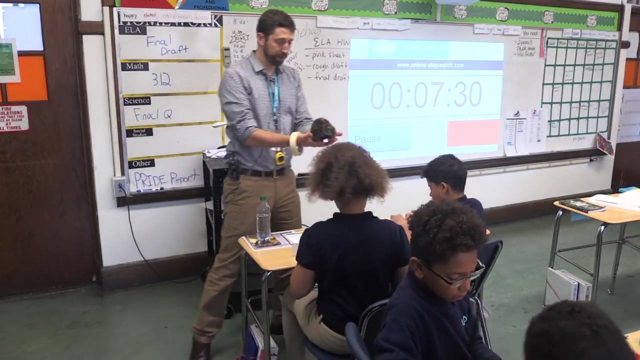 Keep going. Yes, sir, Can we touch him? You may? I'll just chase this part, José. English Timer is going back on. Thank you, Of course, Remember. would you like to feel the hedgehog? Would you like to feel the hedgehog? 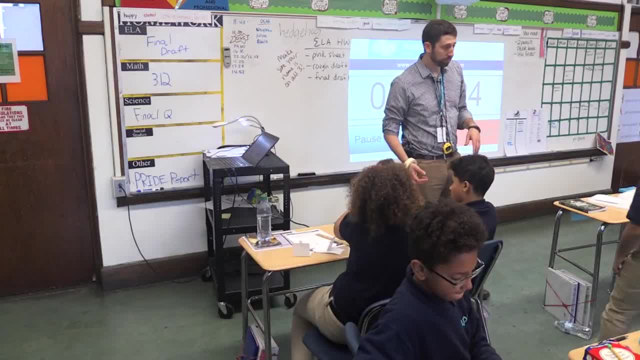 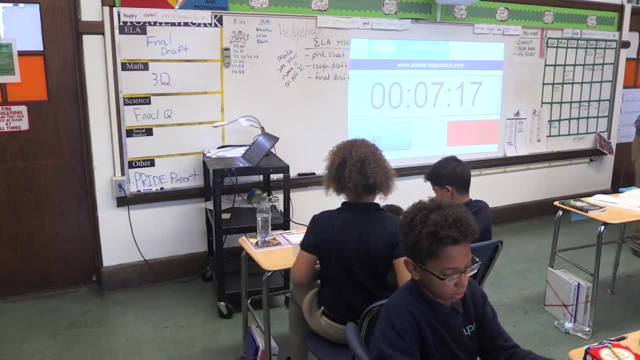 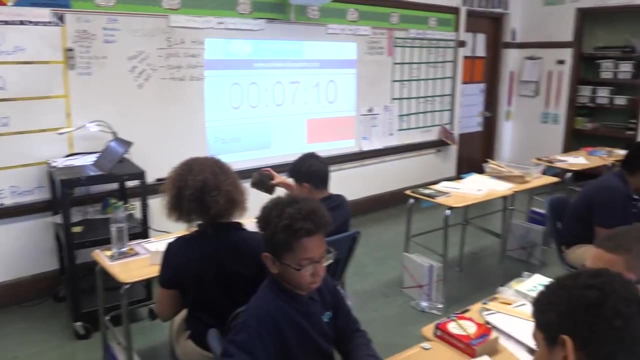 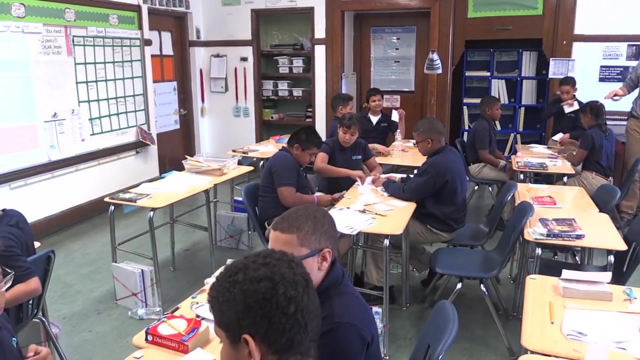 It's pretty light. You know he's José, remember? if you failed the challenge, that's fine, But be respectful, be calm, Do you understand? It's like we talked about on Friday. What do you do when it gets hard? 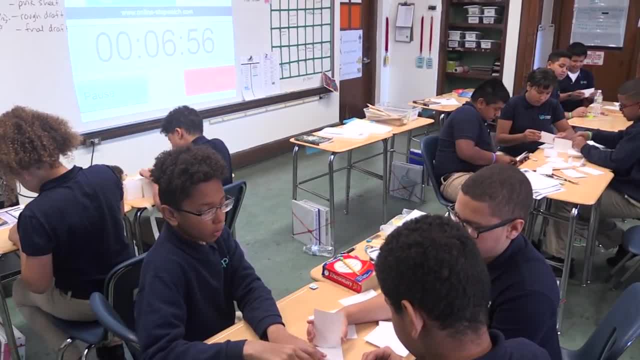 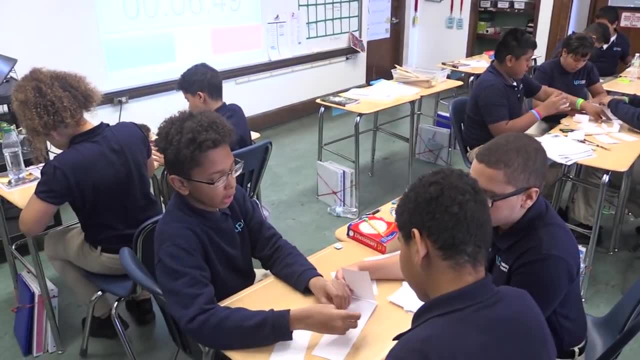 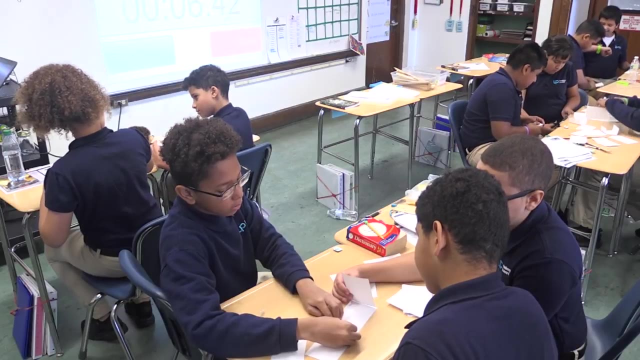 So what is our height at? How close are we to the goal? 13. 13. So you are this close. Okay, let's do it. Is your base strong enough to support the top? Maybe, Mr Warren, take a little bit of advantage, because there's people that have already started. 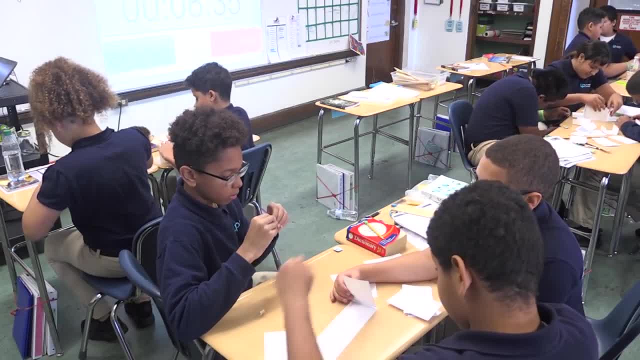 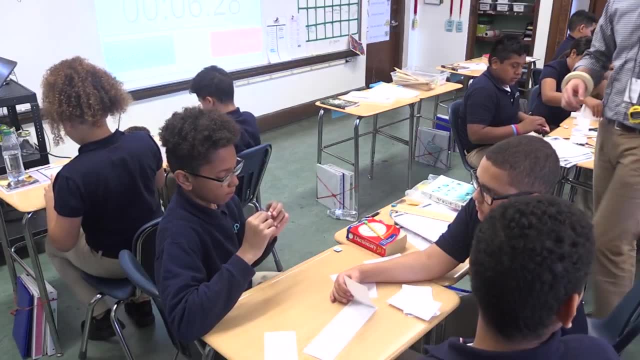 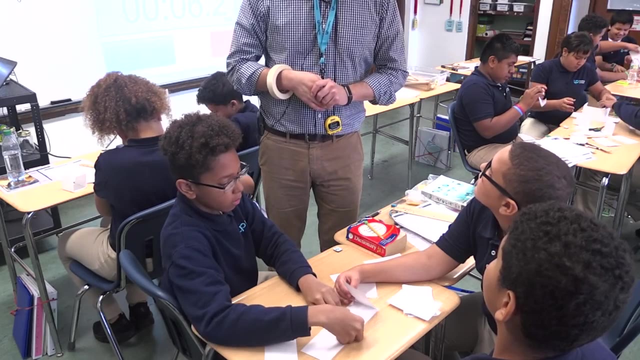 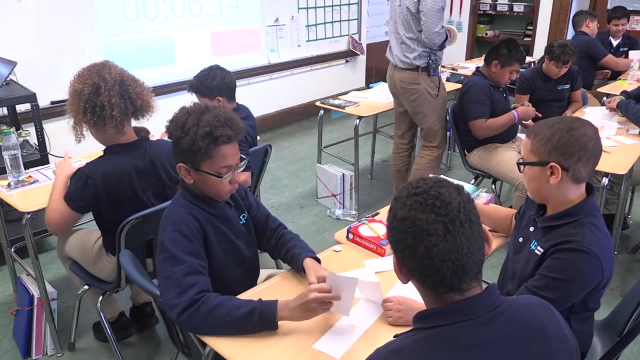 but they're not going to be able to do it. You keep doing what you're doing, then, Now, careful. Is this stable enough? How do we make it more stable? Now, gentlemen, you've got six minutes. What is our height right now? 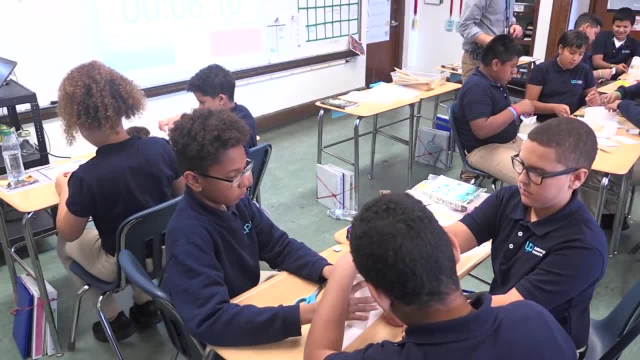 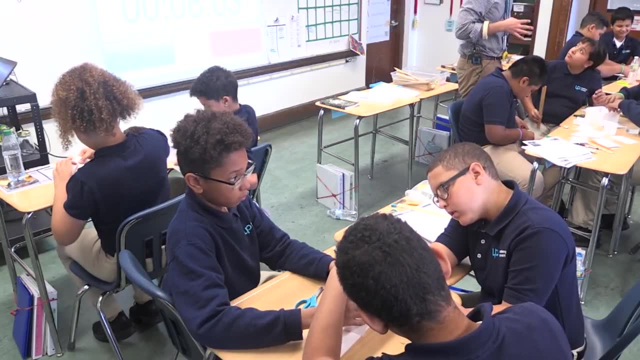 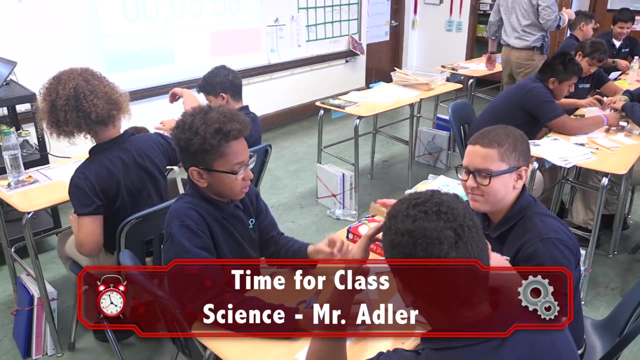 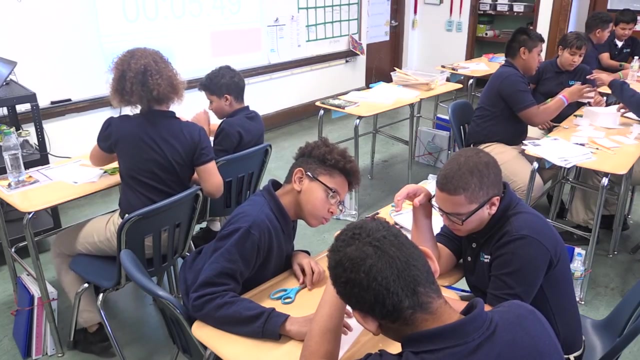 This looks interesting. What is the height of it right now? Seven, Seven, Good, Now make sure that you're dividing up responsibilities to get to 15 in time. So one, I'm not miss. Two, freeze, track me. 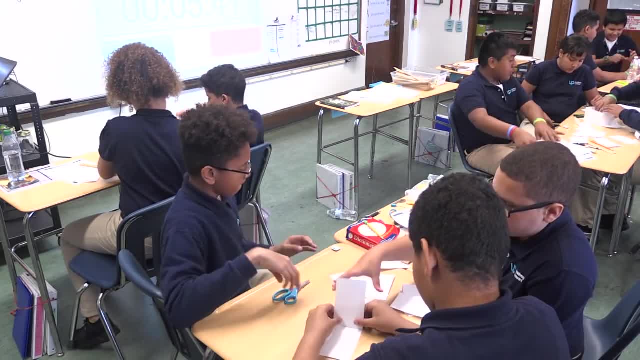 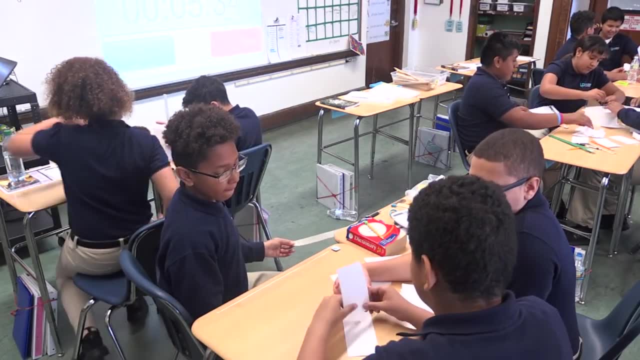 Communicate What could she be doing, Because you need to build more parts And you could have people building different parts right now. I asked her if she can help us. Well, right, But helping isn't helpful if she doesn't know what you're doing. 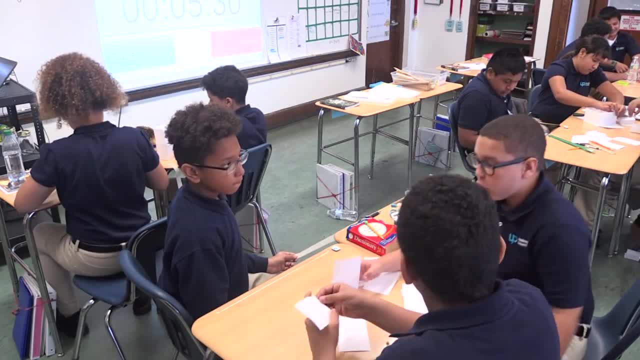 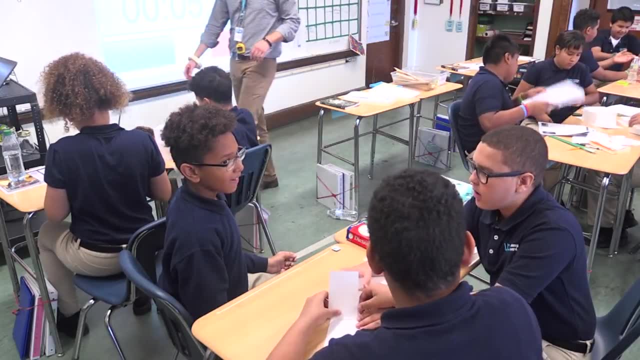 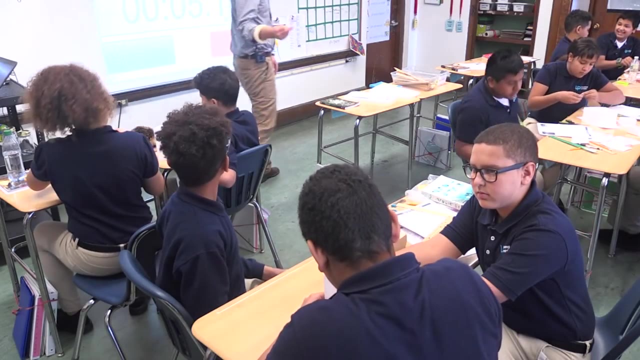 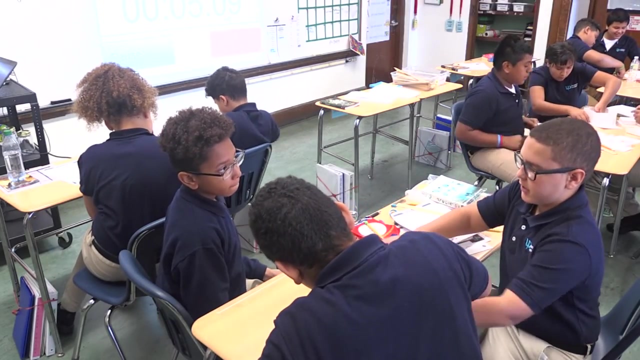 You need to communicate better than help me. Okay, So you're going to make that box. So you're making an additional box. All right, Do you like it? Yeah, Yeah, Yeah, Yep, Yeah. I think this amount of time now, if you want it, should be more or less more than. 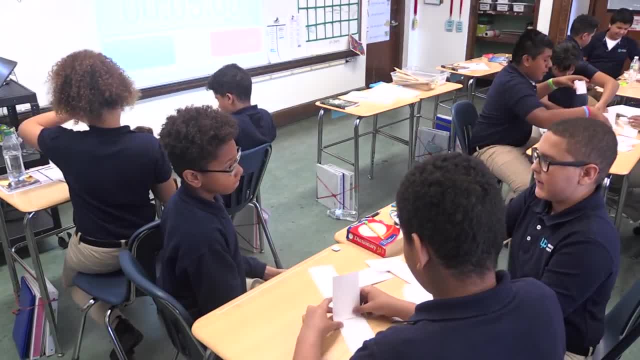 your actual time. All right, Can you get the line Secret 3 to be put on? most of this Mm-hmm. Have you had that? I'm sorry. This amount of time Makes sense to me. Just make sure you're within the time and you've reached 15.. 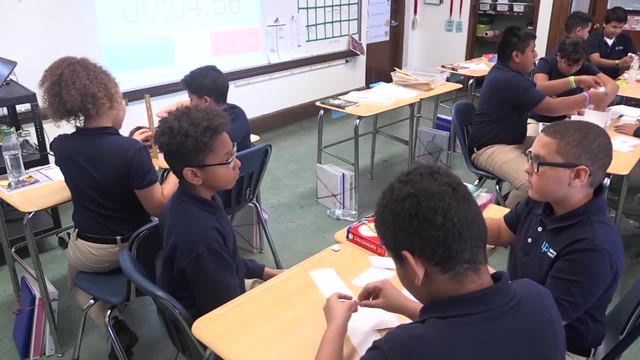 Okay, Um-huh, So now that you hold them on like that, I'm sorry. There's another way, so it could, like Makes sense to me. Just make sure you're within the time and you'd reach 15.. 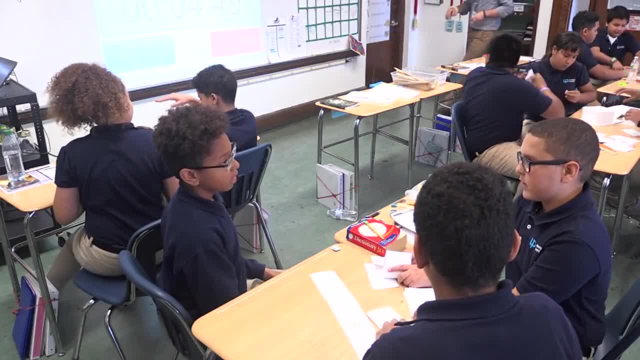 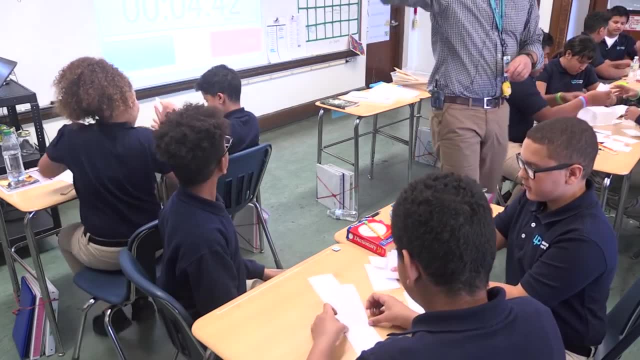 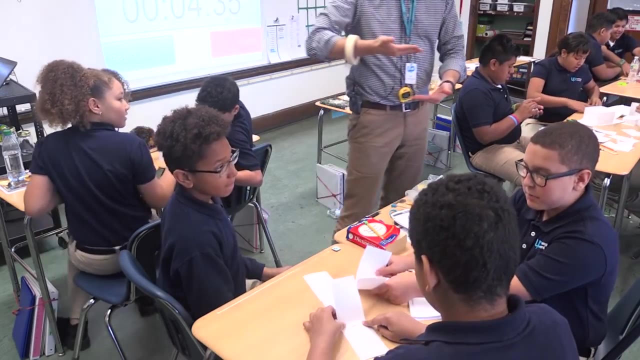 Yeah, No, Now it looks like everyone is getting involved. Excuse me wait. Gentlemen, make sure to keep track of time. You have five minutes. five minute warning. five minute warning, gentlemen. our Brit, our tower is currently flat. we need to make it go up in the next five minutes. now to two boxes: get. 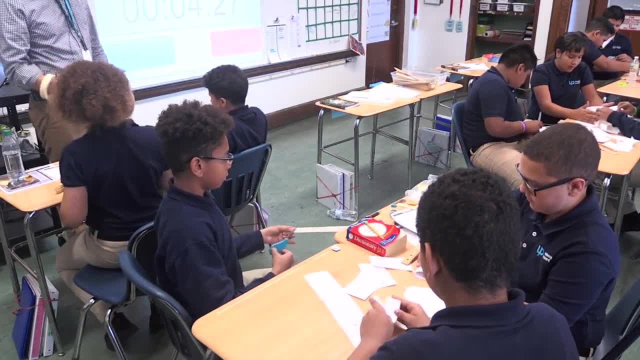 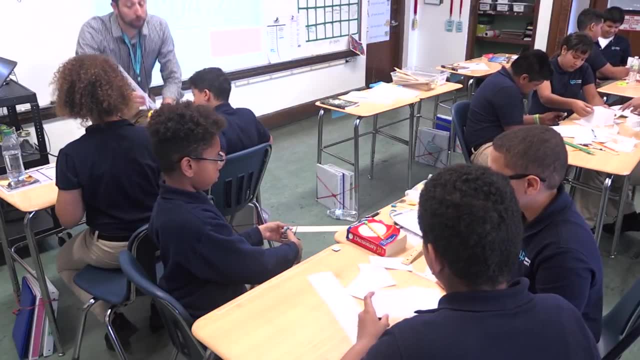 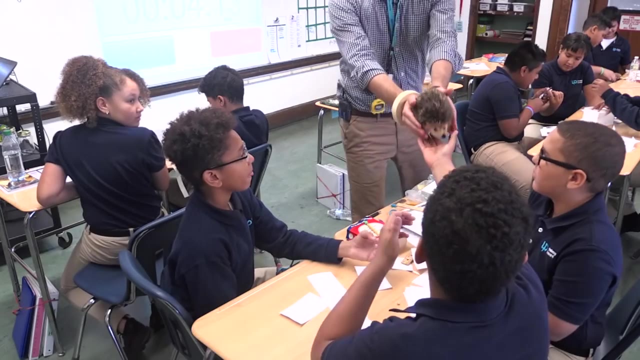 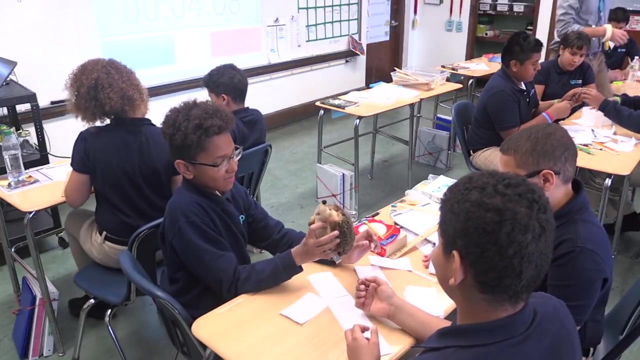 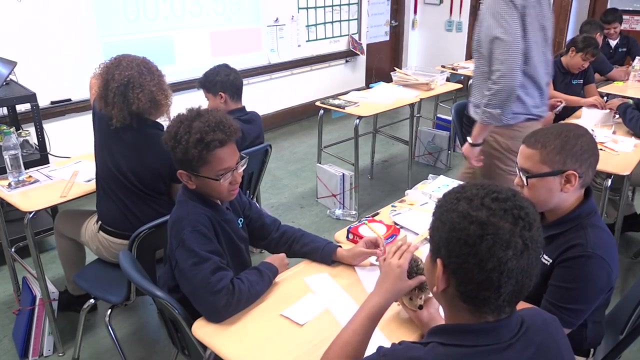 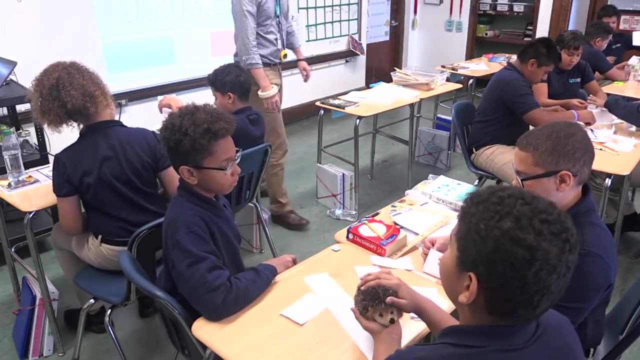 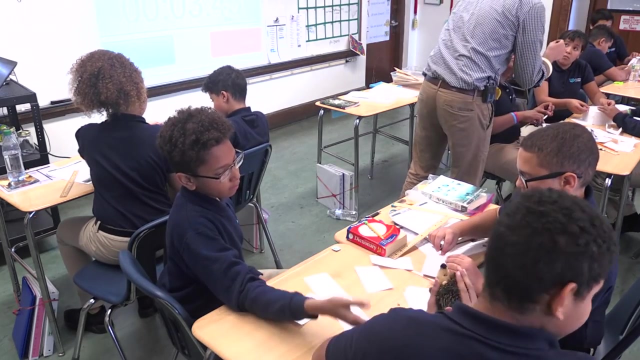 you there, or do you need to go higher? well, let's check it out. oh, you are so close. keep it up. do you need to feel Glen the Hedgehog? okay, okay, all right now, keep going. that looks extremely stable. does it meet the rules yet? well, does it meet the? 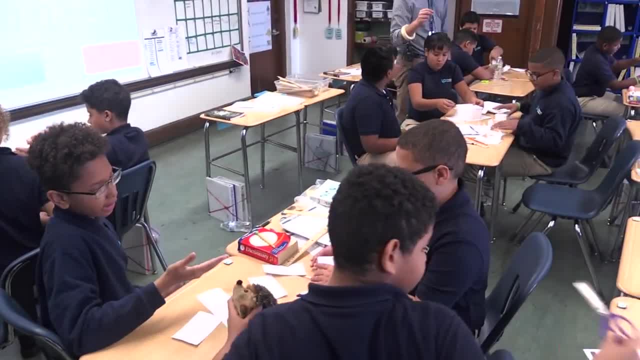 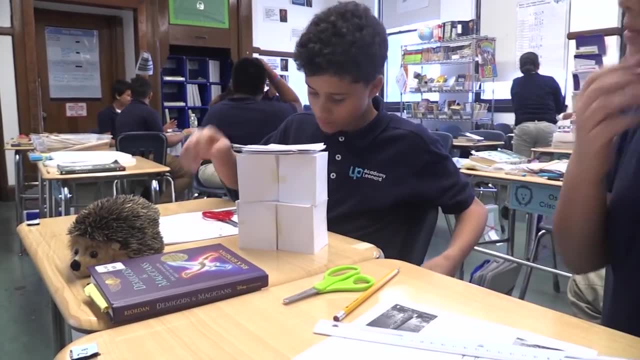 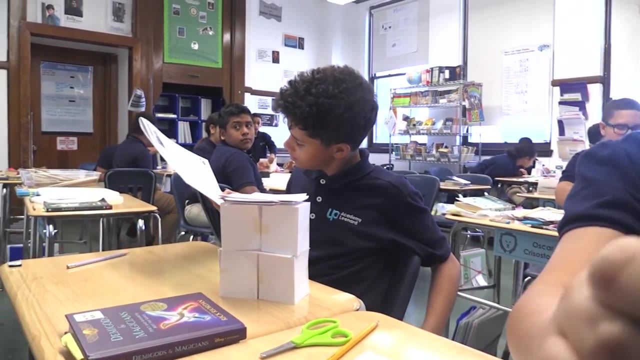 rules of the challenge. yet what do you need to do in the next four minutes? let's do it, oh, but careful. can you test early? can you test early? you cannot test early. so is it tall enough? check page two sixteen. so is it tall enough? check page two sixteen. 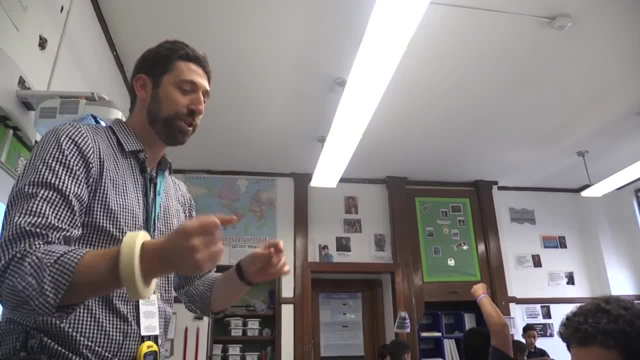 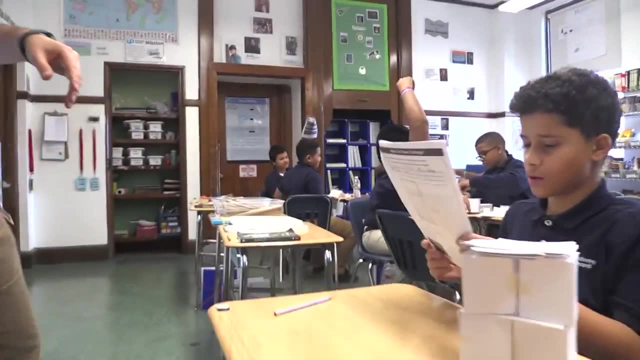 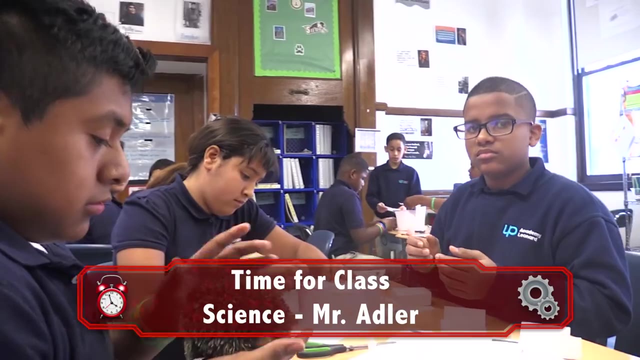 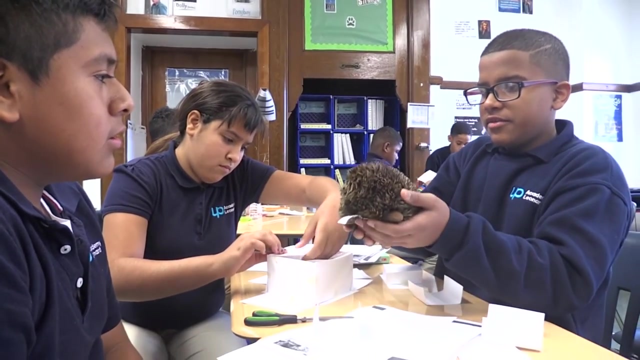 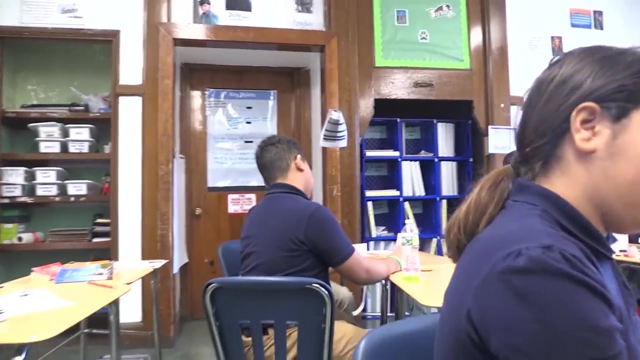 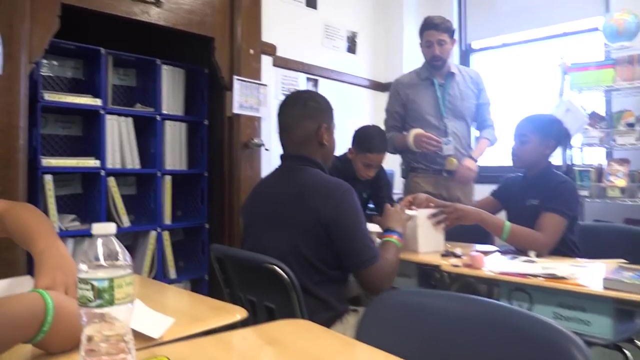 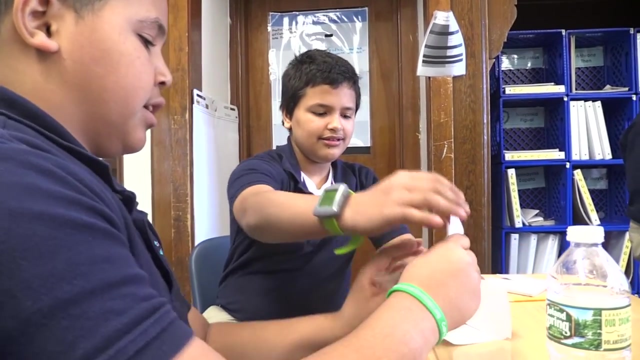 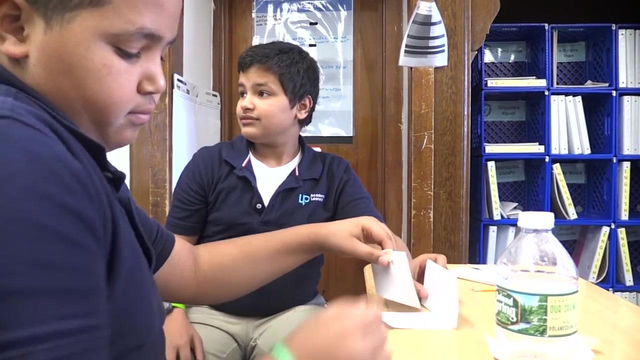 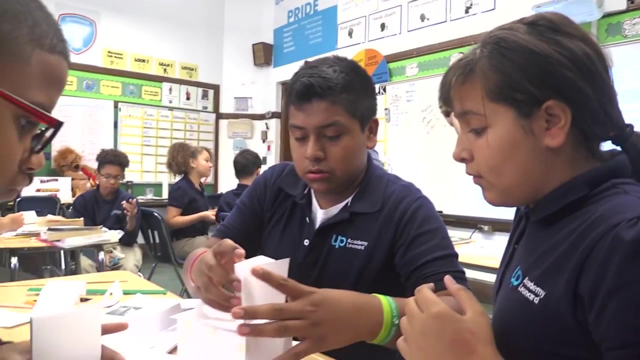 so is it tall enough? check page two: sixteen. what? check page two, see if there are any pieces that you have forgotten in this challenge. yes, you may, but you cannot test with it early. seems to stand up to win. I like it now. I like that. we're not supposed to test early. 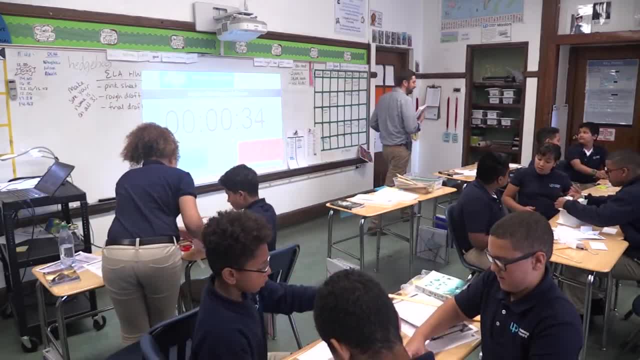 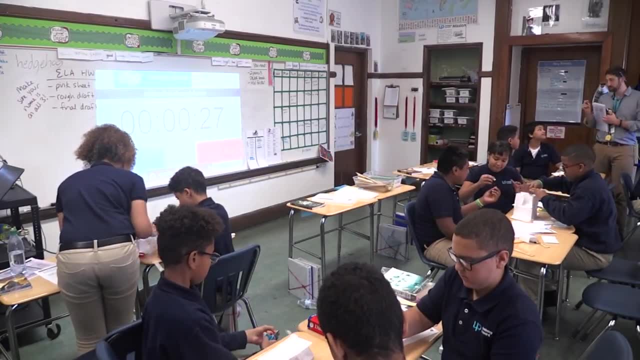 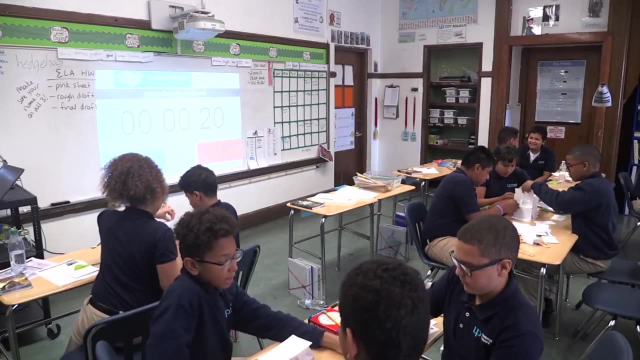 30 seconds, Carlos, okay, did we struggle with the challenge, but did you respect each other? did you share materials? you can still learn in four hours. so it's okay, calm down. is this stable enough down here? so it's okay, calm down. is this stable enough down here? 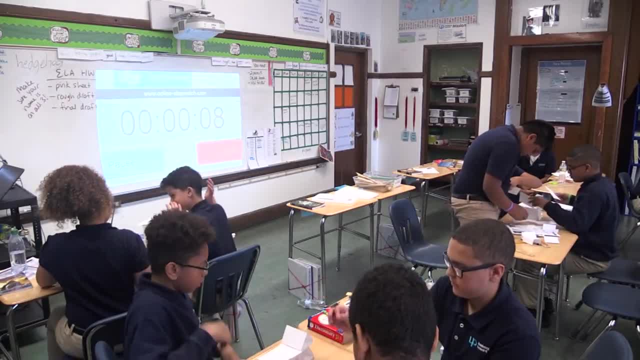 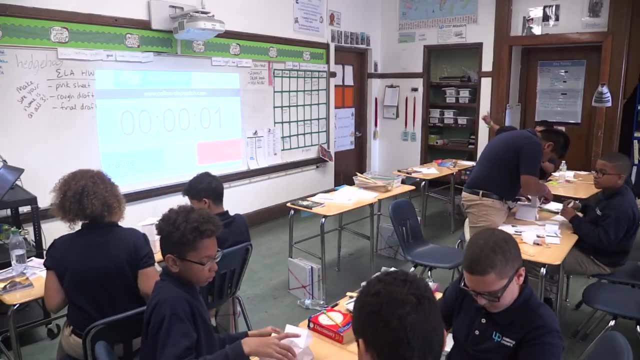 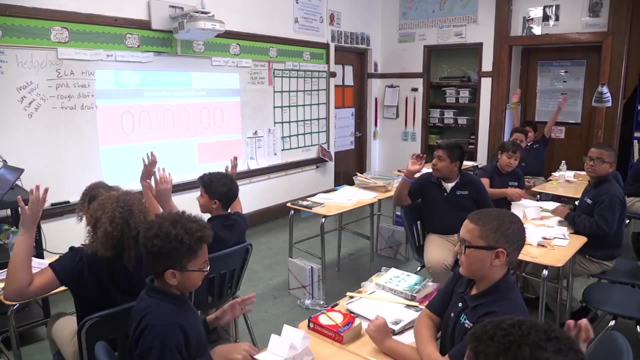 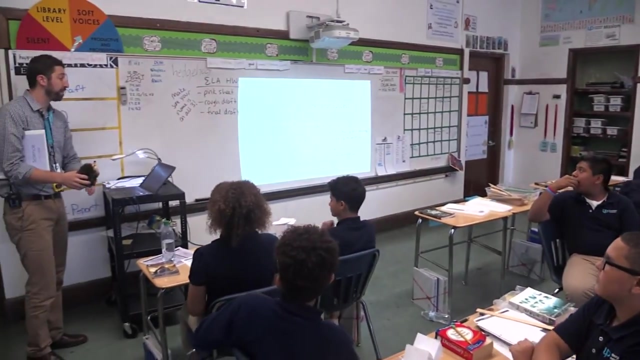 Hands free, track me in 5,, 4,, 3,, 2, 1.. Track the board. If you touch your design, you have failed today's challenge. Remember this was the 4 out of 4.. Thumb up or down. 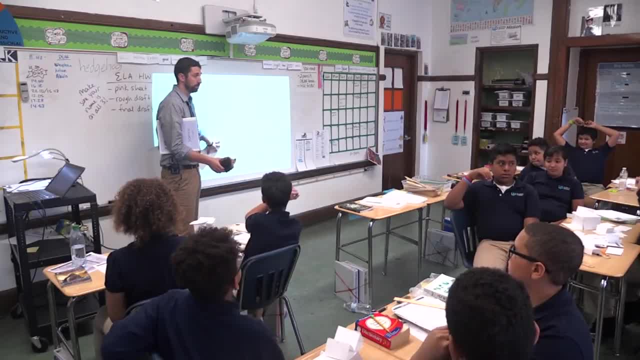 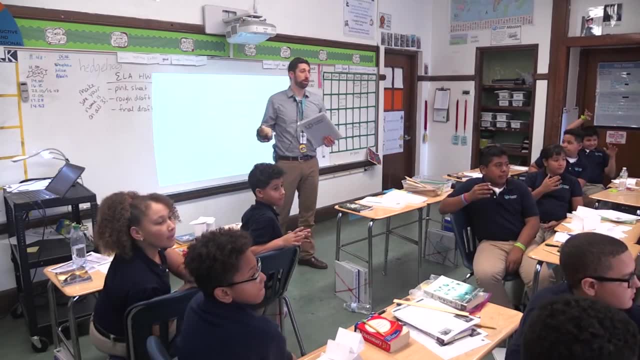 Do you fail today's class? if your tower doesn't work, Hands down, track Nilsen. shining Nilsen does it say you'll get a 0 if your tower doesn't work? Track me. And, in fact, which of the pride values do you see most often on this slide today? 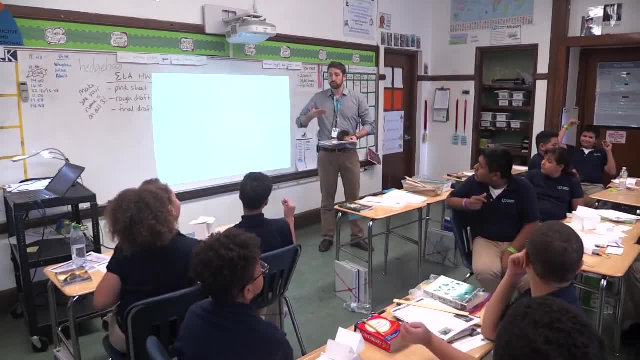 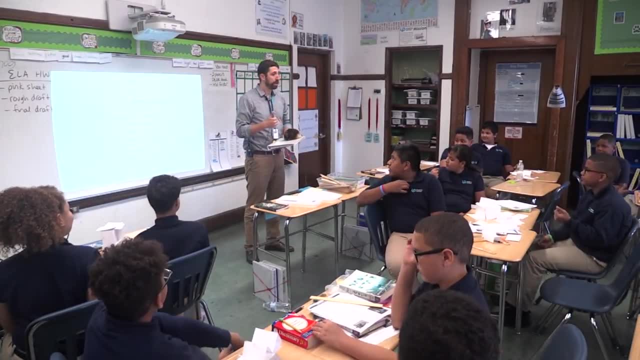 Hands down. track, Jose Mateo, So track me. If I can see you shining for other teams, snapping for them, you're earning yourself points today. If I hear anything disrespectful, you're losing yourself points today. Capisce, I'm going to start over here, move over. 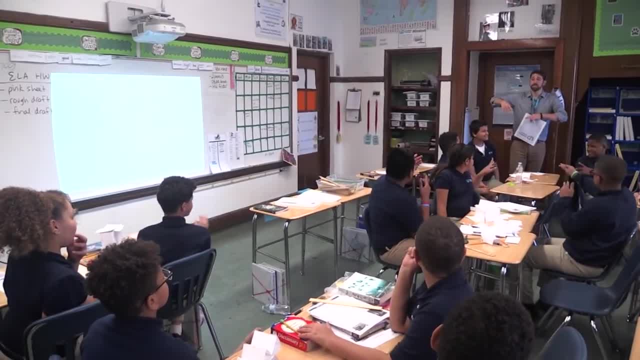 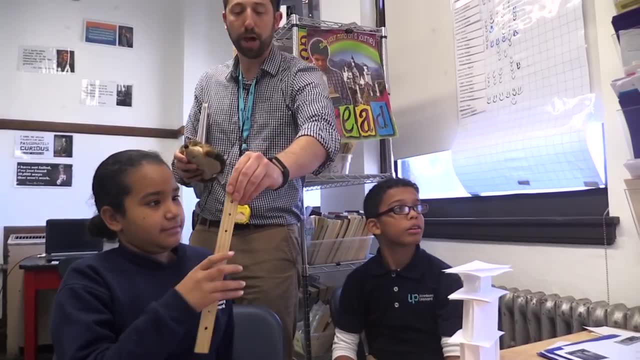 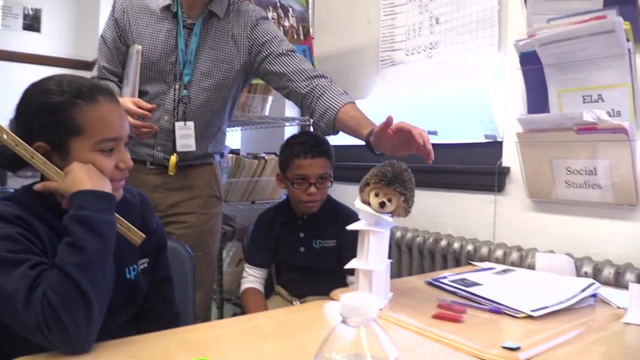 My first group was not able to build a tower, so shine on them. Let's see if they can do better. next challenge: 21 centimeters tall. Hold that please. Glenn needs to stay on for 10 seconds. Glenn could not stay on. 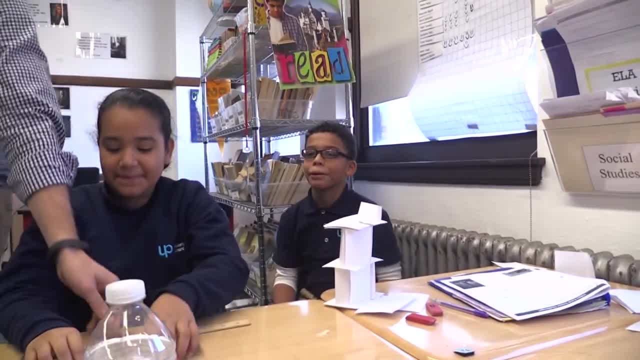 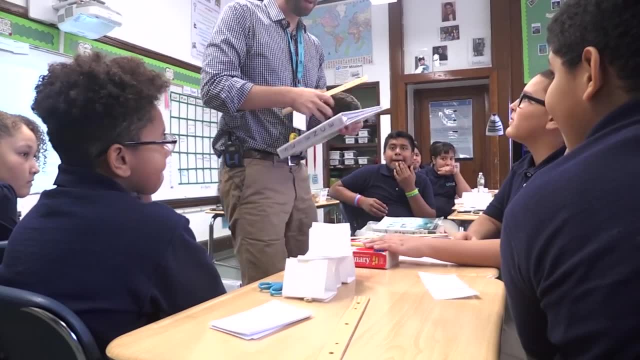 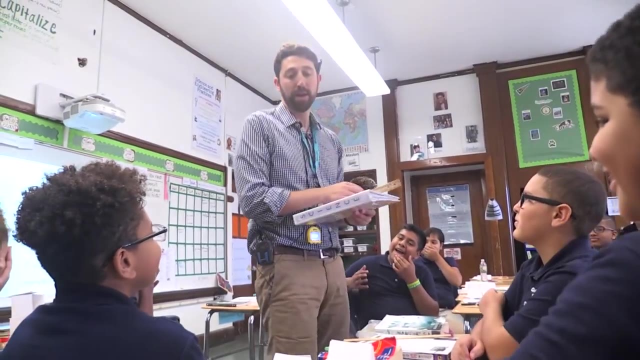 Snap for this group. They met the 15. Centimeter requirement. This group tracking over here, It does not. it is 12 centimeters. Will Glenn be able to stand? Glenn cannot stand on top. Snap it up for this group, though, for a very good effort. 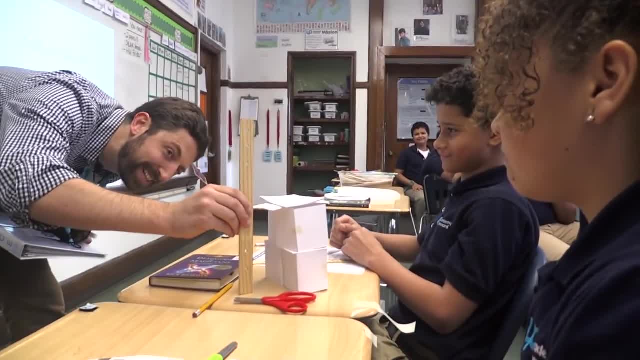 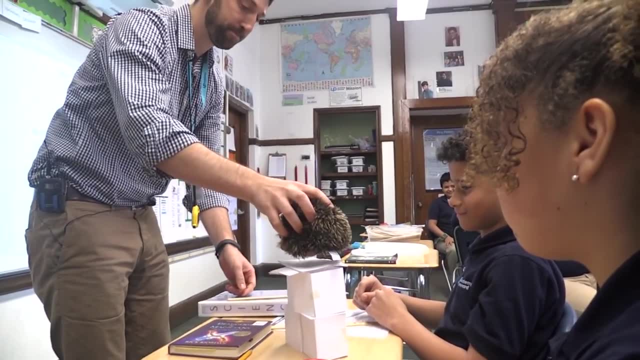 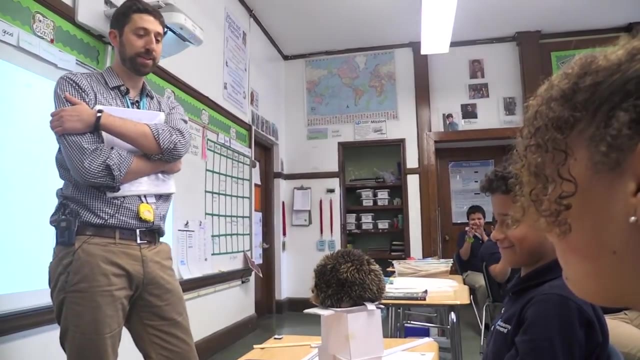 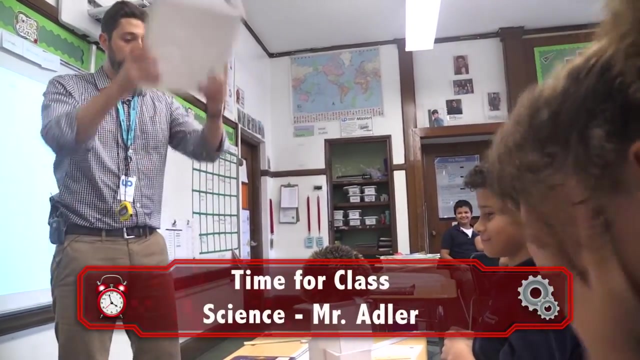 This tower is exactly 15.2 centimeters tall. Will Glenn stay on 1,, 2,, 3,, 4,, 5,, 6,, 7,, 8,, 9, 10.. Last requirement three: second gust of wind. 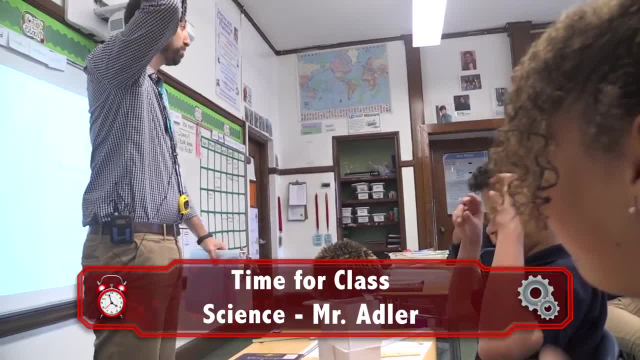 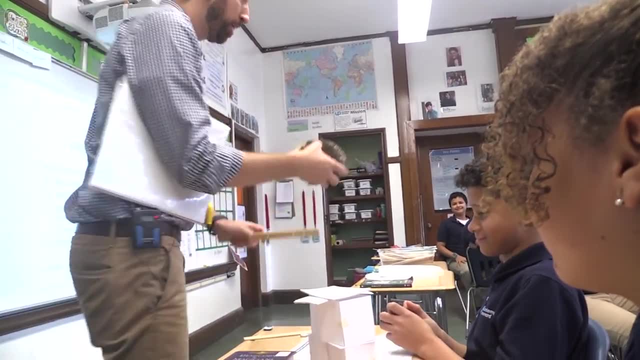 Snap it up for the first group to meet all three parts of the challenge. 2 claps for them on 2.. 1, 2.. All right, Moving on to this group. This group did not meet the challenge. The first group did not meet the challenge.